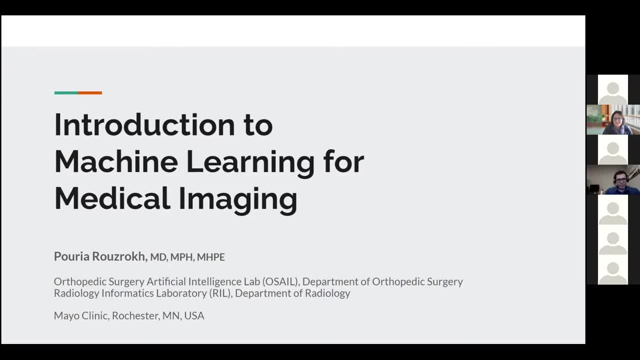 the first lecture in this workshop and I'm glad that he's back again to give our third lecture. So, Poria, take it away. Sure, Thank you and hello everybody. Good afternoon. I'm happy that I'm with you today for my second workshop and your third workshop in this series in general, and I would 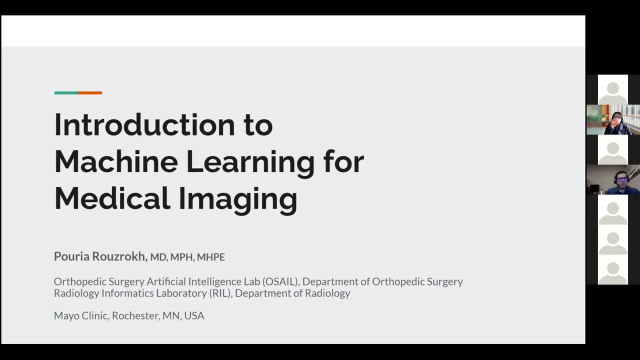 like to seek permission from my mentors, Dr Westendorf, Dr Meredith Tremers and Dr Erickson, who are all available at this call, to start this presentation. I hope that we can have a good talk together. So I am going to talk about applications of machine learning in medical 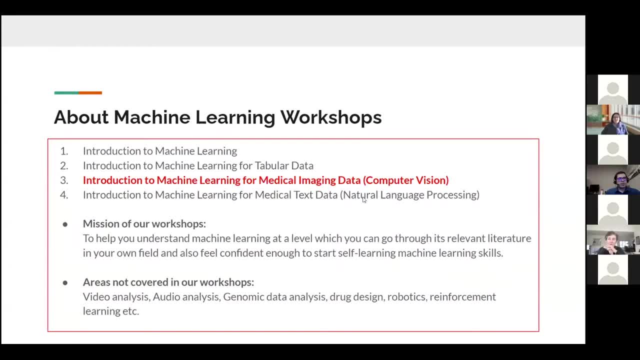 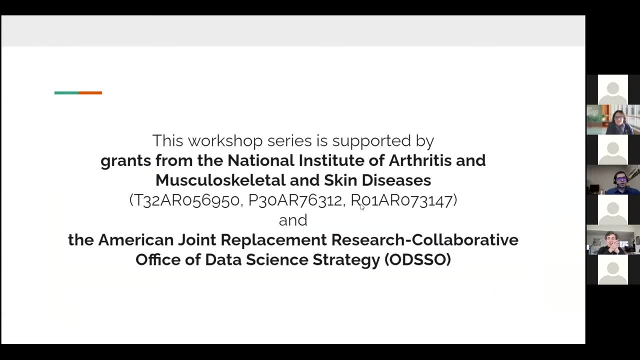 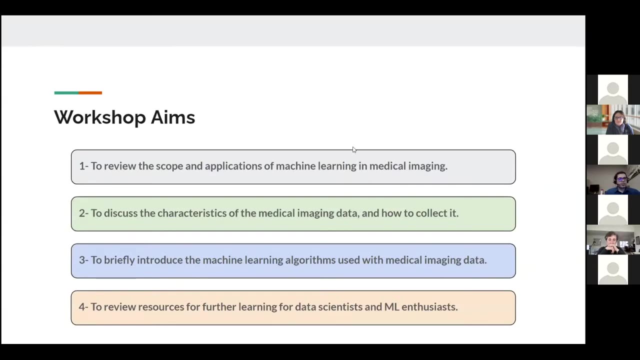 imaging. This sometimes is also called computer vision in medicine, but, as I will tell you a few minutes later, this is something that some people also want to call something else. So I'm going to briefly review the different aims that we are going to talk about today. 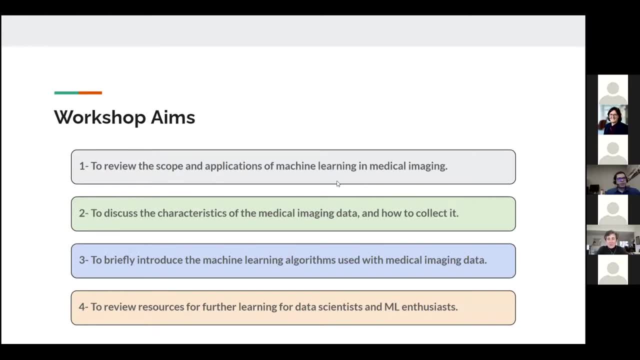 I'm going to start talking about the scope and applications of machine learning in medical imaging in general. This will give you, hopefully, a big picture of what machine learning can do in medical imaging, and then we will talk about medical imaging data itself and how to collect that, what properties of that data is and things like that and hopefully, 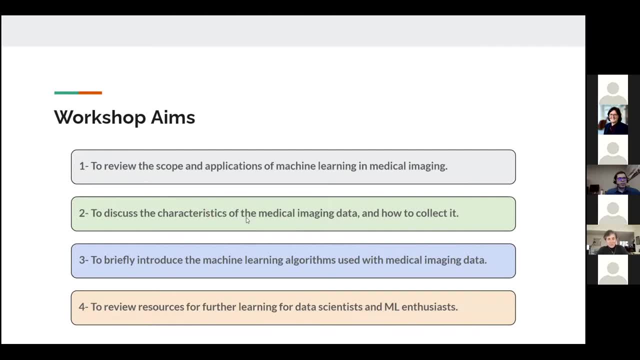 these first two parts will actually give you enough information to understand what is happening in the world of AI and ML when we apply that to medical imaging. And then in the third part- this is where things get a little bit more technical- I would like to talk about the most fundamental concept of computer vision and machine learning. 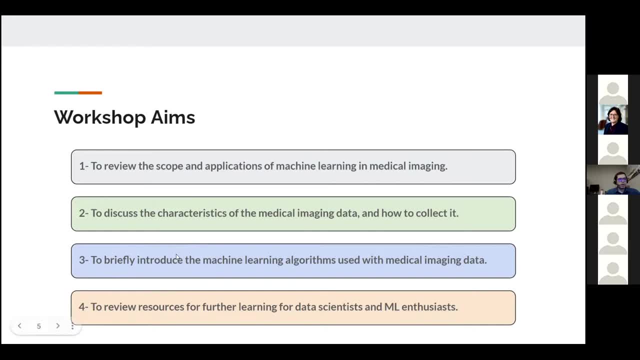 in medical imaging and that is the concept of convolutions and convolutional neural network. We will have a lot of animations and GIF images here, So this is the most technical part of the talk, but I wanted to put that after these two first general parts, so that we make sure that we 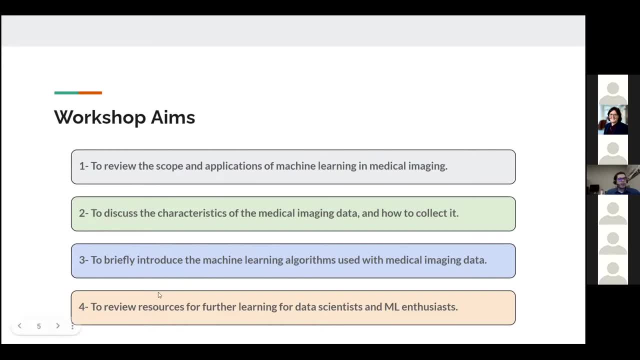 cover the basics first, And then, finally, we will go through a couple of slides and review resources for further learning for data scientists or those who might not want to do the programming but are only interested in it. So this is actually our general plan for today. I would try to go through these first two parts. 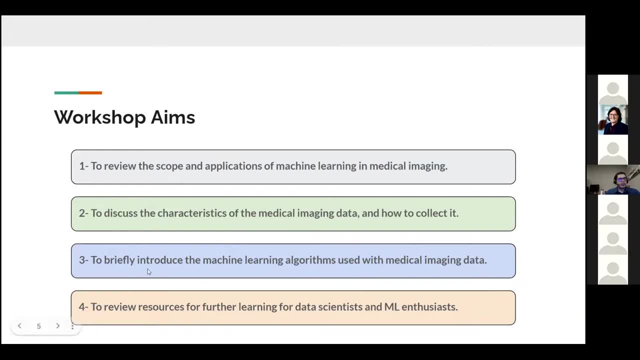 a little bit faster because I want to spend enough time on the third aim, but please feel free to interrupt me wherever you want it. Feel free to ask questions. I would also make sure to have an eye on the chat box here, And then I will also pause at the end of each of these aims to make. 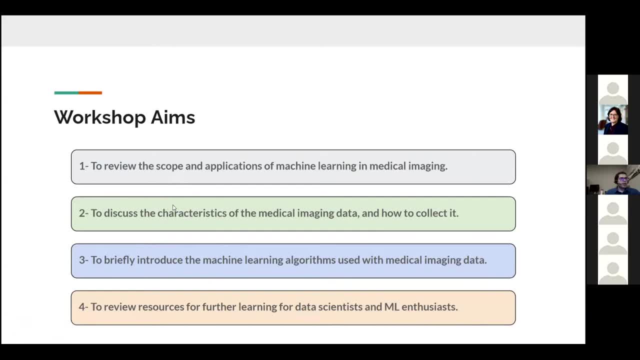 sure that we are all on the same page and following each other. So let's start and talk about the scope and applications first, And then I will also pause at the end of each of these aims to make sure that we are all on the same page and following each other. So let's start and talk about the scope. 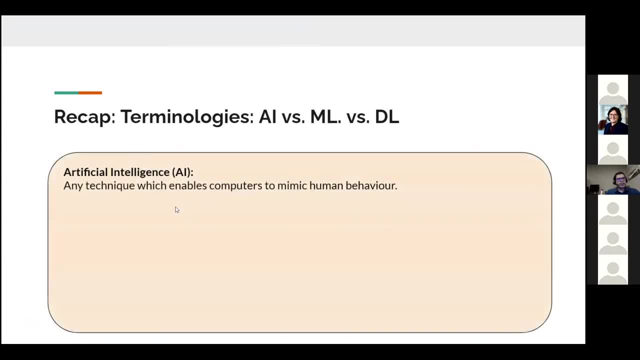 and applications first. Now I would like to start with one recap slide, And this presentation is going to have about six or seven recap slides from my own presentation that I had in the first workshop of this series and also Alex's presentation. So this is only to remind you of the 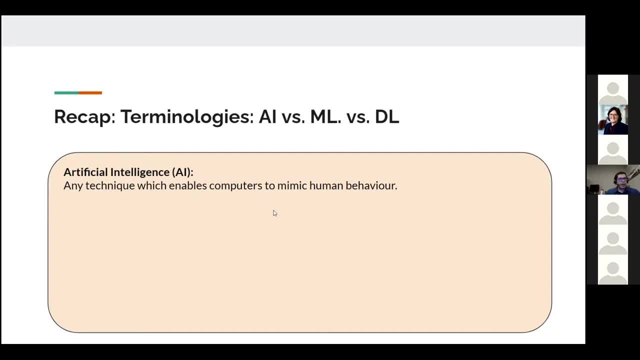 concepts, the basic concepts that we went through, because ML has a lot in common, regardless of what specific application you're looking at- I mean, if you're looking at computer vision or natural language processing. some of the basic concepts are going to be in the first workshop of. 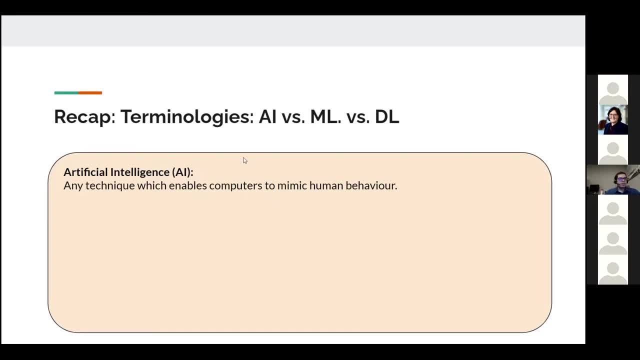 are going to be the same. so it's worth reminding ourselves of some of these basic concepts first. so, if you remember, in our first workshop we talked about what ai, ml and deep learning mean, right? so ai was any technique which enabled us- or enabled computers, better to say, to mimic human. 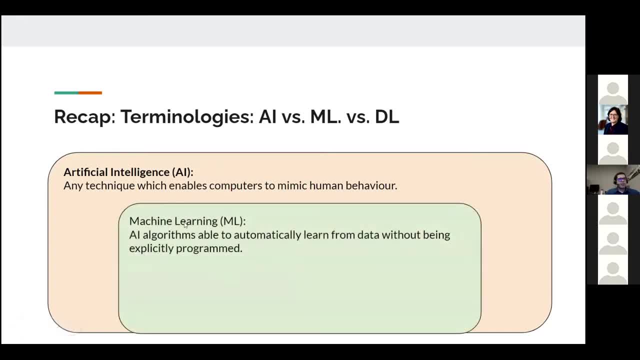 behavior, and then machine learning was a subset of ai, or better to say, some kind of ai algorithms that were able to automatically learn from data without needing us to explicitly telling them what to do or programming them what to do. so these are the kind of applications that are now. they. 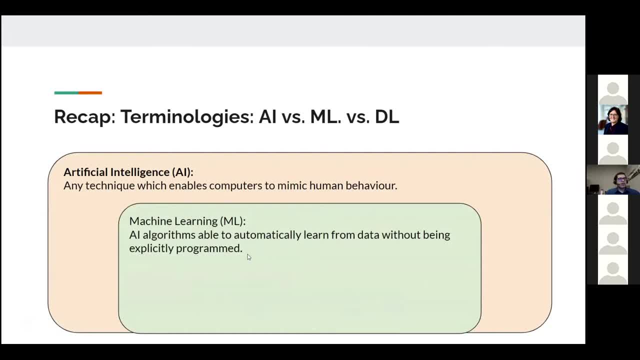 uh, considered almost a state-of-the-art application of ai. and then in machine learning we had a separate, or better to say, a subset that was called deep learning, and deep learning denoted those kind of machine learning algorithms which could effectively learn from big data using artificial neural network. and if you remember, we talked about neural networks. what? 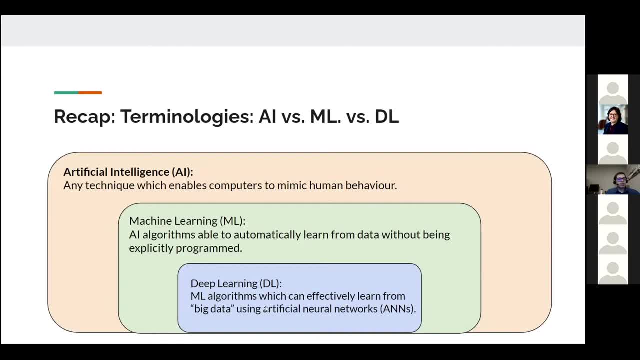 they mean the different architectures they had, and i'm going to quickly review those third part of this presentation as well. but the most important point was that you know neural networks make us capable of applying machine learning to big data, to very, very big data sets, and you know this could be big imaging data sets or text data sets or tabular data sets. 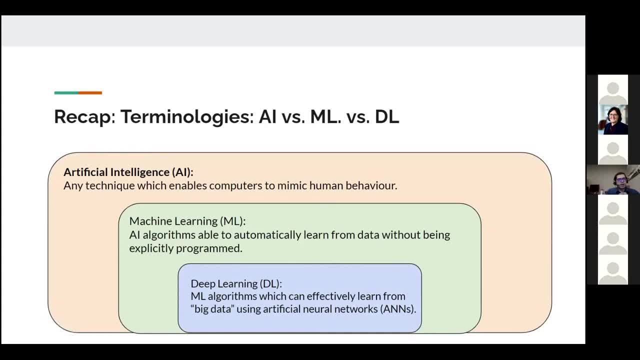 whatever. so deep learning and neural networks are. you know most of the times what people tend to use or prefer to use whenever they are applying machine learning. of course, the most important exception is actually the tabular data, where conventional machine learning is working pretty, pretty good in many instances, as alex talked in our last workshop, but for medical imaging that we are. 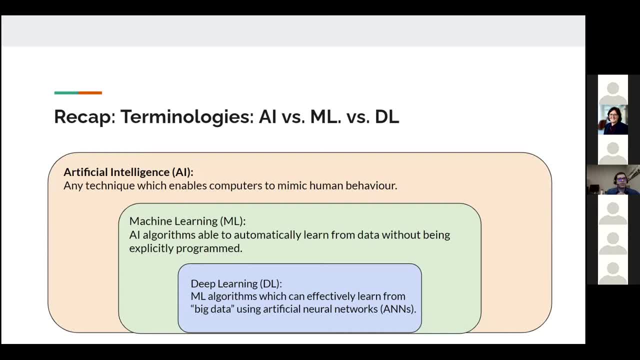 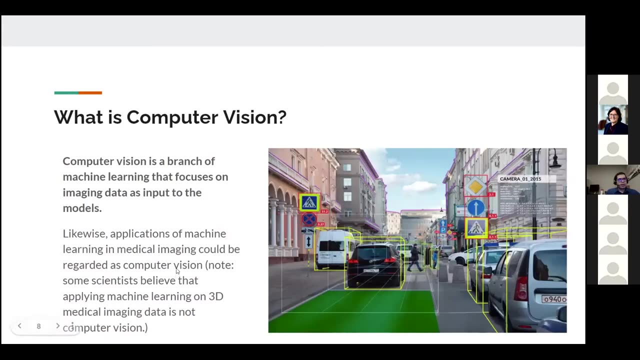 going to review today. deep learning is almost always the state-of-the-art technique that we use, and we sometimes try to amend that using conventional machine learning as well. so that was what we talked about, and you do remember that conventional machine learning was a subset of machine learning that did not include deep learning. now let's talk about computer vision, so computer 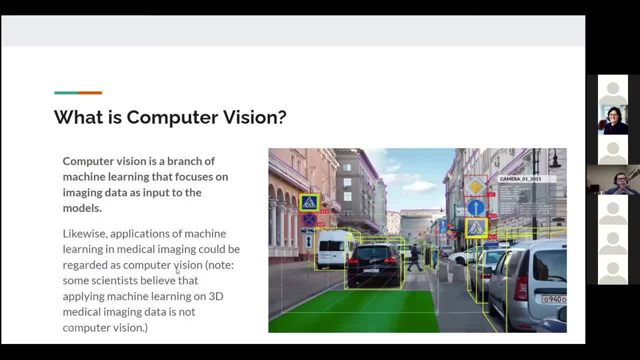 vision is a branch of machine learning that focuses on imaging data as input to the model, so this is a very specific to medical right. so whoever who works in ai and machine learning fields have probably heard about computer vision. so computer vision means whenever you are working on medic, on. 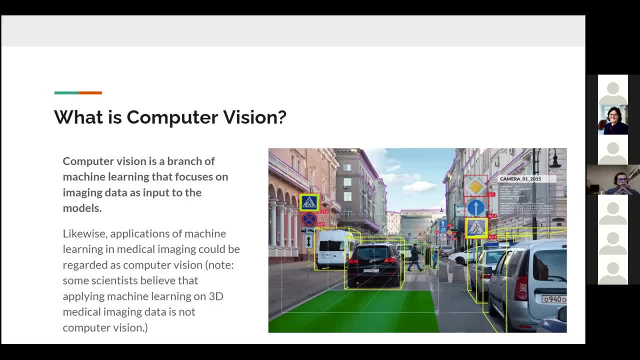 you know any type of imaging data as your input. now, likewise, application of machine learning, medical imaging could also be regarded as computer vision, with one important side note, and that side note is that you know, sometimes some people believe that you know- applying machine learning on 3d medical imaging data, which you know we still 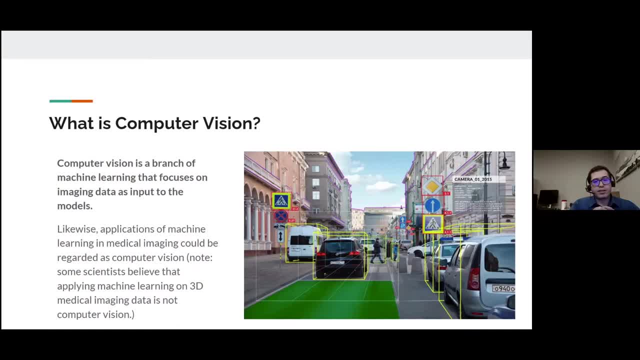 have a lot of people who believe that, you know, applying machine learning on 3d medical imaging in our own medical world might not be regarded as computer vision, because computer vision, you know, most of the times, uh, in engineering world denotes applying machine learning to 2d data. natural images. 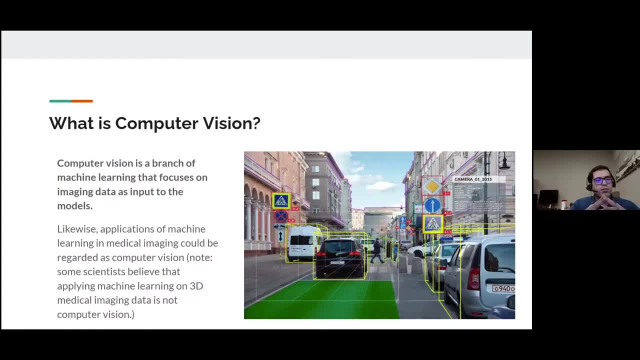 for example. right, so sometimes people have different terms for calling what we are. you know what we mean by saying medical imaging and machine learning, but for the sake of this workshop, i am going to keep using the term machine learning in medical imaging rather than computer vision to. 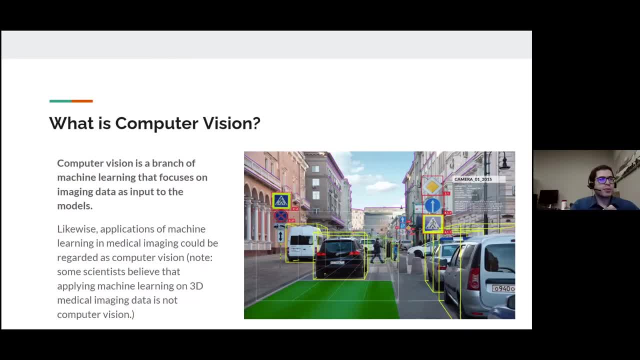 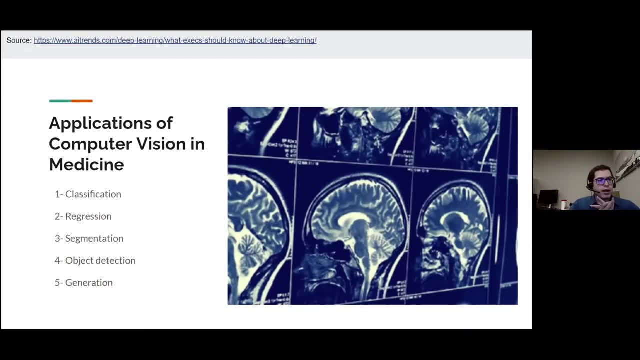 make sure that i'm also emphasizing the importance of computer vision in medicine. so i have put five different, five main applications here. definitely there could be more, but these are the five most common and i'm going to quickly introduce each, provide some examples to you and then you know, make sure that you understand what. 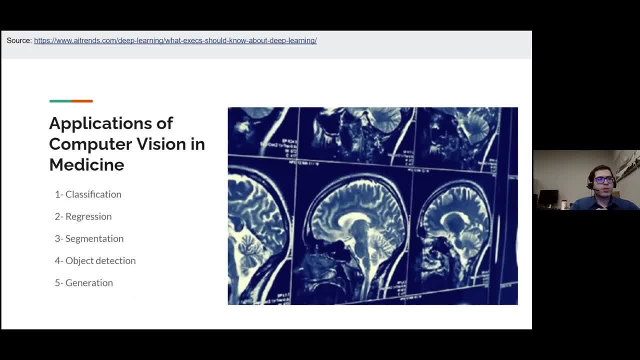 each of these applications mean and how this could be useful in real research or, you know, in real clinical applications. we will talk about classification, regression, segmentation, and then you know we're going to talk a little bit more about what we're going to talk about in the next few minutes, so let's get started. 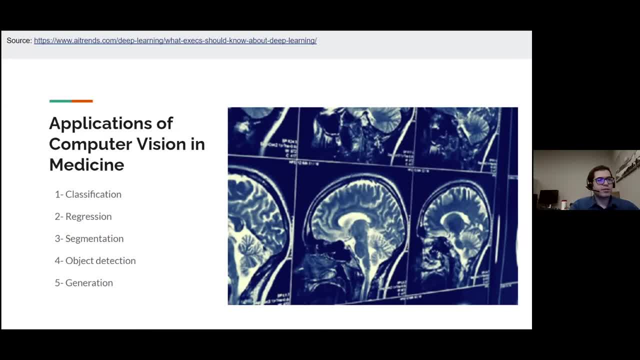 object detection and image generation. so let's start with classification first and then, as i said, at the end of these five, five slides, i would like to pause and make sure that everybody is following. so if you had any questions and if it was urgent, feel free to interrupt me. 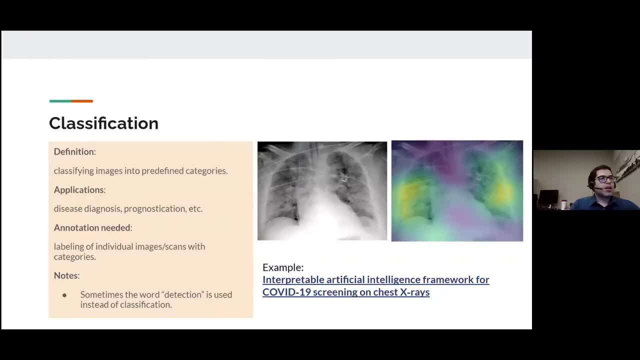 otherwise i will pause and ask you about your questions. so classification basically means that you are receiving, or your model is receiving, some images as inputs and you know you want the model to classify those images into predefined categories. so, for example, suppose that you have this input, x-ray chest, x-ray on the right, and you want your model to understand whether this chest 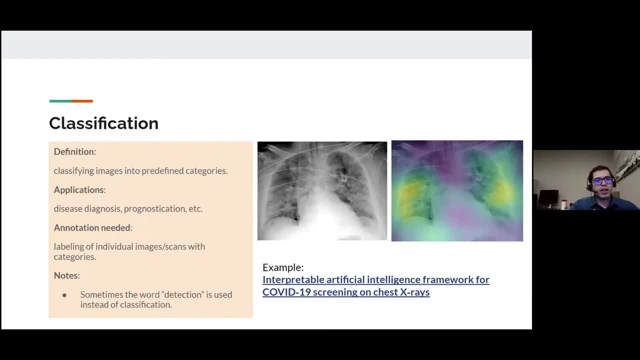 x-ray belongs to a patient suffering from covid19 or, you know, to a patient that is suffering from some other type of pneumonia or even some sort of other lung diseases. so this was actually something that a lot of papers talked about and went through when covid started. you know, actually covid helped. 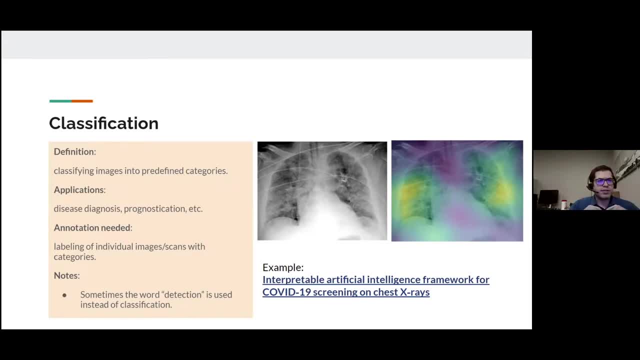 ai a lot specifically in medical imaging, because a lot of people are very enthusiastic to see and you know, you know to understand the diagnosis or the prognosis of covid19 patients, and i will talk about this a little bit more. there were also a lot of flaws there, when you know this. 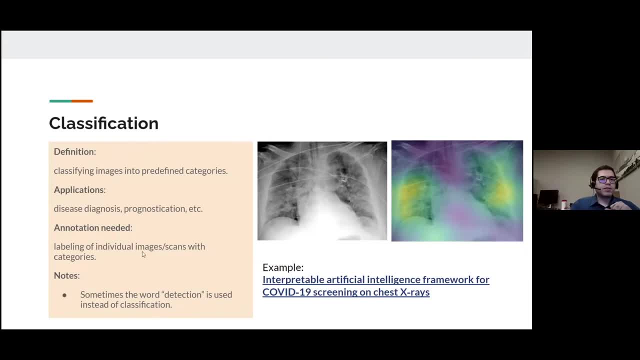 bunch of papers came out, but anyway, this is one of the papers that you know had been cited more than others. so you see that they had tried to understand whether this patient had covid19 or nine. uh, covid19 or not, using medical machine learning applied on medical imaging and you. 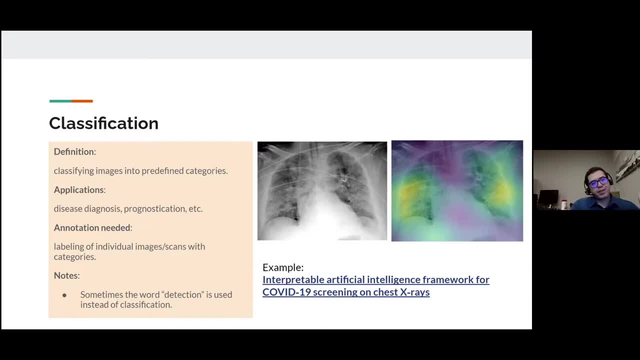 know this kind of uh, fancy image that you see on the right side. this colorful image is a tool that we have to show how these models are actually making their predictions or how how they are actually making their decisions. these are not quiet, accurate tools, but they give us some. 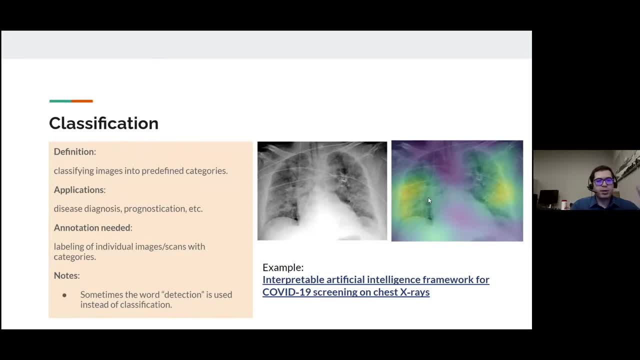 sense they give us some clues of what is happening behind the scenes. you remember probably from our previous workshops, that deep learning where most of the times criticized to be black boxes so that people will not understand how they are making their decisions, because, as i said, there were very, very big equations so nobody could really understand what is happening. 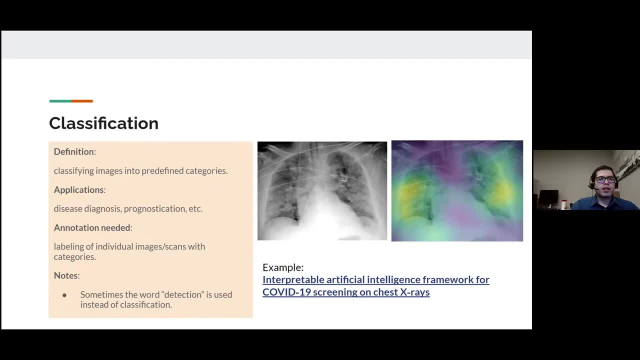 behind the scene, some efforts had been made to make those a little bit more explainable. one of these, uh, you know, famous efforts had been this kind of maps that we usually call them salience map or, you know, gradient activation maps, and these show that, for example, these, you know, highlighted 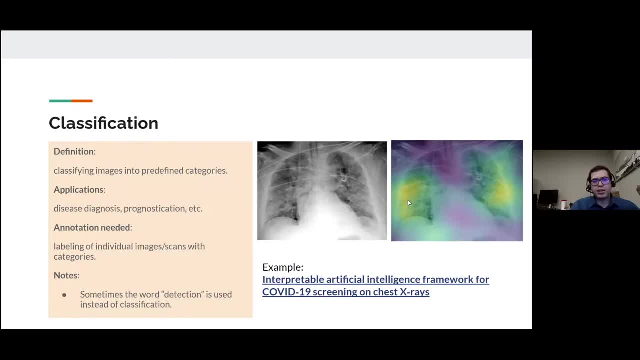 yellow parts of the image have been those areas that the model uh more emphasized on for making its predictions that this, for example, belongs to the covid19 patient. so if you saw this kind of images in you know machine learning classification kind of papers, this probably is trying to explain the model's behavior, but anyway, so what? what i mean? how do we use these? 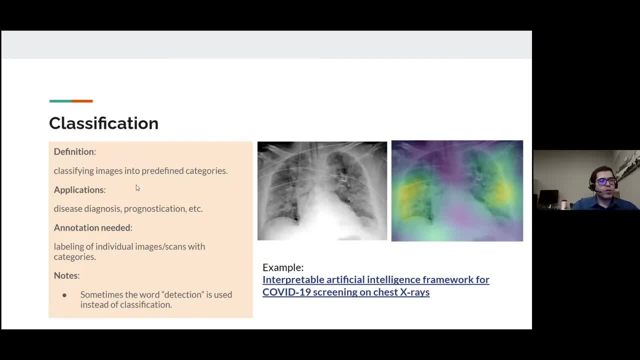 classification models. in medical world. we usually use them for, uh say, you know, we want to diagnose some diseases in patients or we want to- i mean, predict their prognosis. for example, we feed some sort of images, ct data, mri data of patients with you know? uh, you know, brain tumors. 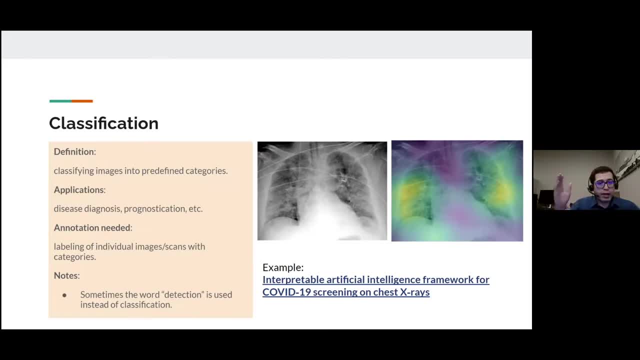 and we want to understand how long the patient is going to survive, or if they have good prognosis, you know, saying that they are going to survive after two or three years, or if they are going to, unfortunately, die earlier. so these are the kind of applications that we usually can. 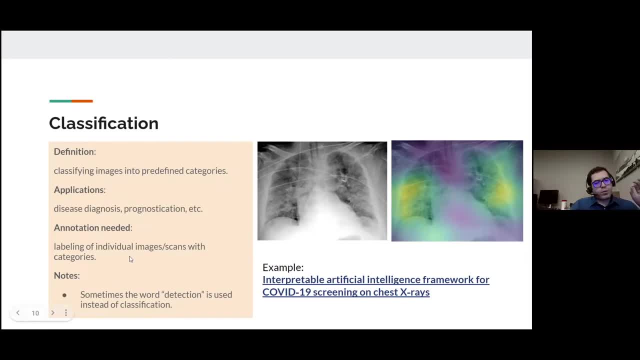 expect from classification models, and so you probably remember that whenever we talk about a machine learning project, specifically in those type of projects that were supervised machine learning, which basically means that the model is going to learn from labeled data- we needed to consider the time, effort and energy that we need to put into data annotation, right. so 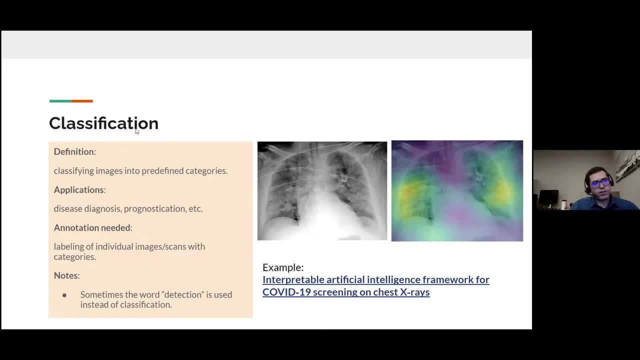 i'm going to specifically mention the annotation needed for each of these. now you know machine learning applications and medical imaging. so if you're going to develop a classifier or a machine learning classification model for medical data, you probably need to have your experts go through some of these images. you know they could be x-rays, they could be ct data, mr data, pets, sono. 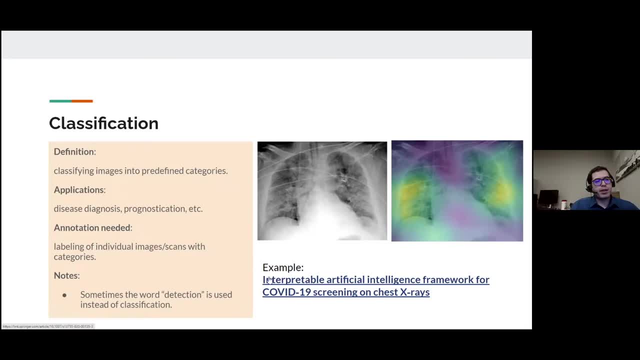 whatever modalities you are working on, and ask them to label individual images or scans with those categories that you're interested in. so, for example, people who actually authors or quarters who actually develop this paper. they had an expert team that went through, say, you know 2 000 x-rays, you know 10 000 x-rays. 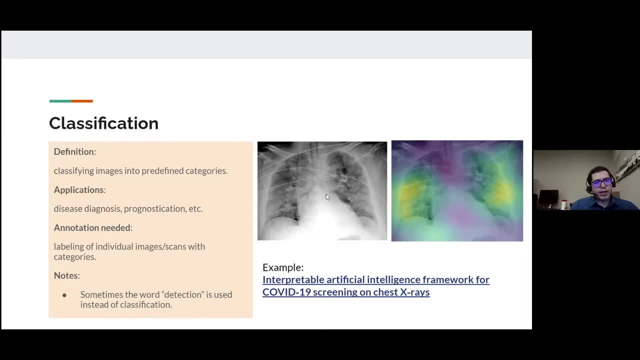 you know whatever. so, and they tried to look at the x-rays and some experts say you know whether or not this patient had covered 19 or not, or even better than that, they looked at some sort of pcr test and say that you know these patients with covet 19. uh, you know a covet 19 like x-ray we. 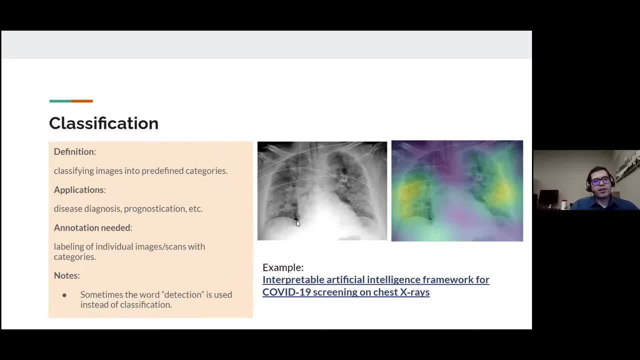 confirmed that had really covered 19, you know, looking at their pcr test for example. so you need to have some sort of labeling annotation for these kind of classifiers if you want to train them in a supervised manner. sometimes you need experts to go through those and label them for you manually, which definitely 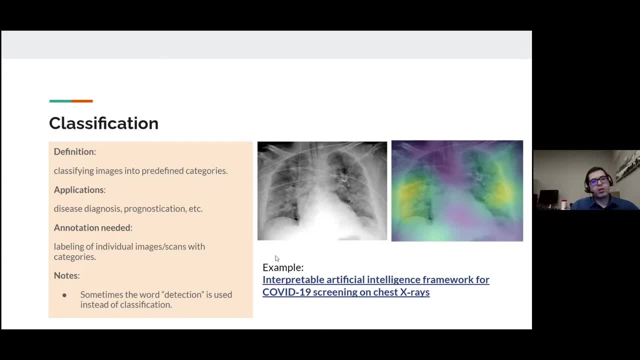 would take more time and energy. sometimes you will have you know, cold standard answers, like from pathological images or, you know, from pcr tests or whatever. so anyway, you should consider the annotation needed for these kind of classifiers. can i ask a question here? sure for sure. so uh, how? 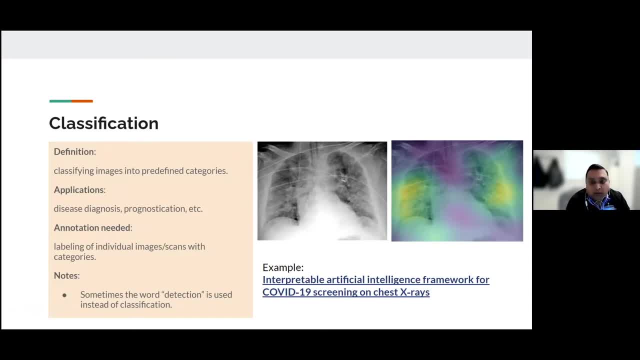 would, uh, the software or the ai model determine a covet 19 lung with with any other fibrosis, like smokers or like countries where there is too much pollution? uh, a related question with that is: so if you have a tissue consistency, let's say in the lung, and with covet 19, you see also systemic effects. 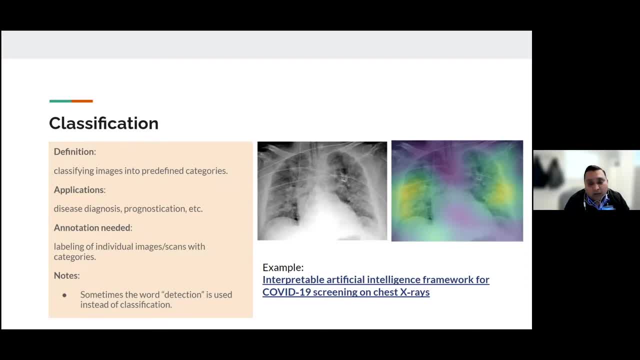 and that image learning ai model can recognize the same consistency of tissue or changes of tissue. so that means you can, you can, see the different, uh, like let's say, in this image. that is hard, okay, so have i made my question here? yeah, i guess i understood you so, so let me go through. 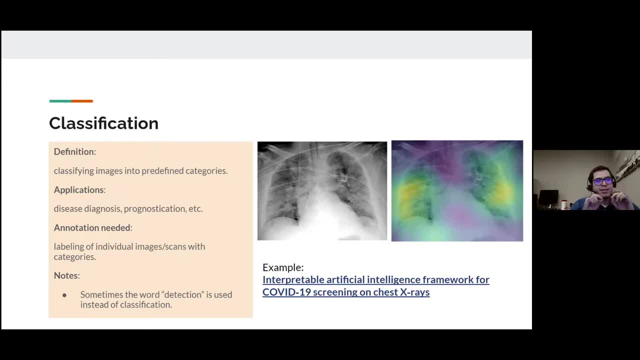 your first question now first. so, uh, you know part of the reason that classification- and you know machine learning engineering in general- is something quite tricky is that you need to pay close attention to what your model is learning. right, you need to provide these models with useful data to learn. so, as you said, 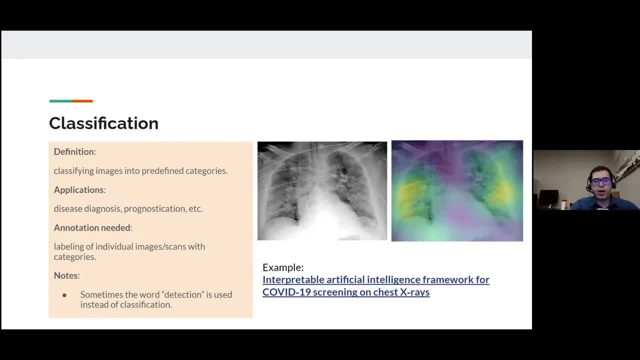 only put, you know, COVID-19 x-rays into a model and then we put normal x-rays, as you know, kind of the other class, to the model and ask the model to understand whether or not patients have COVID-19 or not. the model would probably confuse COVID-19 with all other non-normal type of x-rays that are. 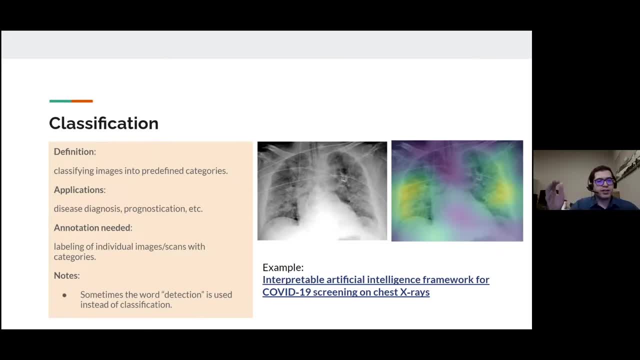 out there right, So other type of pneumonia, interstitial diseases or other things there. So part of the task that data scientists need to do is that they need to put together very accurately built data sets for training. So, for example, in the days of COVID-19, what we wanted- the models. 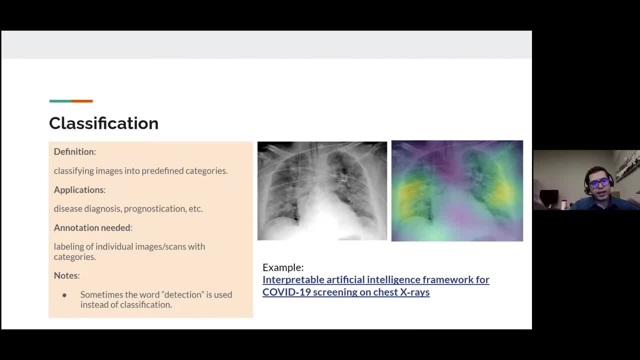 to specifically focus on was to discriminate COVID-19 x-rays from normal patients, but also from other type of pneumonias or, as you said, maybe smoker lungs or, you know, ILDs or whatever other kind of diseases that we had there. So for those reasons, those data sets that you know, 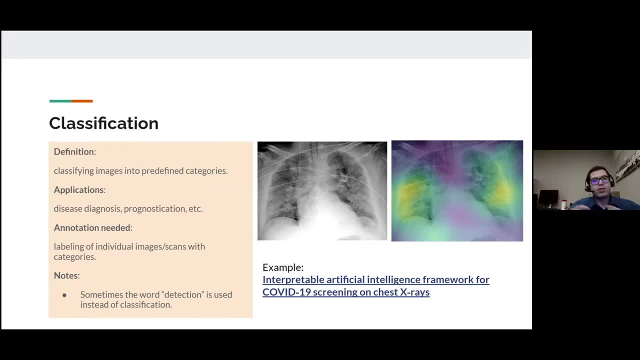 actually resulted in the disease. they were not able to do it, So we wanted to put together a best models. Those were consisting of not only COVID-19 and normal x-rays, but also other classes of x-rays, For example, x-rays from patients with pneumonia, but not COVID-19 pneumonia or from 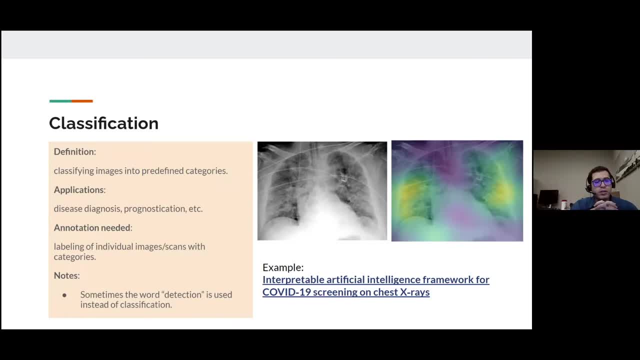 for example, from lungs that had been suffering from smoking or other type of interstitial diseases. So, yes, the answer to your question is that it all depends on the data sets that we are putting together for these models, and we need to be very careful there. Now to your second question. 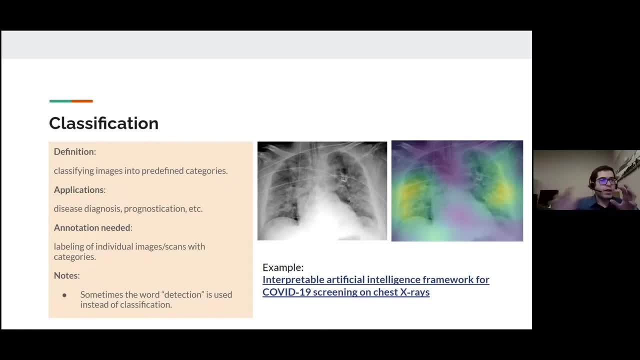 if I understood your question right. so the point is that you know we can, and this is something that we always want to do, that you know we feed in not only the x-rays but some sort of other variables as well. So sometimes we combine imaging variables with clinical variables, So for 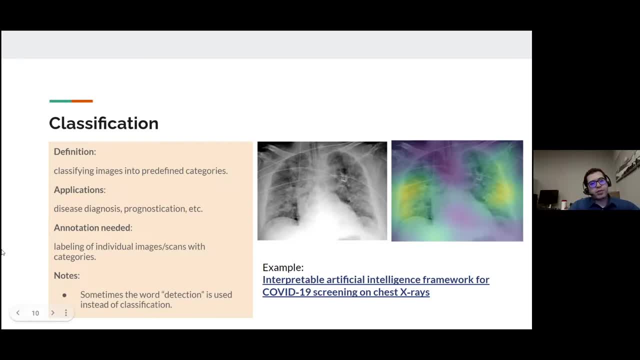 example, say that you know, I trained the same classifier here to realize that the patient has COVID-19 or not. but I also feed in the age and sex of the patients And at the same time I might also feed in- I don't know, maybe some lab data out of those patients, right? So we have, we are. 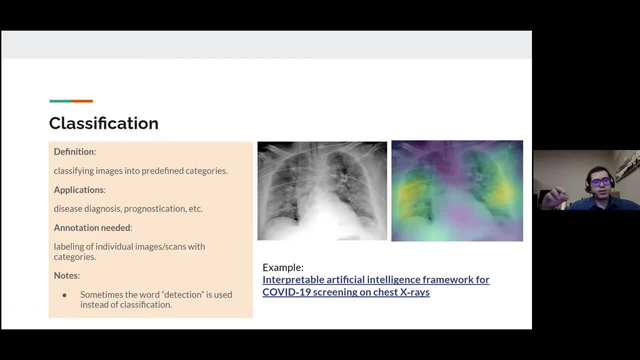 somehow merging clinical data, our tabular data, to say, and this imaging data, right, And this is again going something to be quite useful for the models And if you train your model on multiple type of modalities, say imaging data and tabular data, sometimes imaging and text data, sometimes 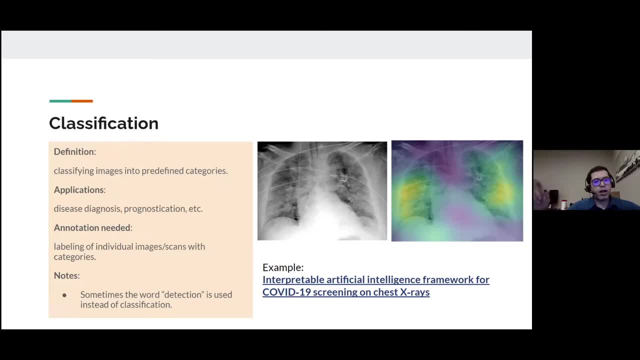 multiple imaging data, say, one CT scan, one MRI, one x-ray from the patient. If you feed more than one modality to your models, then your final models are going to be probably more robust, right? So this concept of multimodal, 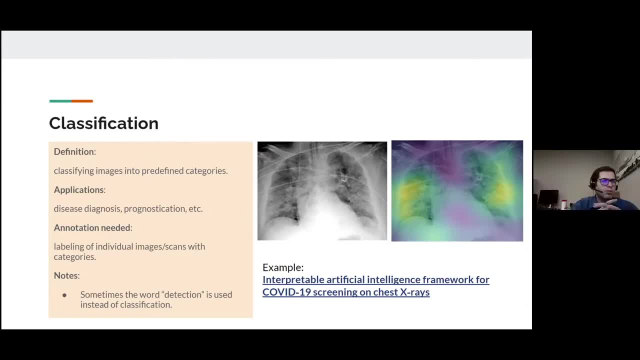 more. fusion training is something quite fancy in today's machine learning. People are almost always interested in doing that, And if you have the data for it, this is very important, And I'm going to talk about this a little bit more when we reach the part that I introduced. that comes to: 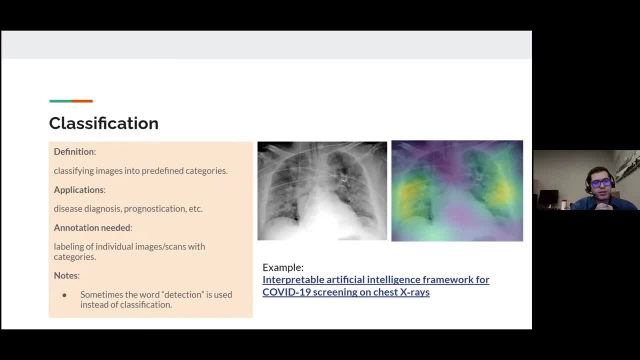 you, because sometimes some of these- you know- tabular data, some of these clinical variables are pretty easy to obtain, but we should not forget about those. Thank you, Right, So let's quickly jump to the second application, and that is the concept of regression. Now, 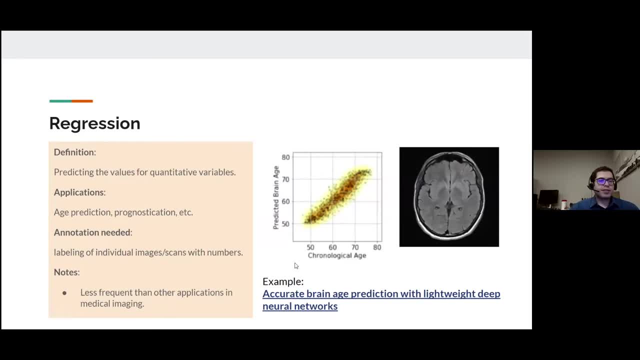 regression. you probably remember from Alex's presentation on tabular data that you know, whenever we are going through a regression machine learning problem, we want to predict the values for some quantitative variables, right. So, for example, you know you put some image. 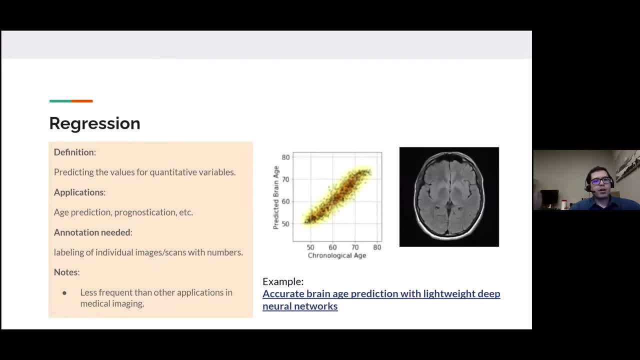 some data regarding the patient's weight, you know sex, you know lab values, things like that, And just imagine the previous scenario we talked about, but without the imaging, and you want to understand how much. you know how many days the patient is going to be able to do that. So you 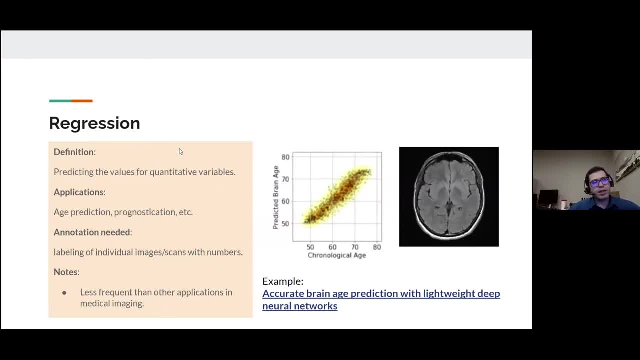 want to understand how many days the patient will survive, something like that. So this would be a regression problem. But when you talk about medical imaging you will not see too many instances of regression applications. We do have some of those out there, but they are not as common as 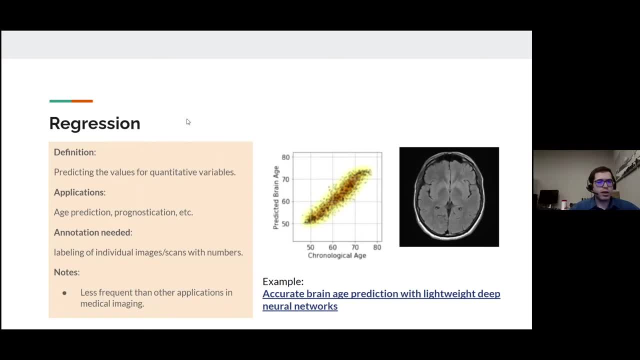 classification or other applications that we are going to talk about. One of the most common things that I remember Dr Erickson and a few of us talked about months ago in the lab was to predict- you know, predict age looking at different parts of the body, For example, looking at brain CT scans. 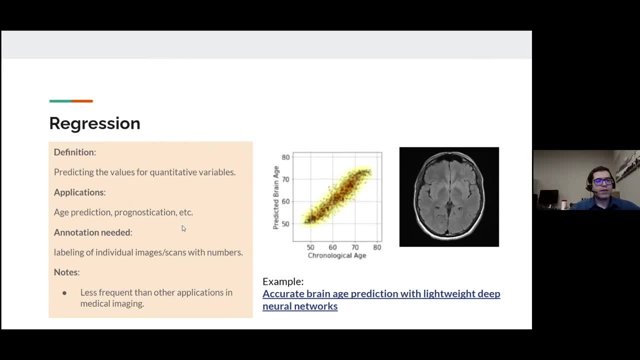 brain MRIs, or you know brain CT scans, or you know brain CT scans, or you know brain CT scans or maybe lung CT scans, things like that. So if you train a model that receives some sort of 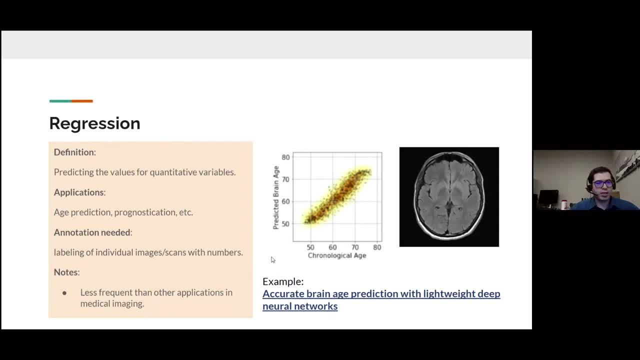 medical imaging as input and then try to predict the age of the patient. this could be a regression model And, you see, if you see this example paper that I put for you here, you could also, you know, visualize how good your model is actually performing by contrasting the chronological age. 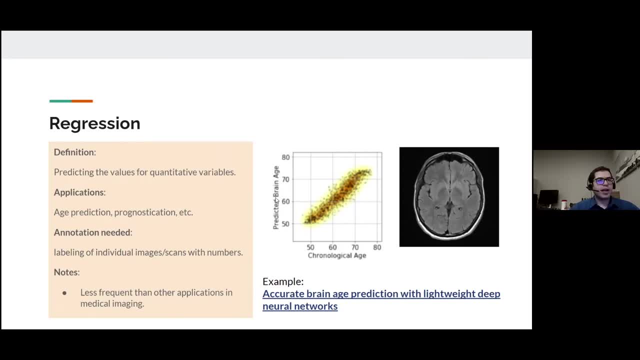 the real age of the patients versus their predicted ages that were actually guessed by the model looking at the imaging data. But that doesn't say this is not something quite common. So if you want to annotate for this kind of machine learning application again, you need to either you know. 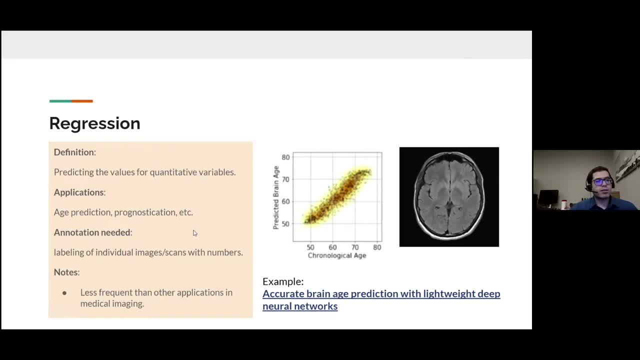 look at your. I mean ask your experts to look at the medical imaging data and provide labels to you. But most of the times for regression, we usually have the numbers as a clinical variable, you know, saved somewhere out there. For example, the age of the patients is quite obvious. looking at their. 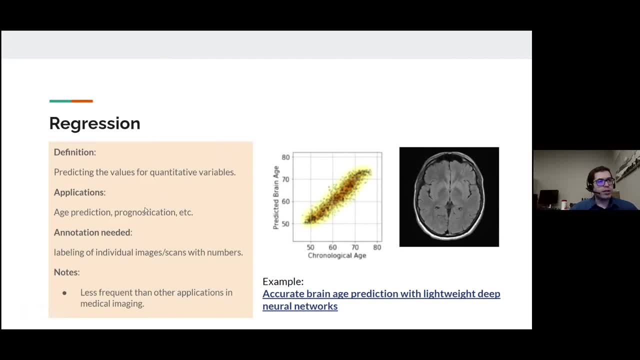 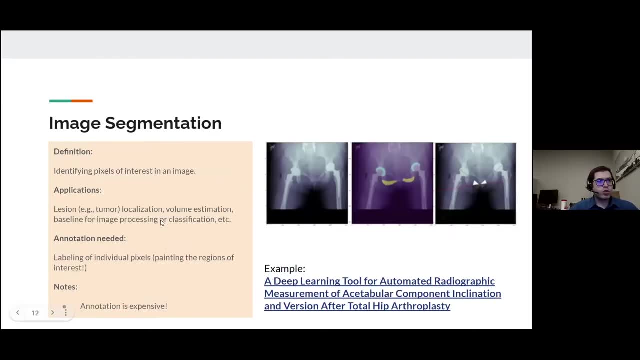 medical record or even their DICOMs. So this is the second application that we talked about. The third one is actually image segmentation. This is quite common in the medical imaging data. So if you look at the medical imaging data, this is quite common, even, you know, sometimes more common than image classification. So you will. 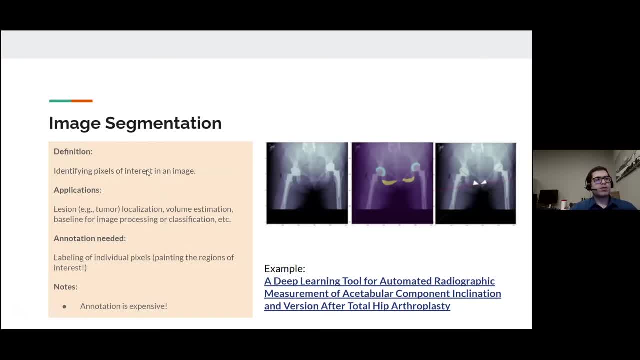 see a lot of examples from image segmentation if you go through the literature of machine learning applied to medical imaging. So image segmentation, you know, in brief, means to identifying pixels of interest in an image. So this is one of our own papers here at OSAIL And if you look at that, 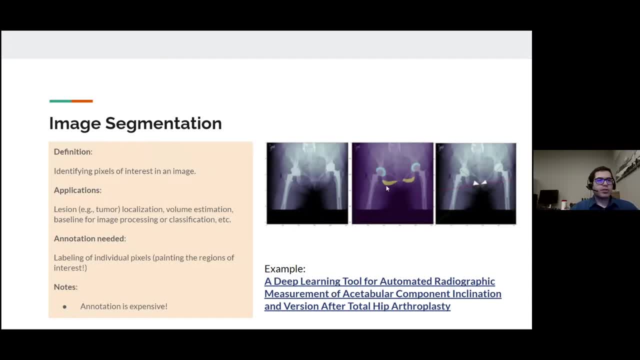 you will see that we wanted to, you know, try to somehow segment these scale tuberosities, these pelvis x-rays and also the cup of the implant put there. So these are totally arthroplasty patients, those patients that need to go through some sort of joint. 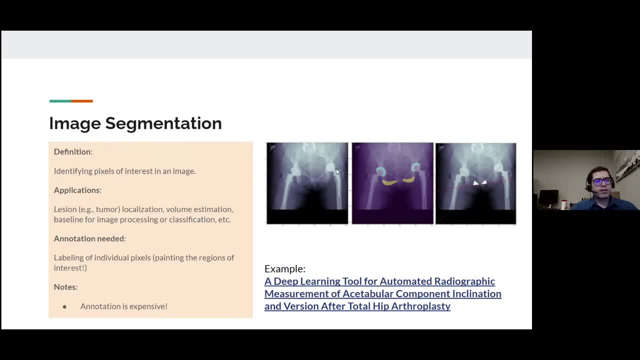 replacement operations And they have these kind of artificial implants in their body. So we wanted to recognize, or better to say, to identify those pixels that belong to specific areas that we were interested in, And to do so using a machine learning model is going to be. 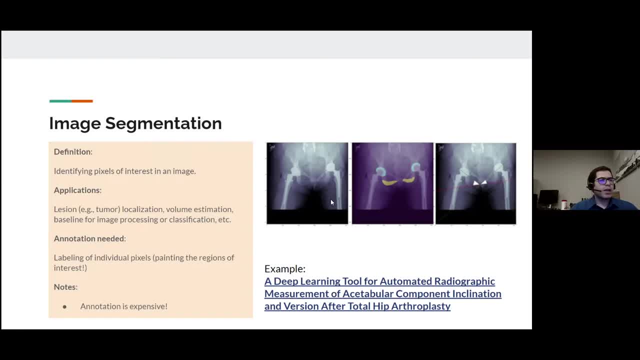 medical, I mean image segmentation or semantic segmentation. Now there are a lot of applications for segmentation. Sometimes people use that for localizing a lesion, for example a tumor, in some medical imaging. You know, suppose that you give a brain MRI to your model and you wanted to quickly understand the exact or accurate boundary. 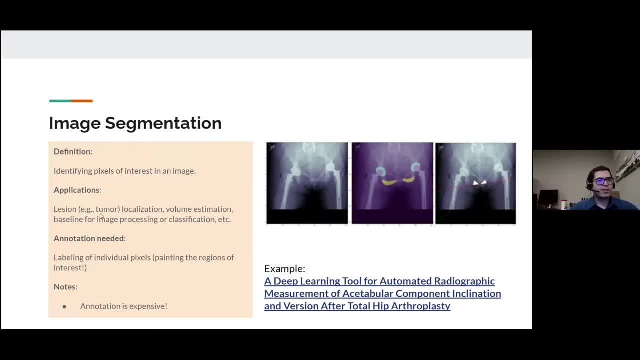 of the brain tumor, a glioblastoma there, for example. So these kind of applications are usually possible using image segmentation models. Sometimes you want to estimate the volume of a lesion And again, if you want to estimate the volume of a lesion, you want to estimate the. 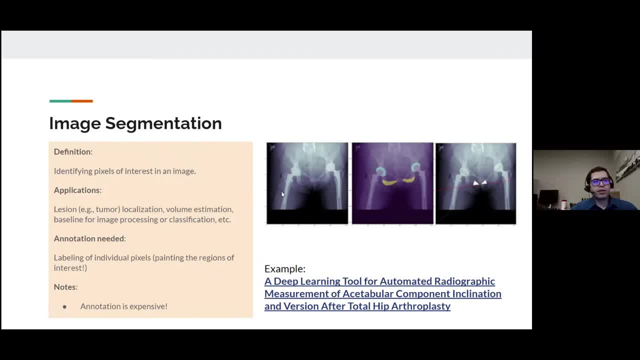 volume of a lesion. And again, if you want to estimate the volume of a lesion, you want to estimate the- that you have an image segmentation model to accurately tell you the number of pixels that actually belonged to that class of interest for you, and then you could do some sort of 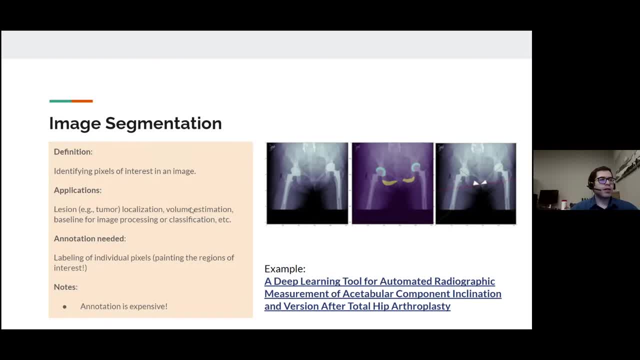 programming mathematical operations to understand the volume of that area for yourself. Or, as we did in this project, sometimes image segmentation is the baseline for you know some sort of further image processing algorithms. Now, the kind of image processing that we did in this project- and image processing, you know, doesn't need to be done using AI, for example. 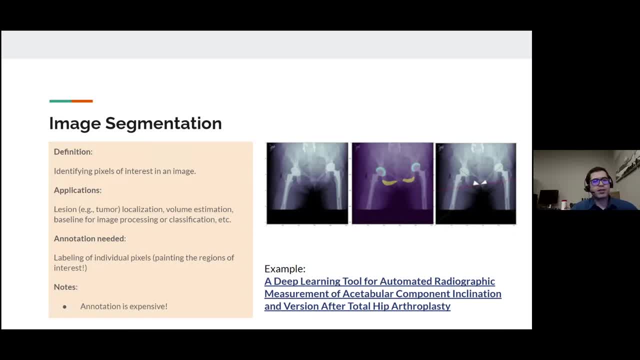 in this project. it was pure python code without any kind of machine learning. there. the machine learning step actually happened earlier, so we fed a pelvis x-ray like this to our models. we received a segmentation mask like this one, so we did know what pixels actually belonged to ischial. 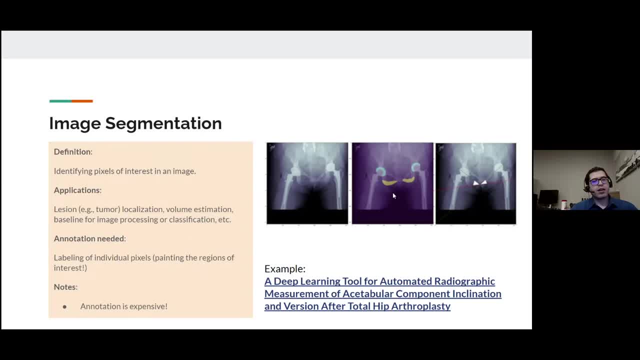 tuberosities or to the, you know cup of the implant here, and all other pixels were zero. and then we did some sort of image processing on that to draw these lines that you see here and finally measure these angles that these green and red lines build with each other. we 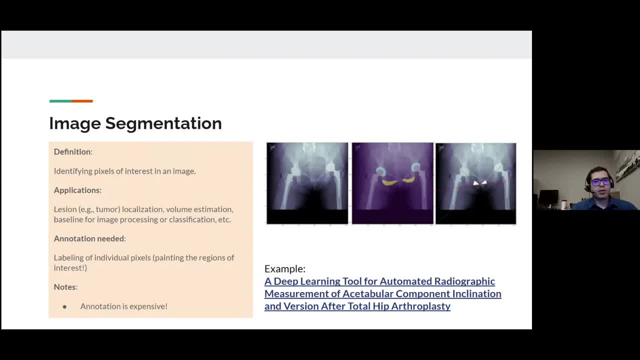 were interested actually in this kind of acetabular angles for some sort of orthopedic application. so sometimes people you know, combine segmentation with further image processing. so medical image segmentation a lot of time is actually one component of the pipeline, not the entire pipeline for itself. so it is good to have this in mind. oh, the important note here is that annotation for 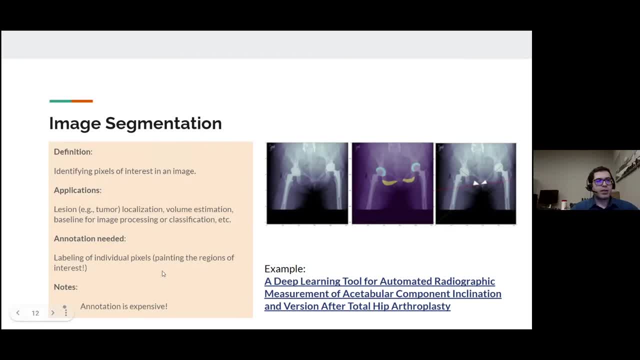 these actually takes a lot of time right. so medical image segmentation is one of those applications you need to spend a lot of time for annotating. one or two people at least need to go through that they. we have a specific software that people can use and basically what they do is that they. 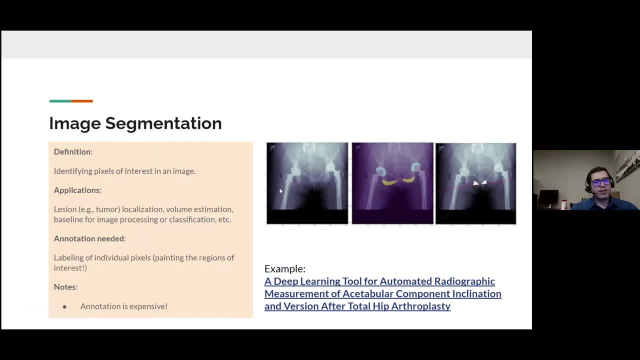 try to, you know, manually segment some of these pelvis x-rays or you know whatever other image data that you're interested in using mouse, so they basically paint the objects of interest using their mouse and then when we have a lot of manual annotations, then we feed all those. 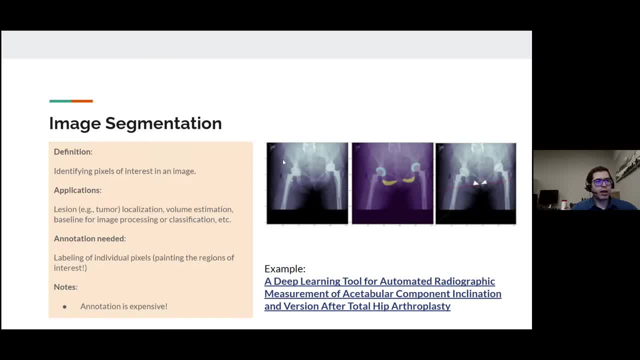 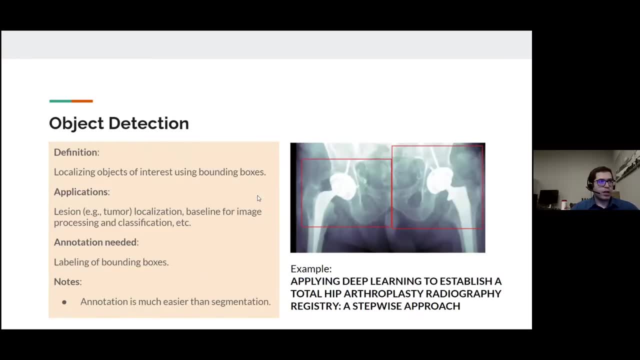 to a machine learning model, and machine learning model will hopefully learn how to automatically those areas that we care about. so this is called image segmentation. now, object detection is actually the force application. now, object detection, you know, is somehow similar to medical image segmentation, but to be honestly, i mean less. 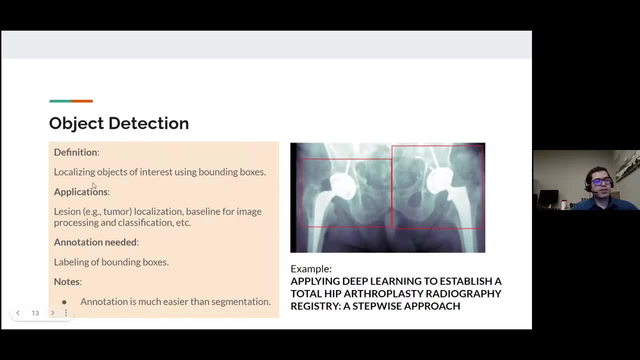 accurate. so the the intention of object detection is that we are going to localize objects of interest, but we are not going to care about individual pixels. we only want to understand or, better to say, to estimate the rough area for an object or tissue or lesion of interest. 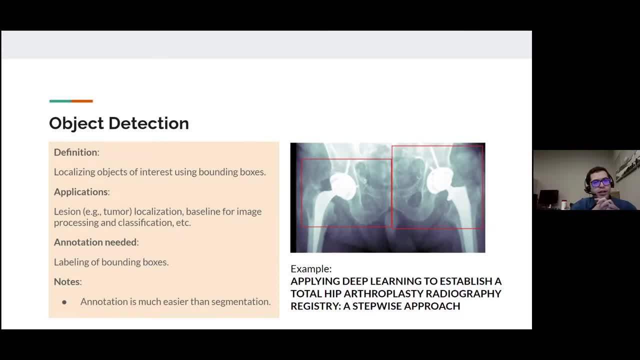 now, for example, in this study that you see on the right- and this was again one of our own publications- we cared about understanding, uh, the, you know, estimated location of the head of the implants. right, we didn't care about the exact location, but we wanted to crop the images to be 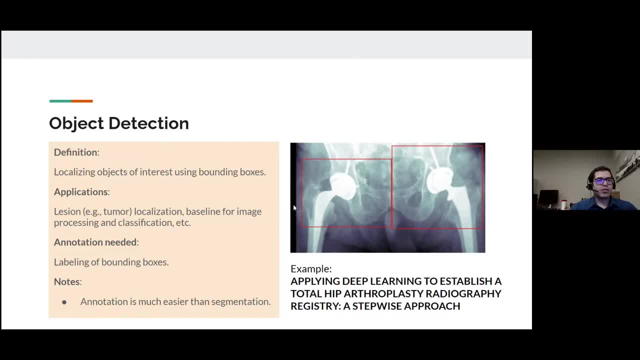 honest, we wanted to use these, uh, some sort of areas in order to crop the images and then, if you are interested, feed those cropped images to a second machine learning model to do a classification. so basically, object detection could also be put together with other type of algorithms to be a pipeline, but, uh, you know the object detection itself, the only. 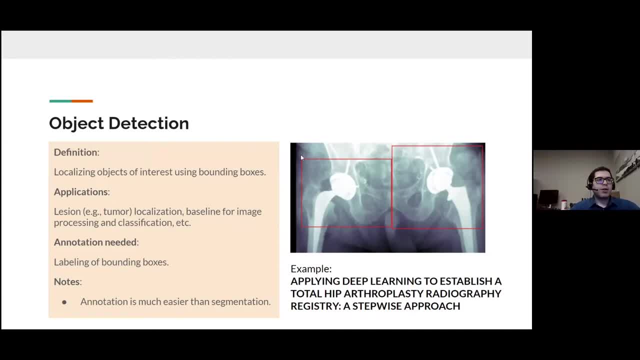 thing it did for us was that it actually denoted these red rectangles for us, saying that you know, this is probably the area that you are interested in, so it helped us to focus on that area that we wanted. so, if you, if you note here, it has not segmented the implant for us, or? 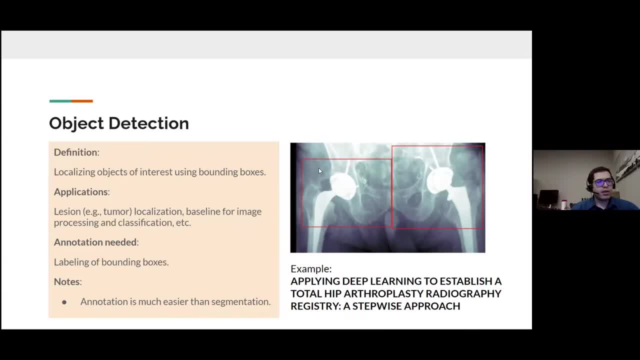 bone for us. We do not know the pixel value for anything here, but we do know the rough predicted area for some sort of objects or tissue that we were interested in. So this is called object detection. Now you might ask, why do we need object detection at all if it is less accurate? 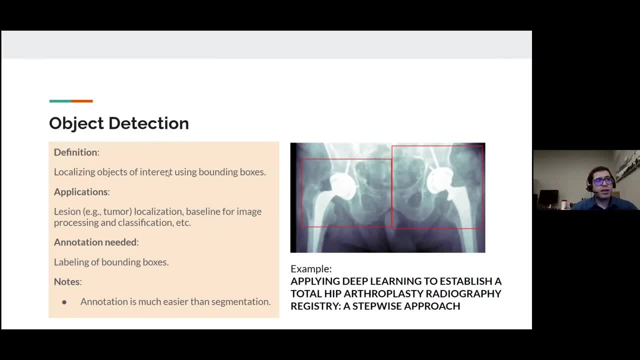 than a medical segmentation algorithm. And the answer is that, as I told you, annotation for segmentation is going to be too much expensive And you know, annotating for this one is going far easier, So I have done both. If you want to annotate data for an object detection model, 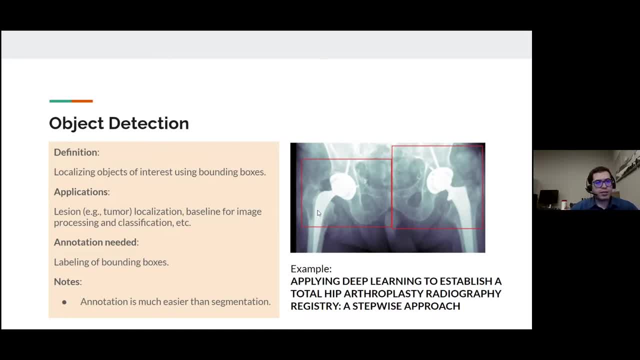 you just need to go through a software again, but this time, instead of painting every single pixel by yourself, you are just going to draw a rectangle around that, and this is going to be quite easy, right? So this is a good question to ask yourself If you're interested in localizing. 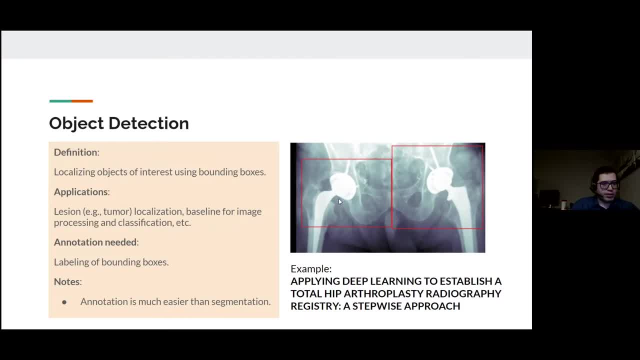 an object. do you really care about the values of individual pixels or not? If you do, then you probably need to proceed with the segmentation model. If you do not, then maybe an object detection is going to be a more feasible approach for you. and finally, i would like to talk. 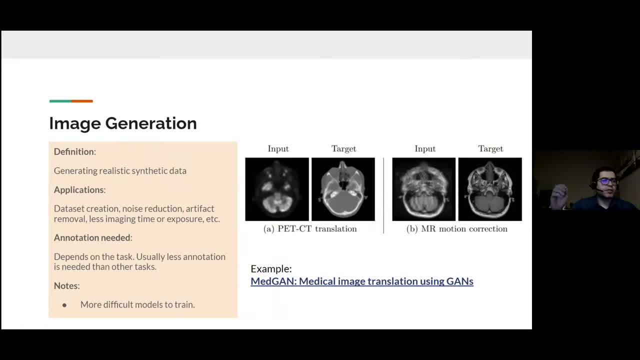 about image generation, which is actually the final, or better to say, the final important application of medical, of machine learning applied to medical imaging. now, image generation is actually my own interest. it is something quite exciting to talk about. so you know that these machine learning models are very powerful, and they can even generate images that do not exist for us. so 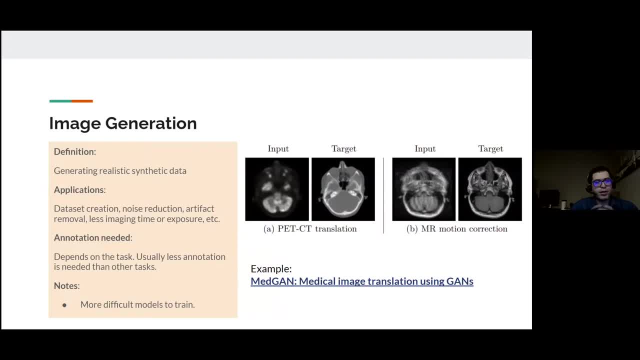 i once tried that and it failed, so i'm not going to show you right now. but if you are not on meo intranet or meo network, just try to google- this face does not exist- and open that. there is a website there and there is a button. the website is quite easy. there is a button there, you just 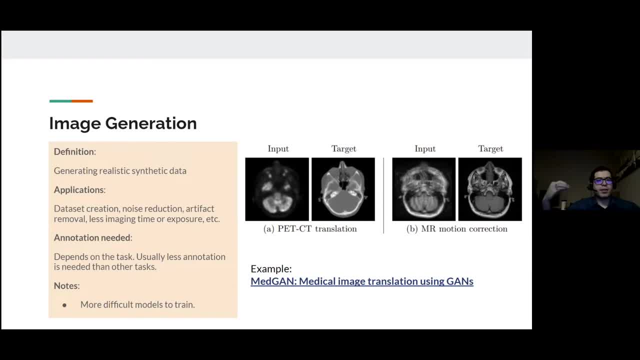 press generate and you will see a complete, realistic image of a person's face. but, to be honest, that person does not exist, so that image was quite synthetic, built using a machine learning model. so this kind of image generation is going to be a very important part of the machine learning. 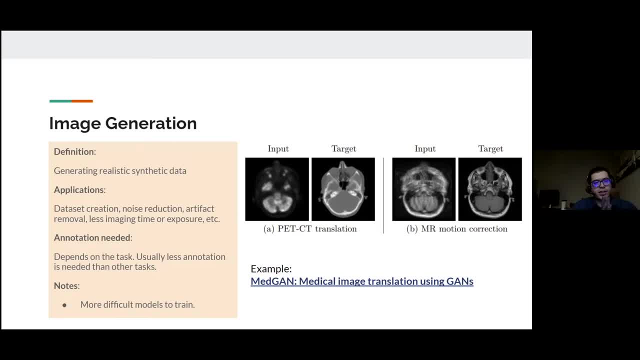 the most important or the most famous architecture used for image generation that you will probably hear a lot about, if you're interested in such topics, is gans or you know uh, generative adversarial networks. so if the architecture itself is not that much important for now, but if you are interested, 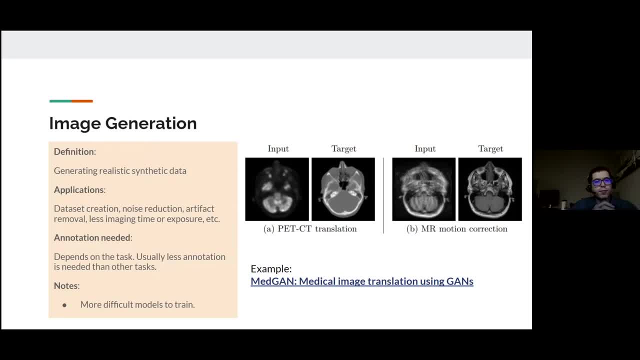 in that just search gan keyword and put some sort of medical uh keywords that you are interested in in addition to that and go through google and see what you will find. now, image generation in medicine could be used for a lot of purposes. for example, we could use: 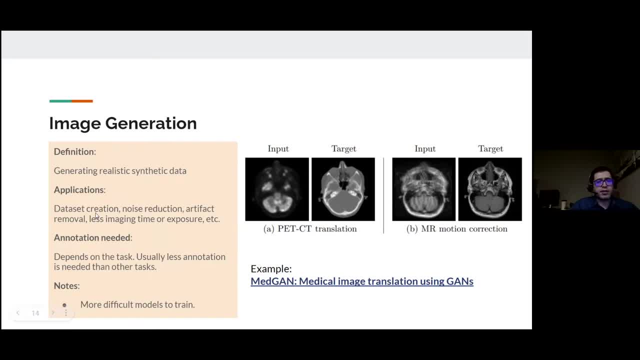 that for data set creation. you know that machine learning almost always needs a lot of data, specifically if you are working with deep learning. so the problem that many researchers have is that you know we do not have too many medical imaging data or you know other type of modalities available. 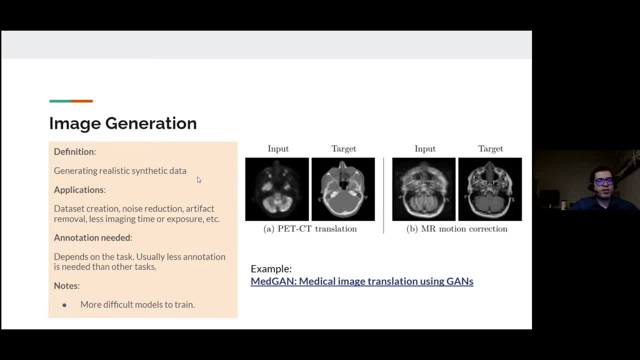 to us. so sometimes people use these kind of generation models to create synthetic data sets for themselves. suppose that i have 10 000 pelvis x-rays, but i need millions. but can i do? one strategy could be to train a gan or an image generation machine learning. 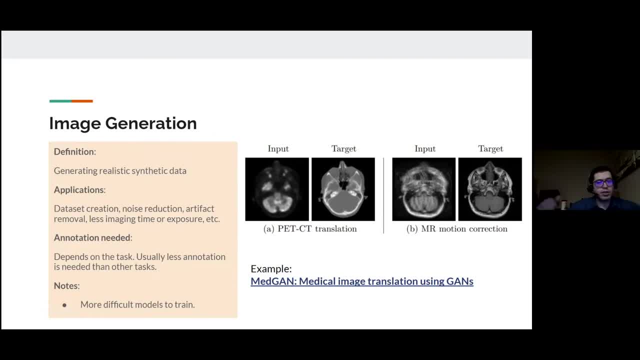 model to create more pelvis x-rays for you. of course, the value of those synthetic x-rays for the model is not going to be, uh, similar to the original- you know real x-rays that you could have found- but this is going to be still super useful. we could also use that for noise reduction. so for 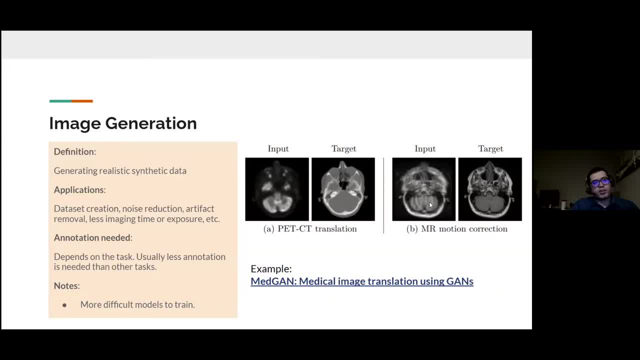 example, if you look at these, uh, you know two images on the right side some gans have been used for motion correction in mri. so if you can use some gans and some gans on another model, you can use that for another experiment. make sure that you have already used gans in other scenarios, like 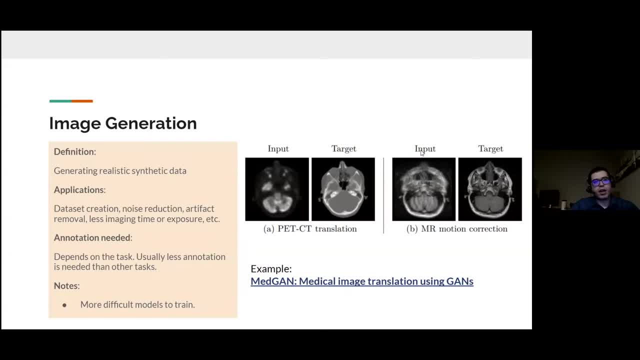 So artifacts actually had been removed from this input MRI using some sort of artificial neural networks here, And we could also use that for less imaging time or exposure. So one thing that we can do is that we can probably pick a PET scan here and then try. 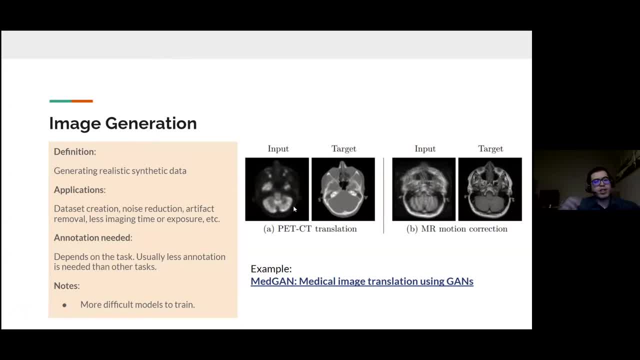 to apply a machine learning model to that to generate a CT scan quite similar to that cut that we were looking at. it's PET or an MRI for the same cut. So this is quite something fancy. Many of the colleagues in our lab have already done these. 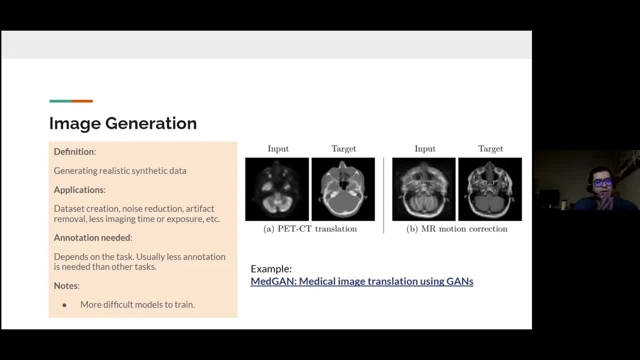 In Dr Rickson's lab we had colleagues who actually created a model that was able to convert a T1 to T2 MRI And we also have amazing colleagues who could actually achieve increasing the resolution of some sort of 3D imaging data like CT scans or MRIs. 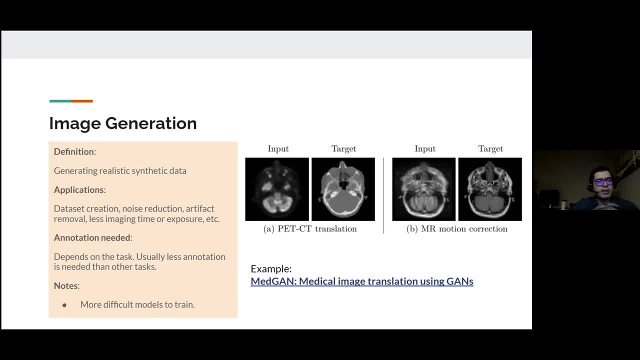 So there are a lot of applications for that. Just feel free to search for that. And image generation is something that is actually getting more and more attention these days. So that was the end of part aim one, part one to be able to say we went through some. 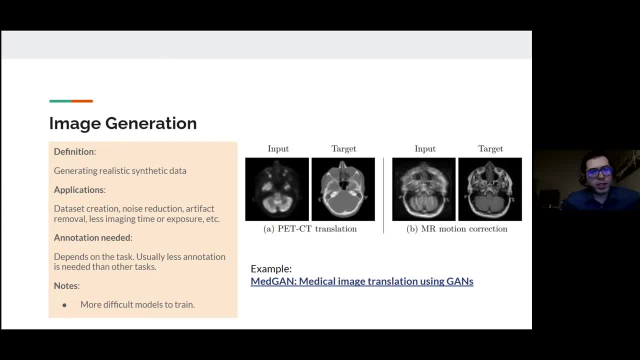 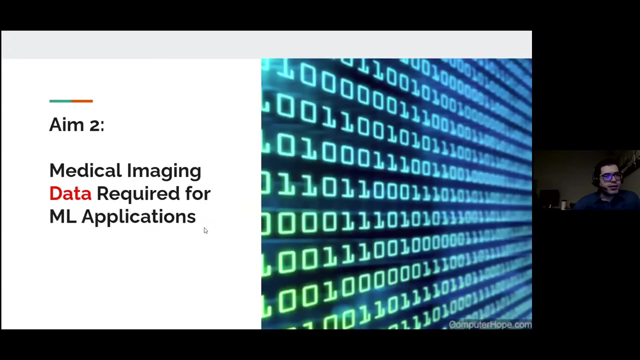 sort of application, And I would like to pause here and give you some time to ask your questions or hear your comments, if you're interested in sharing anything with everybody. No questions, Perfect. So this is good news, As we can have more time for aim three, which I was personally more interested in. 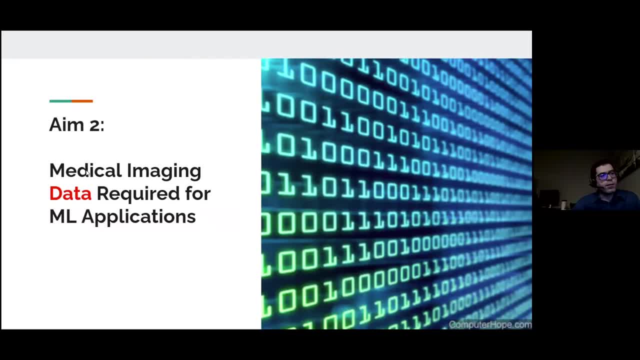 But let's proceed to aim two, which is now about medical imaging data itself. So you probably have now a general understanding of what is going to happen in the world of machine learning when we apply that to medical imaging data. But let's talk about the second component now. 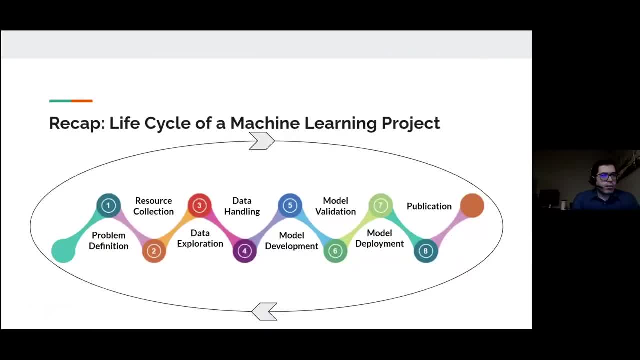 What is medical imaging data right? So before we go through this process, it's good to remind you of this lifecycle of a machine learning project that we've been doing. So we went through in our first workshop. you do remember the different steps that we 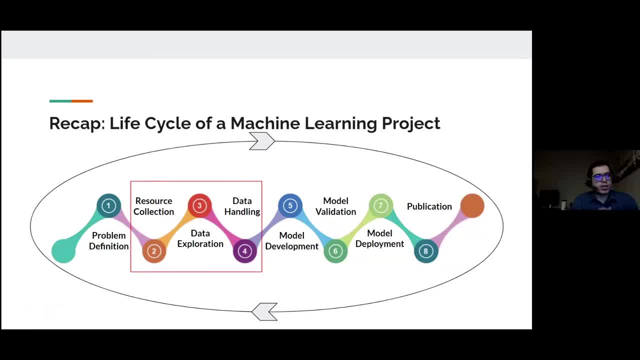 needed to go through whenever we wanted to run a machine learning project And in this specific aim. I am going to talk about three steps here: resource collection, data exploration and data handling. So whatever slides that we are going to review with each other belongs to these three steps. 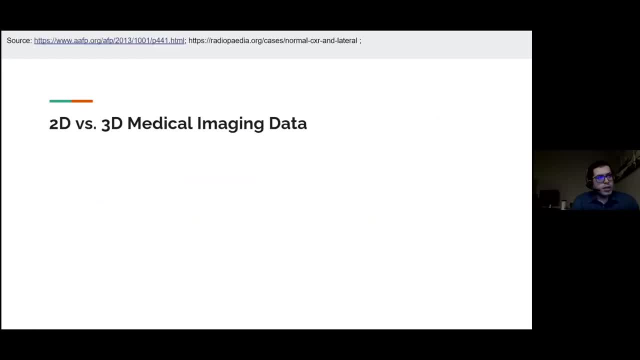 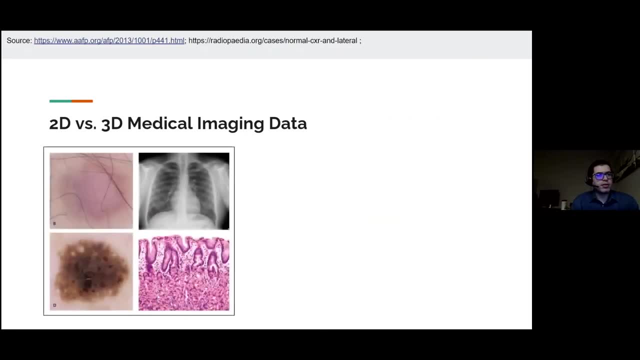 of the general pipeline that we had put together. So let's talk about first 2D versus 3D medical imaging data. You probably all know about this before, But only as a quick recap. So in medical imaging world we have many different types of imaging available to us. 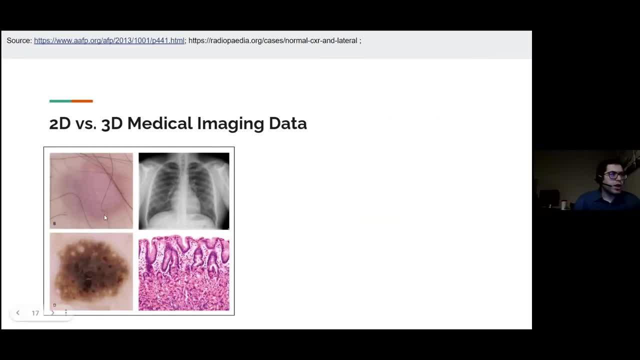 We have some imaging, for example, that dermatologists work on, And they look like natural images, at least are much closer to natural images than radiology images. They have these images of skin And you see that those are colorful images that could be quite similar to other natural 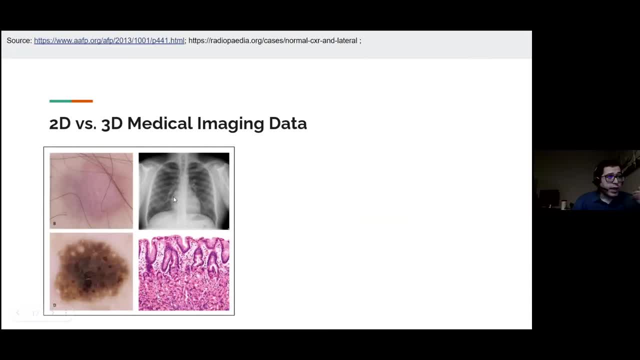 images like nature images and things like that, But we also have 2D radiology images, which almost all the time may mean X-rays, And then we also have pathology slices that, again, pathologists work on, And AI and machine learning has actually advanced a lot in both radiology and pathology. 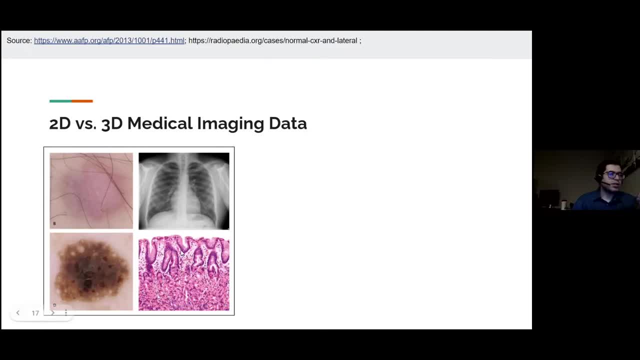 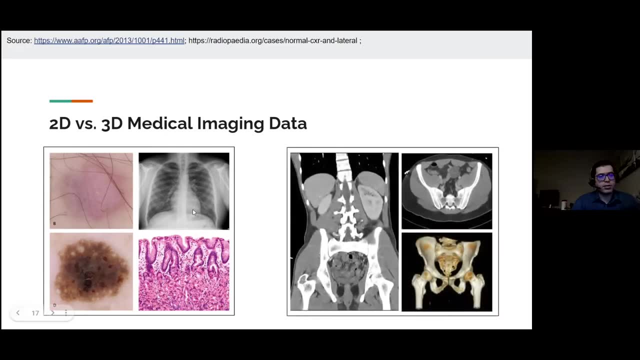 So you will probably see a lot of applications of that already published in the literature. But as opposed to this 2D type of data, we also have 3D data available to us And, as I told you, this is where the term computer vision might be a little bit tricky. 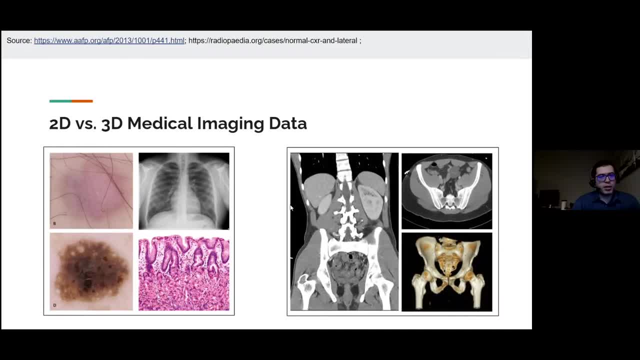 to apply to machine learning for medical imaging, Because we do have CT scans, MRIs and this kind of 3D data. I know that they are originally built of some 2D data that are stacked on top of each other, But we can actually generate 3D rendering out of those, like this 3D rendering of pelvis. 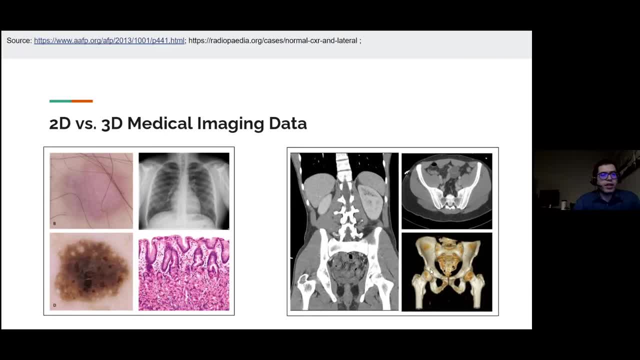 bone here, And this means that we are somehow dealing with 3D data right, And we can actually obtain more than one 2D view of, for example, sagittal view, coronal view, axial view. So we do have access to a kind of medical imaging, to a kind of imaging data. 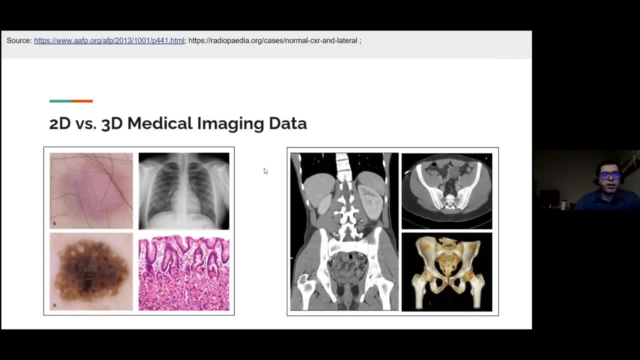 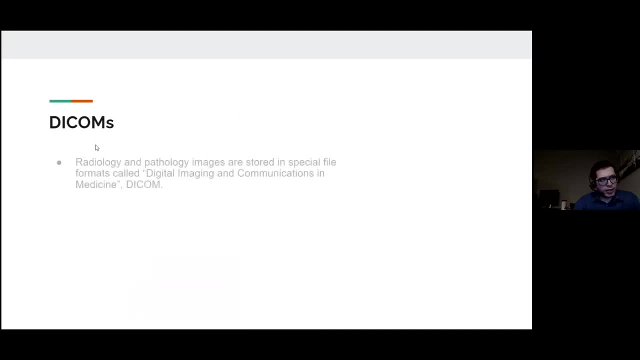 That is somehow different than those non-medically oriented engineers work on in real machine learning world. So we need to be careful about this data, And this is actually what makes imaging data and machine learning quite interesting. Now, another topic that I would like to introduce to you again. some of you might already be. 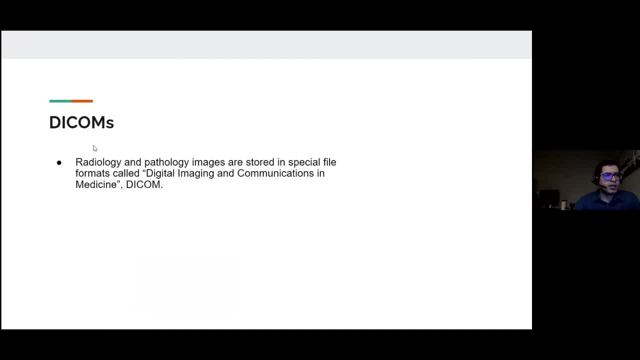 familiar with is the definition of DICOMs and their application. So DICOMs are actually a specific type of data and also a protocol for data transfer. So you know that most of the research, Most of the radiology images- you know- I can't even say all of those- and some of the pathology, 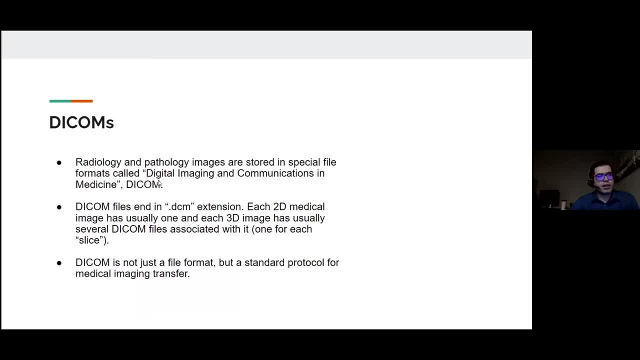 images are stored in a special file format called Digital Imaging and Communications in Medicine, which is abbreviated as DICOM. right Now DICOM files end in DCM extension. You might have already seen those. Sometimes you download them from different databases or data sets. 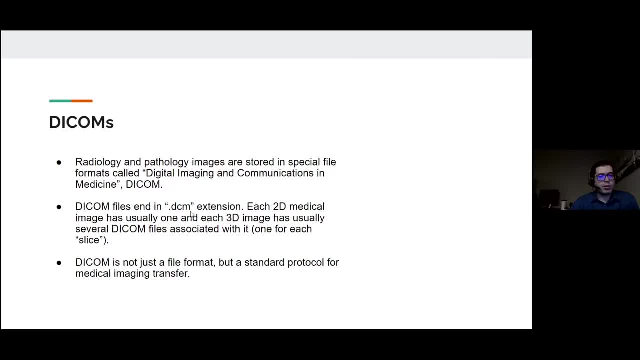 So whenever you saw a file that ends in DCM, it's probably a DICOM file, But it's important to know that you know when you go through, for example, a CT scan or an MRI, it doesn't mean that that CT scan or MRI is going to be saved only on one DICOM file. 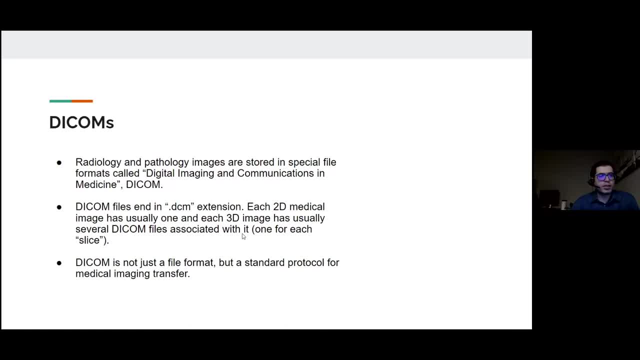 We usually store X-rays or 2D medical imaging data on one DICOM file, So one X-ray could be- I mean, one DICOM could belong to one X-ray. But when we talk about 3D images like CT scans, MRIs, 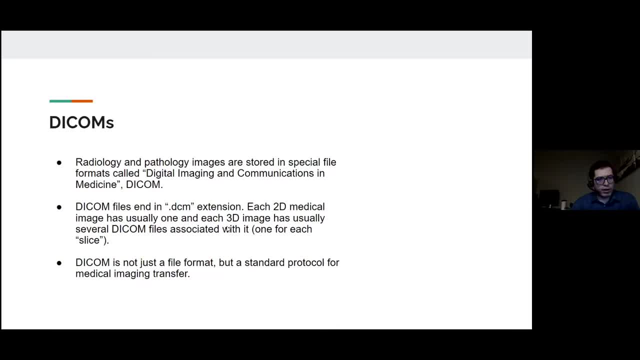 so those usually are stored in multiple DICOM files, right? So, for example, if a CT scan has I don't know, 20 COTS, 20 axial COTS, then you probably are going to see 20 DICOM files associated with that single study, right? 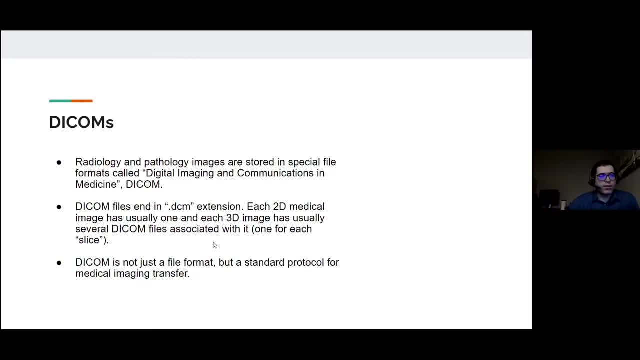 So there are ways, there are attributes in DICOM files that make it possible for PAC system, and also for those who are interested in working with DICOMs directly, to understand which DICOMs actually belong to each other. For example, they form the same CT scan. 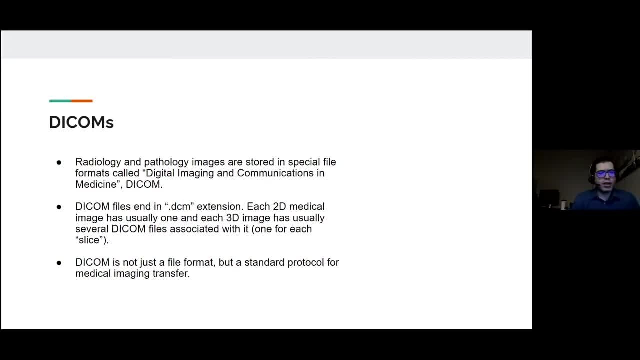 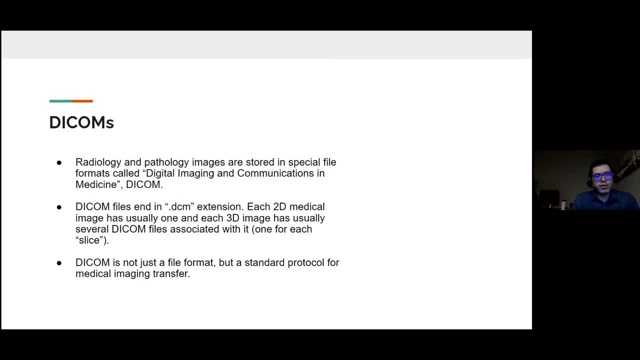 But for the purpose of this presentation it's only important to know that DICOM- I mean one study, one CT or MRI study could go to multiple DICOMs. And the second important point is that DICOM is a tricky term. 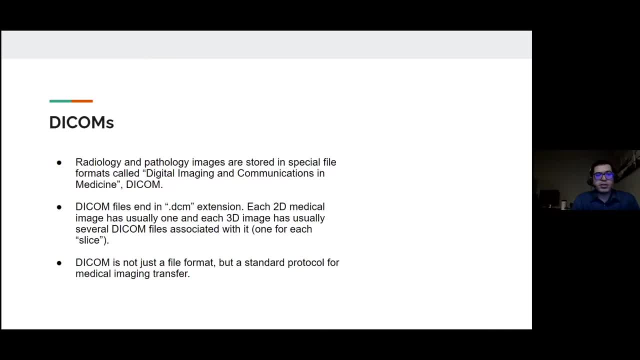 because it not only denotes a file format but also denotes a standard protocol for medical imaging transfer. And this is important to know because you know, DICOMs are the magic behind all these different PAC systems that come from different vendors, but they are capable of opening, you know. 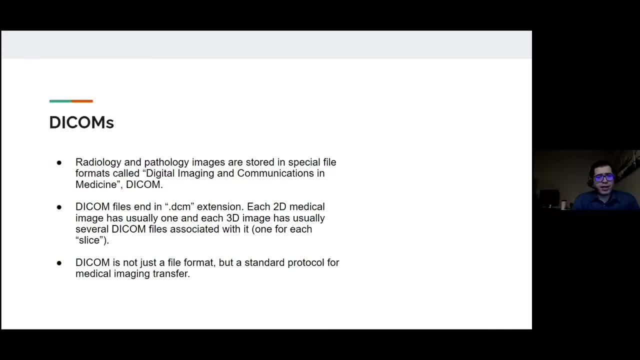 all radiology images or some pathology images, regardless of where the patient has actually gone through imaging, right, So I can go through an imaging here at Mayo and then my DICOM files could be easily read in another country, because this is a kind of protocol for data transfer. 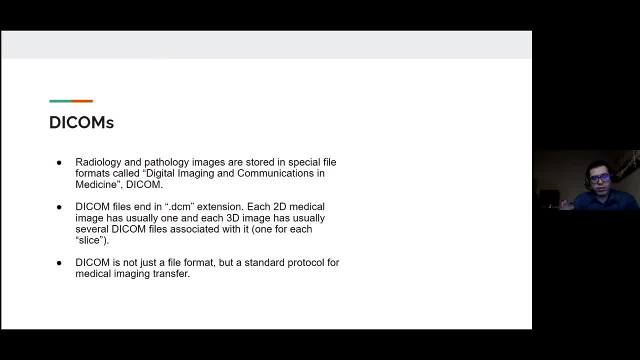 PAC systems. all PAC systems know how to read DICOM files and how to convert those to real images that specialists could look at when going through them in PAC systems or DICOM viewers. Now the final important point- and this is what actually makes DICOM quite interesting- is that 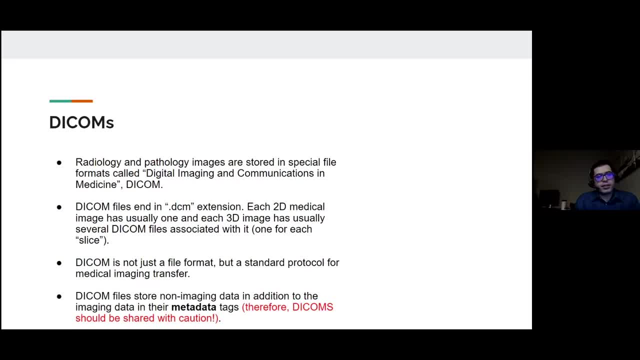 Now the final important point- and this is what actually makes DICOM quite interesting- is that DICOM files store non-imaging data in addition to the imaging data that they include. So this is important. So if you have a DICOM file that belongs to a chest X-ray from a patient, 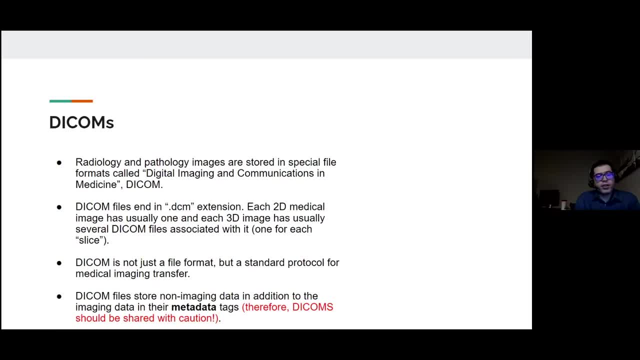 that DICOM file includes some other information, some other data, rather than the imaging itself. It does have the imaging, but it also has some other kind of variables in that which are usually, you know, coded as a small text there. So what kind of variables I mean, can we you know? 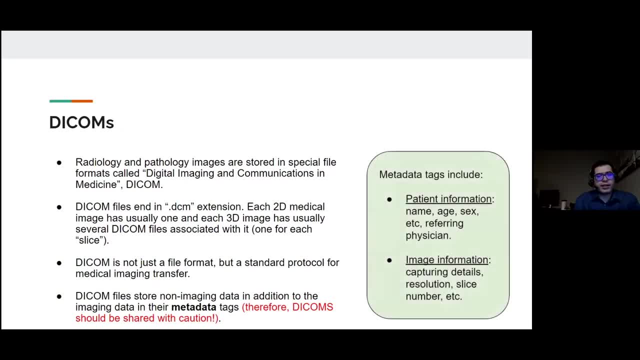 So what kind of variables I mean, can we you know? So what kind of variables I mean can we you know, can we find in DICOM files, rather than the imaging itself? So the two important categories are: one: the patient information. 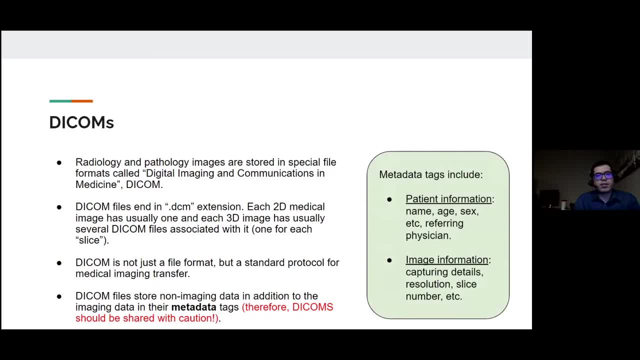 For example, you will find patient name, patient age, sex, you know, referring physician, whatever data that might be recorded there, And this is not something consistent. Sometimes different institutes have different protocols for what to put in DICOM form files. 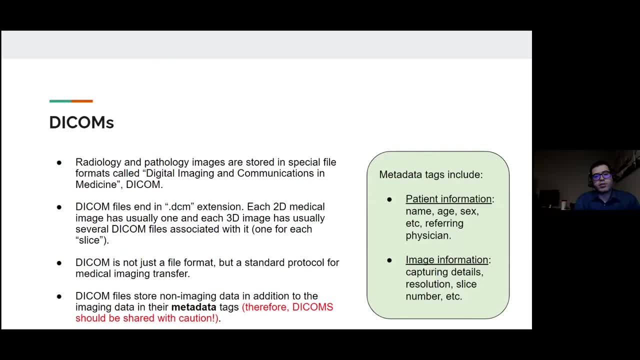 And then we also will find some additional information or additional data regarding the imaging as well. For example, you know we understand the range. For example, you know we understand the range of the pixel values. We can understand something like the resolution. 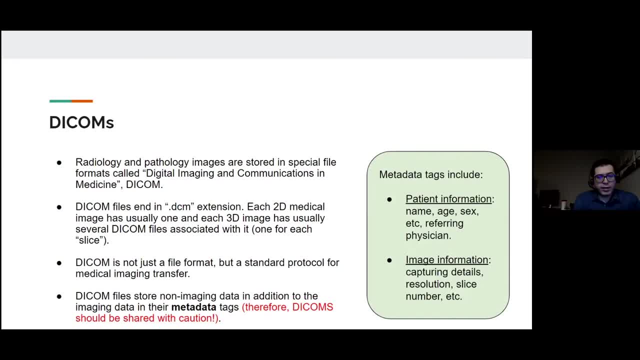 We can understand the slice number If the DICOM, for example, belongs to a CT scan And, as I told you, there are also attributes there that will help us to understand if this DICOM, for example, is the fifth axial slice from a CT scan with 20 slices. 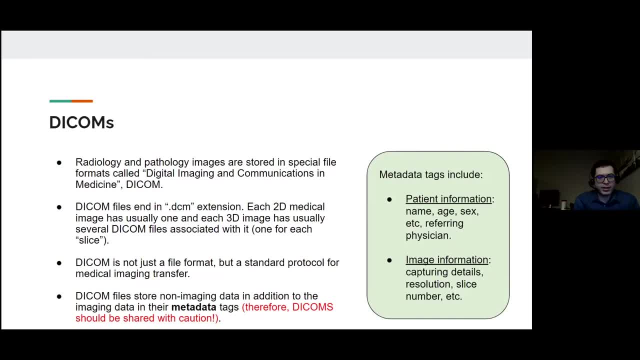 You know, if I look at one DICOM file from a CT scan, I can easily understand this: How many slices were there in total, And which specific slice is this DICOM talking about, right? So these are the kind of data that is actually. 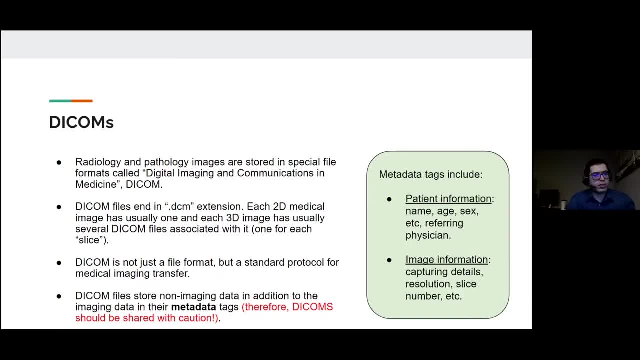 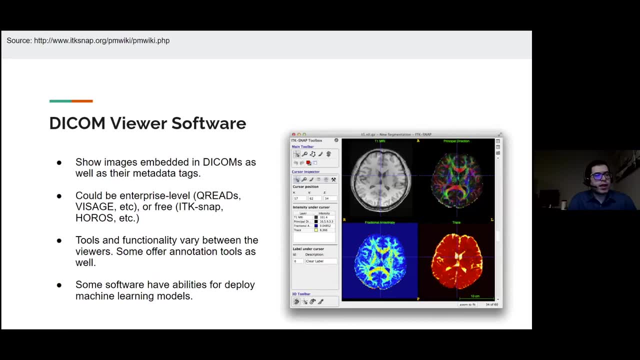 also stored in DICOM files in addition to the imaging data, So this is important to keep in mind. Now, as you probably can guess, we do have a lot of DICOM viewer software, and those are designed to show images embedded in DICOMs. 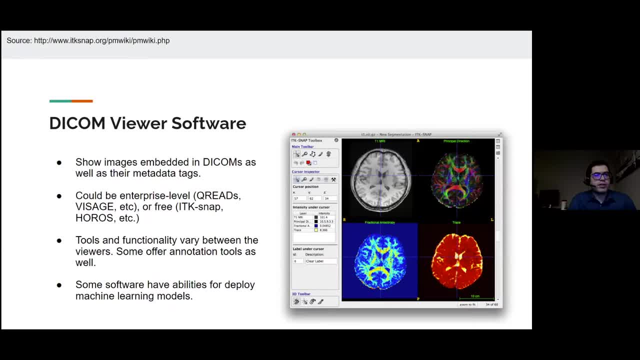 as well as their metadata tags, right? So if you go through some of this software, you are going to see the patient's name. You are also going to see their imaging, for example, MR, CT, X-ray and a lot of other things that are stored in DICOMs. 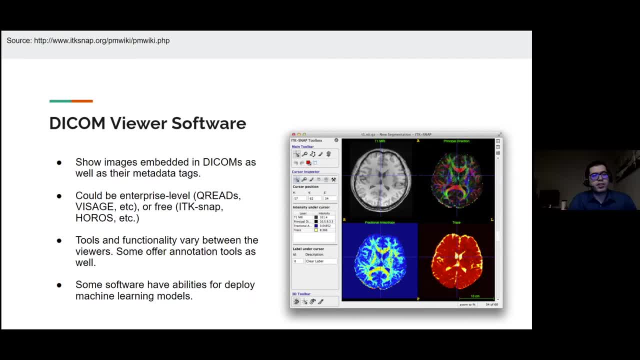 could also be used, And definitely the software use some of those imaging and metadata. So that's one of the attributes that DICOMs store: to visualize these images to you in a way that you find appropriate right, And we have a lot of DICOM viewer software. 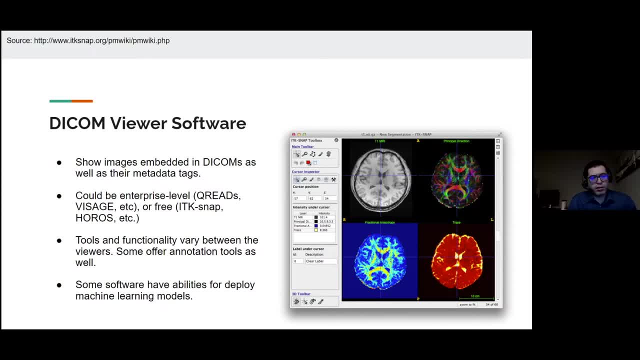 Some of them are at enterprise level. you know QReads, Visage- Those are the ones that radiologists here use. You probably have used them before- And we do have some sort of free or out-of-charge open source tools available to us that most of the time, data scientists 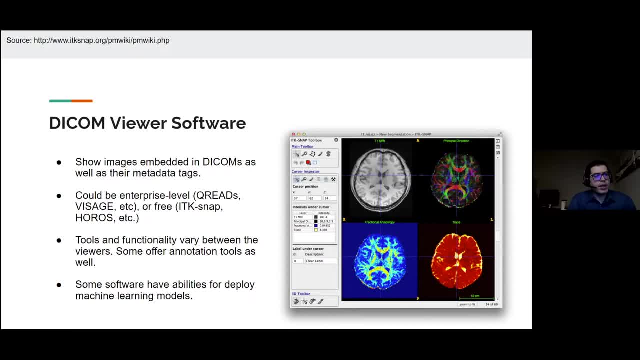 are more interested to work with, because they could also be used for image annotation, for example, And the most famous one, if you want to search for them, are ITK Snap Horus, which I believe is for Macs, And we do have 3D Slicer Reel Contour. 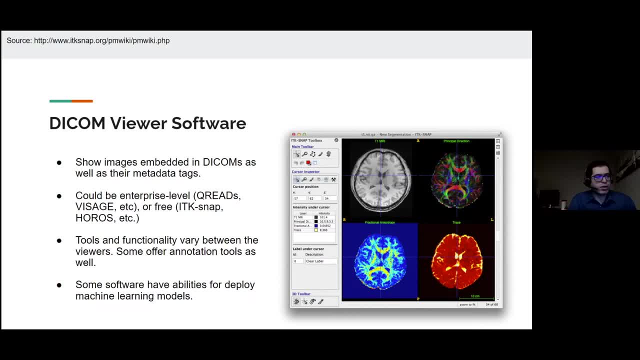 So there are different types of those available. If you are interested, just search for them. You will find a lot. Tools and functionality definitely vary between these tools. Some offer annotation tools, as I said, And you know, some software also have abilities. 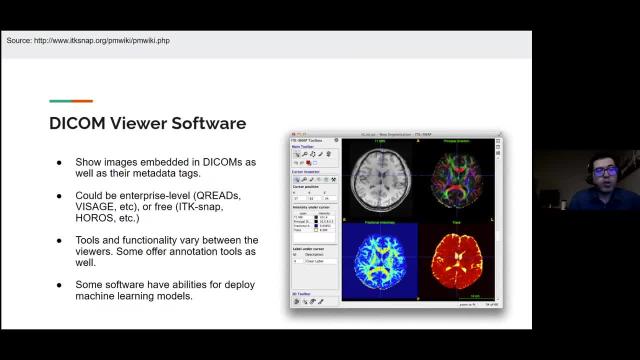 to deploy machine learning models. So this is important, right? You might wonder: if I train a machine learning model that could be applied to medical imaging data, then how am I going to use that in real practice, right? So this is an important question to ask. 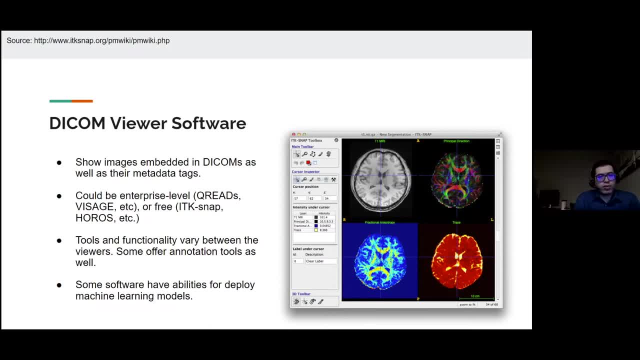 And this actually is related to a very important area in machine learning that is called deployment, or deployment of machine learning models, And in medical imaging world this is also quite important because we already have a very established icon viewer software in each institute, So we need to find a way to add machine learning. 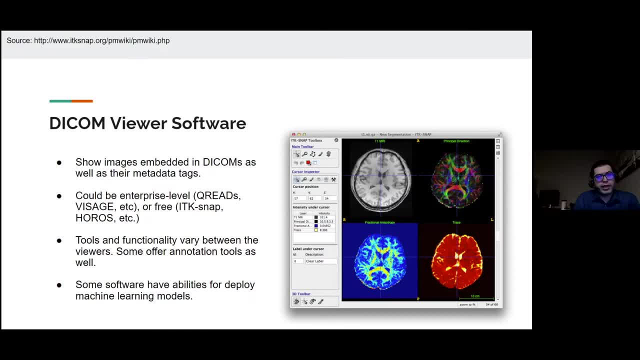 models to those software, And some of these software fortunately provide capabilities for that. So for example, at Mayo we have tools And some models are already deployed that year. so we do have tools that can, for example, receive an input CT scan and then, for example, segment. 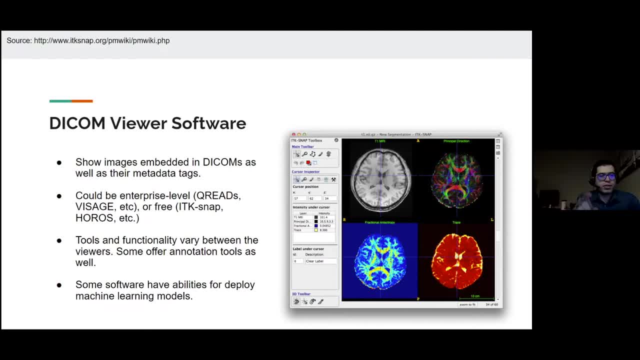 different organs in that CT scan for the radiologist, if that radiologist, when reviewing the packs, just pushes a button right. So this is going to be super easy if those models are actually implemented within these viewers. So this is the concept of the icon viewer software. 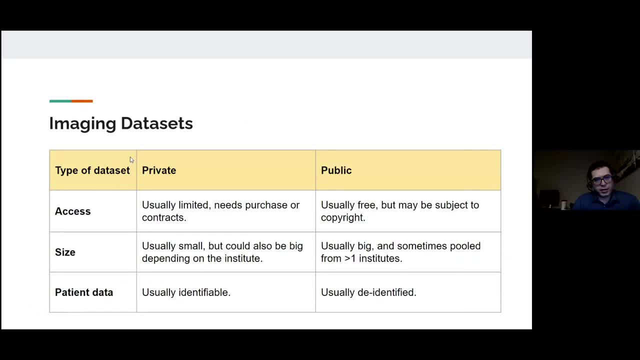 And now I'm going also to talk about imaging data sets, And this is again something that you need to if you are going to work with machine learning models, because you do need to collect some data, And data usually comes from imaging data sets. 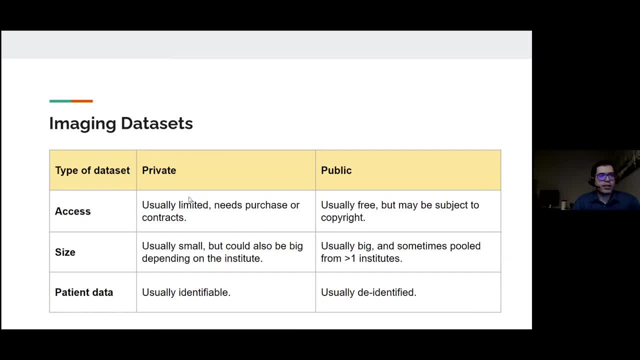 Now we do have two type of data sets here. right, We have private data sets and public data sets, And some things are different between these two kind of categories. Now, talking about access, private data sets say, for example, the medical imaging data. 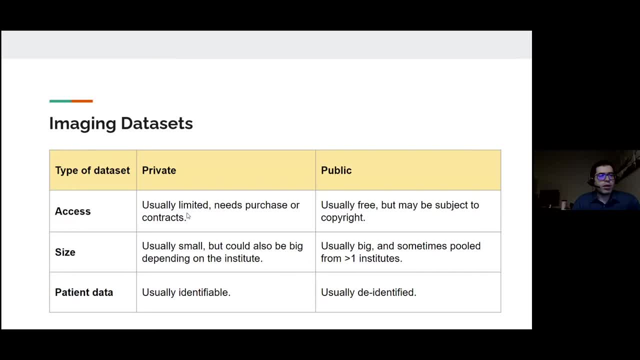 sets that we have available at Mayo. they are usually limited to people working at that specific institute right. So, for example, people out of Mayo not easily access our data, They need to purchase that or they need to sign contracts with us. 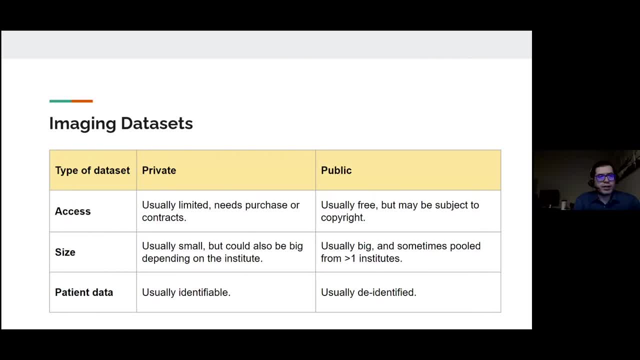 MOU with us and then maybe they will be provided with some sort of access. But when talking about public imaging data sets, you can almost always easily find access to them. You probably need to sign some sort of consents, but those consents are free. Everything usually can be done in a 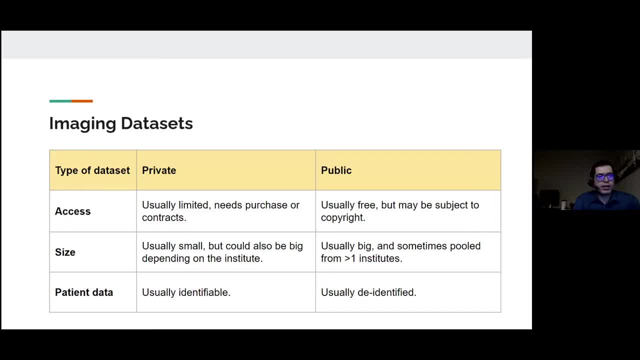 few minutes and then you will be provided the link to download that specific data set for yourself. Again, private data sets sometimes, or better to say usually, are small. Of course, it depends on the institute. If you are talking about an institute as big as Mayo, even the private 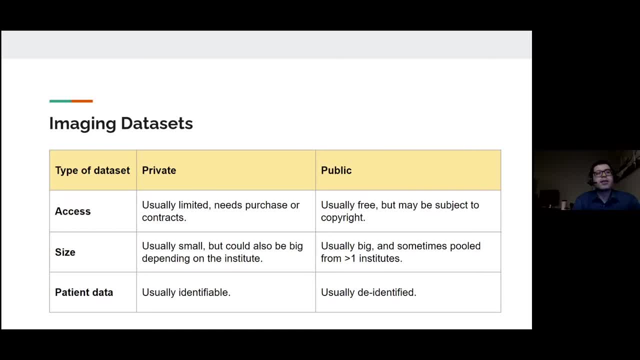 data sets are going to be much bigger than some of the public data sets out there. But for most of the institutes that are every size or smaller, private data sets might not be that much big, But public data sets they are usually big. The reason is that if you are publishing a 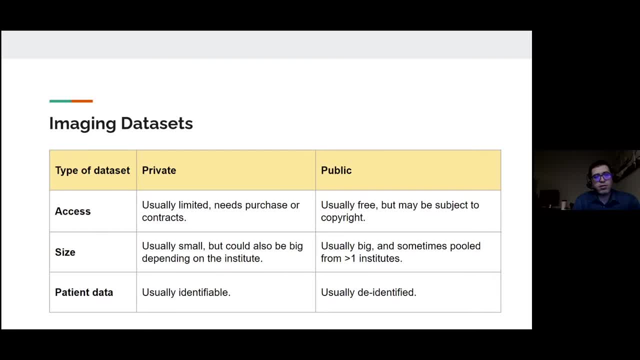 data set and if you want other people to pay attention to what you have released, you want it. But if you are publishing a data set and if you want other people to pay attention to what you have released, you want it to be big right. Because, no, there are definitely values in even releasing a small data set. 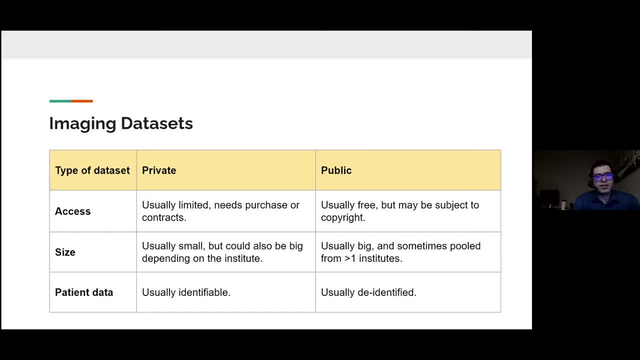 smaller data sets, but people usually tend to release bigger data sets containing images from a lot of patients and even sometimes from more than one institute. So some institutes sometimes come together, sign contracts and then release a pooled data set from images coming from different patients. right, And finally, the data coming from private data sets is 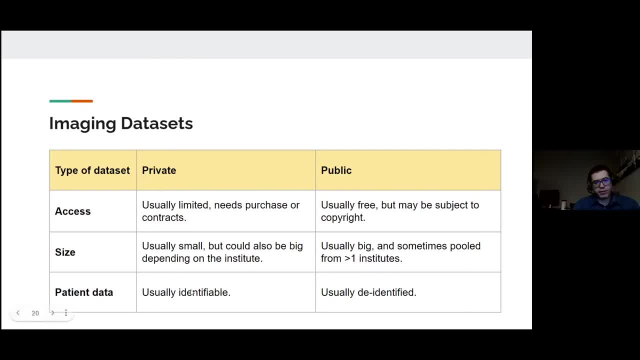 most of the time identifiable right, So these are not de-identified, So you probably need to be careful with that. As you remember, DIACOM files store a lot of patient information, patient data, So if you are working with that, either you need to be. 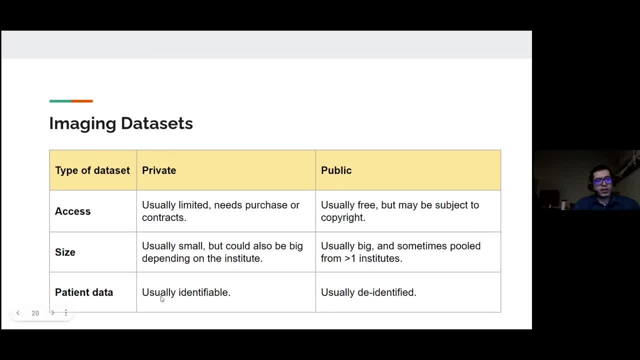 quite careful with. you know where you are putting those data sets, where you are uploading them, those data, that data should not be uploaded to anywhere out of the institute. Or if even you have the permission to do so, you need to de-identify the private data set first. So this is 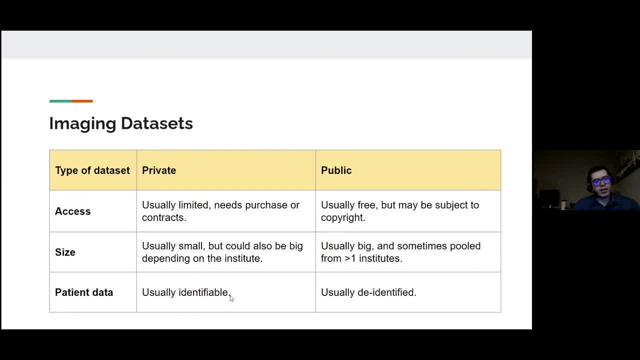 something quite important, And it's worth noting that even de-identifying some private data, that doesn't necessarily mean that you have the permission to share that with everybody else, right? So be careful about what you do with private data sets, But when talking about public data sets, 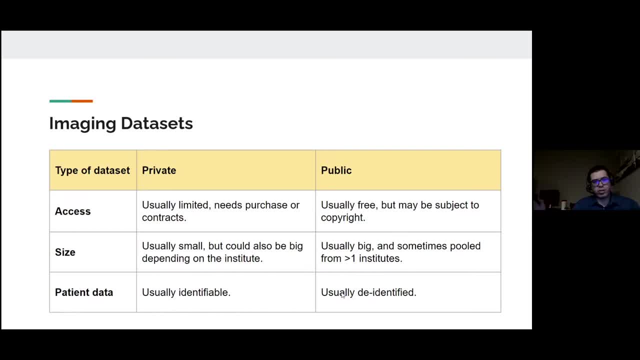 most of the time, almost all the time, they come de-identified, So usually you do not have to worry about the de-identification process, The very high quality data sets. they de-identify the DIACOMs directly And this is a better approach because if you de-identify the DIACOM, you are 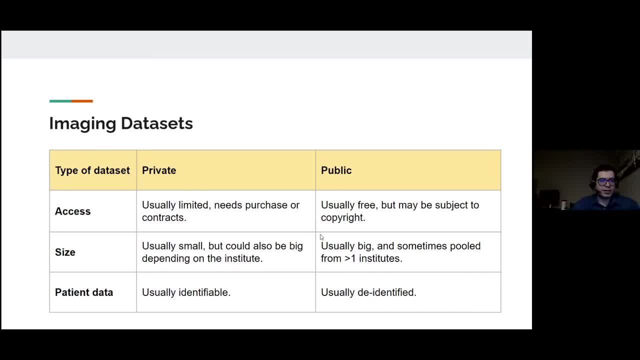 still going to provide DIACOMs to data scientists, which basically means that data scientists are going to have access to some of the data sets that are available to them, and they're going to have access to some of the data sets that are available to them, and they're going to have access to some of 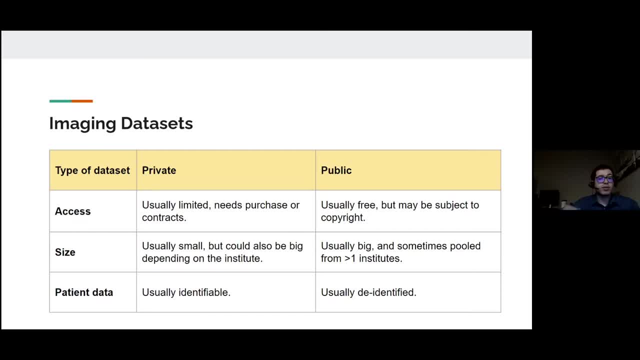 the data that were not considered sensitive but still could be useful for training models, For example, in the example that we talked about. if we are training, for example, a machine learning model on COVID-19 patient x-rays, it's good to have the age or sex of those. 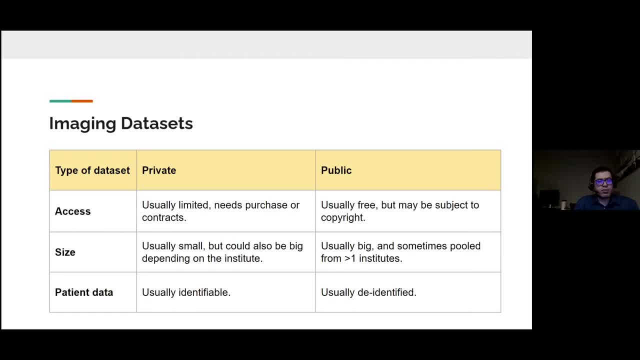 patients, And these are not something quite sensitive to usually blind, I mean to blind them. So if you de-identify your DIACOMs but still keep those two fields in the DIACOMs, then maybe data scientists could come up with more robust models. But 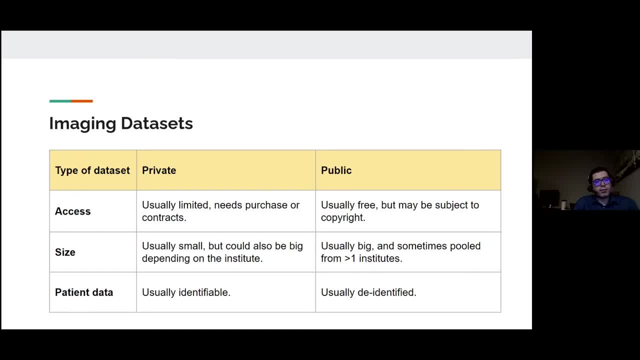 unfortunately, the more public, the more common approach is that if people want to de-identify the DIACOMs, they just simply get the imaging data out of that, which basically means that they will destroy the DIACOM and only give you the stored image in that DIACOM as a PNG image or as a JPEG. 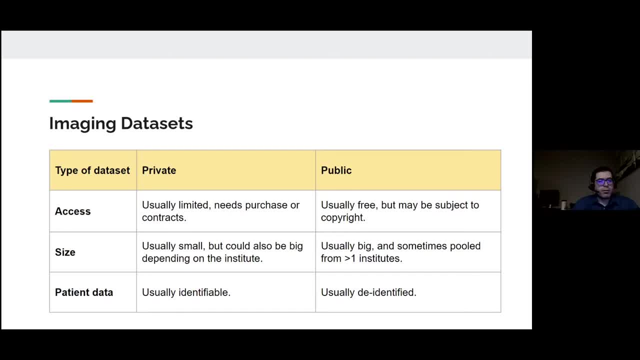 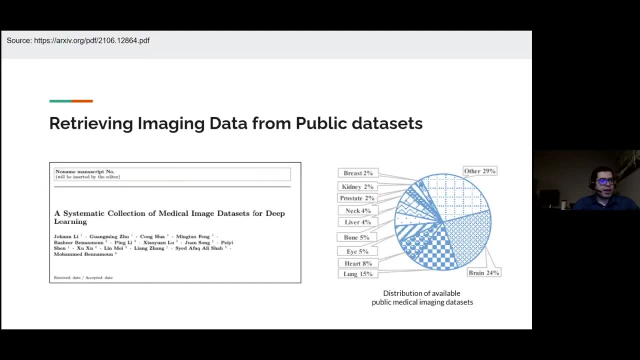 image, which basically means that you are not going to be able of accessing the other metadata in those DIACOMs- original DIACOMs, Now, talking about public data sets. I guess I also introduced this paper before, but it's worth mentioning again. We have a very nice paper here, a systemic 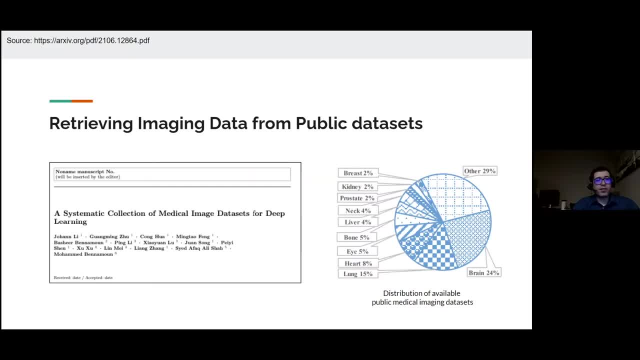 collection of medical image data sets for deep learning. This is not very recent, but it's still very useful. So whenever I care about a project, whenever I want to think about a project, almost the first step I do is that I go and check this paper and then I also Google that to understand. 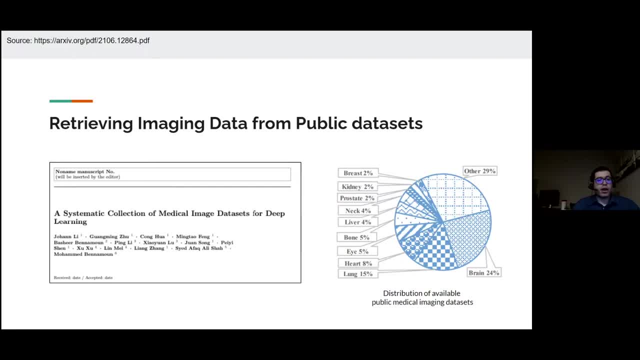 if there is any kind of public data sets already out there. Even though I might have access to very big private data sets, you know that it will never hurt expanding your data set and also give you some, you know, external kind of images to your data sets, because this is going to be. 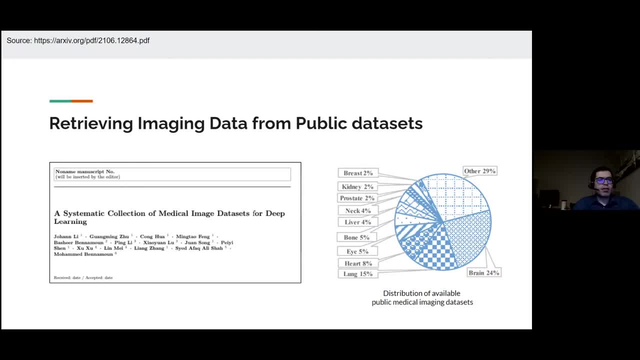 super useful both for training and also validating your model. So- and I have put a kind of interesting chart here. So at the time of publishing this paper you can see the distribution of available public medical imaging data sets. For example, two percentage of that belong to breast, If you look. 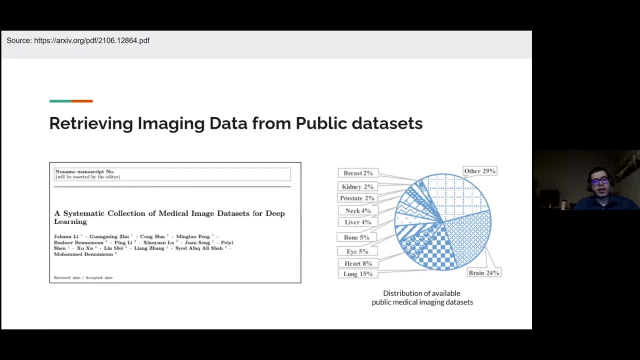 at that. the majority of the release data actually belongs to brain. So we have a lot of brain MRI, brain CT scans published publicly, but we do all. we do have, for example, five percentage of bone which we usually care about at ORTO and other things here, And lungs definitely, of course. I believe some of these. 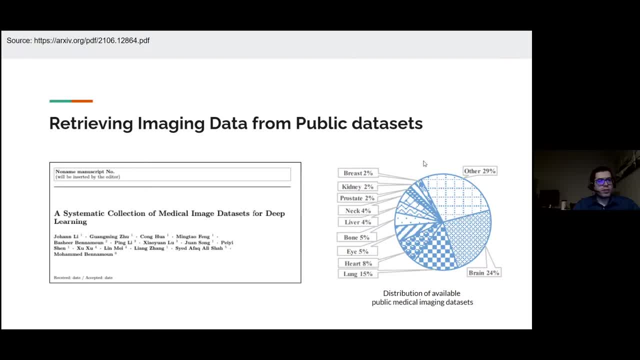 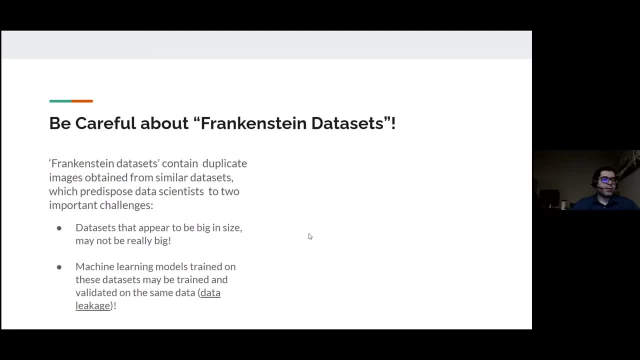 percentages are there thanks to COVID, But anyway, so it's good to take a look at this chart. Now I would like to talk about another concept that I learned its name from Dr Rickson once, and this is the problem of Frankenstein data sets, And this is something very fancy, Dr Rickson and 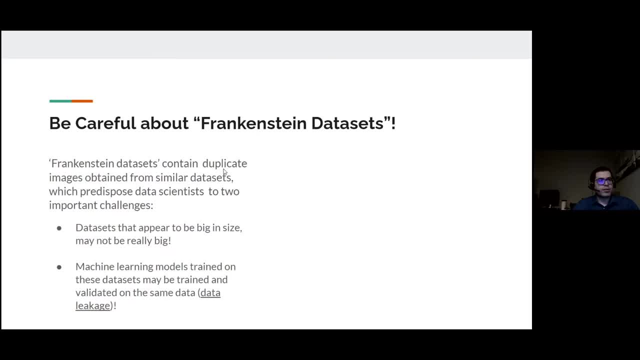 a few of us also talked about this in a review paper that we recently submitted to Radiology AI. talking about, you know that- the best practice of data handling for machine learning projects. This is something that actually happened to a lot of COVID publications in less than a year ago. 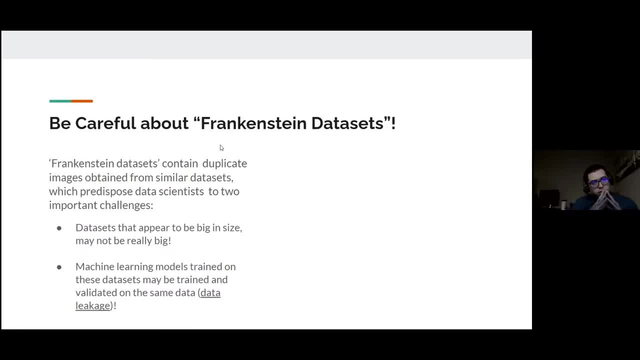 right. The problem is that. so you probably remember from our previous two workshops that whenever we want to go through machine learning training, we want to separate or split our data to some falls that are, or to some sets that are clearly separate from each other, And by this I mean that no patient overlap should be between. 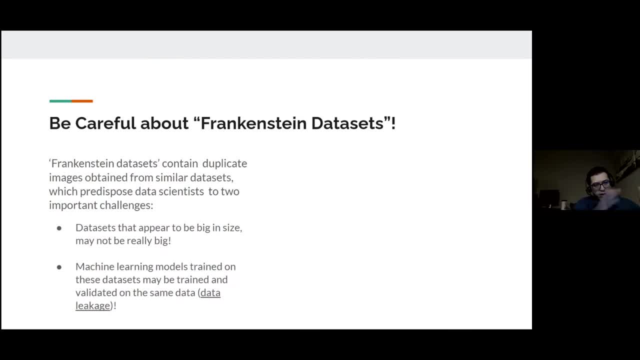 those sets. If I'm going to train my model on a fraction of data I have and then validate that on a separate fraction of my data, we do want these two fractions to have nothing in common, And the best practice in medical work is that we usually provide separate patient ideas to 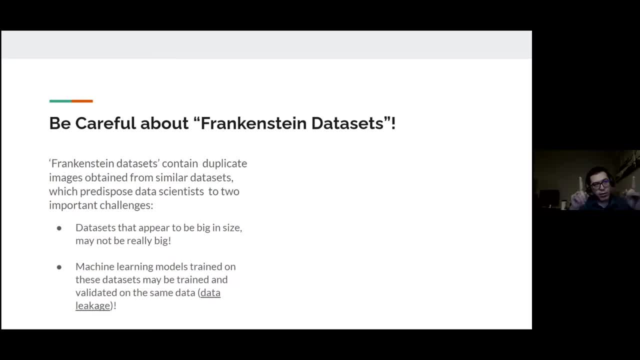 these two sets, So there is no patient overlap there Now. at the time that COVID happened, everybody was craving for data. They wanted big and big data sets right, And some data scientists did a good job there and released their data- Even some individual patients. 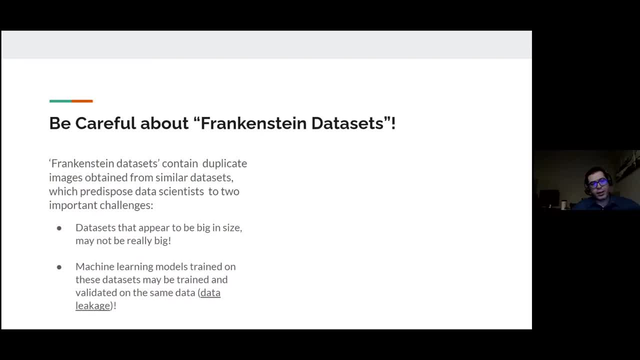 some individual data scientists released data on their GitHub pages. Now, the problem that happened was that some of the people who were there- and they, you know, maybe intentionally or unintentionally- they said that you know, I am going to release the biggest data set ever. 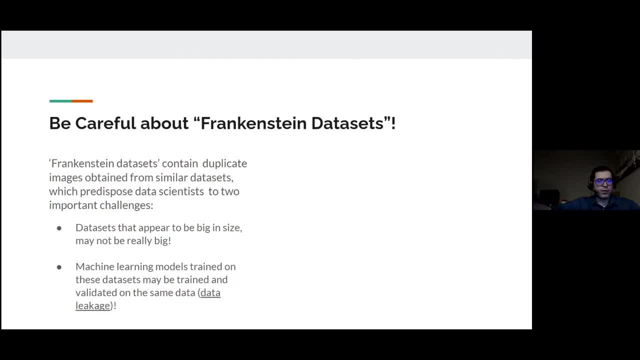 And what they did was that they downloaded the data from whatever other repositories or data sets that are already available in the internet, And then they renamed the files, deleted some images from their own and reuploaded the entire data set And, of course, the uploaded 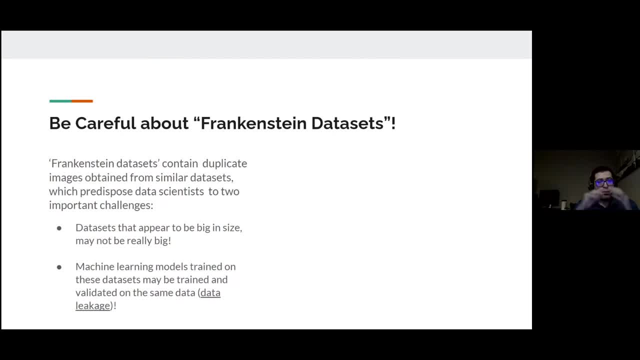 data set could be bigger than whatever else that could be there, But I, as a data scientist, could have gone there and say that, oh, this is data set X, which was older, and this is data set Y, which has been recently published and includes a lot of images. 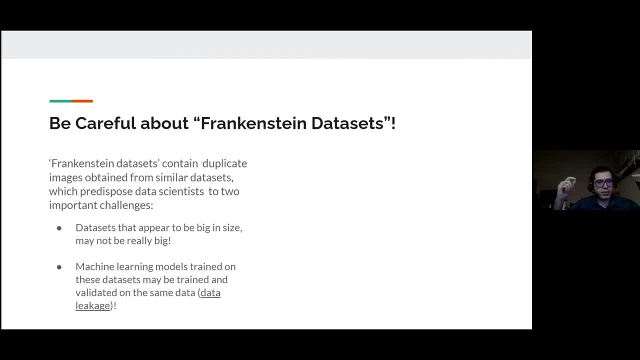 So let's get both of them, And I will make this assumption that the patients between these two data sets are quite separate from each other. I'm going to, for example, train my model on one of those and then validate that in another one And, to be honest, what will happen is that, if that Y 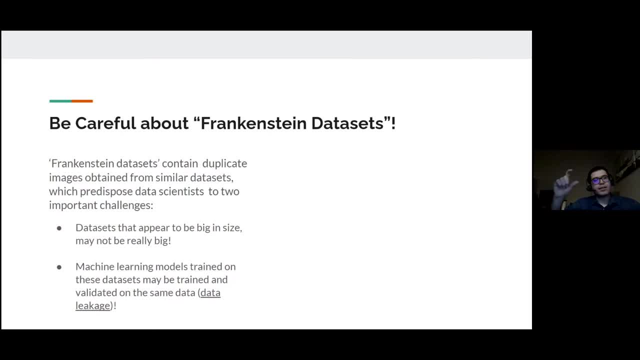 data set Y big data set had been made of some of these patients that had already been in the X data set, then my split is going to be a mess And this happened to me personally. that Erickson probably remembers that on those times that we didn't have too many COVID cases at Mayo, we were doing our 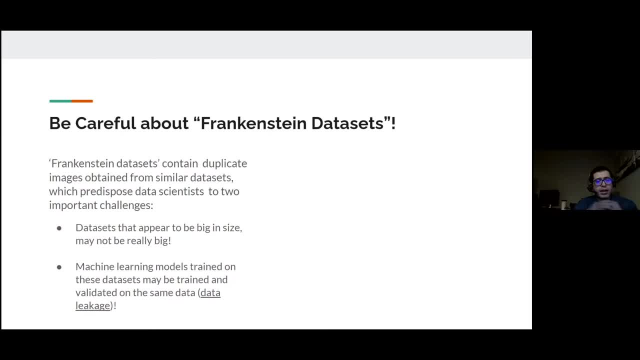 best to go through some of these public data sets and train a model, And I had a model that actually looked to work quite nicely On my training and validation set and that was quite interesting. we had scores that were close to 99% of accuracy for detecting COVID or distinguishing that from other pneumonias. 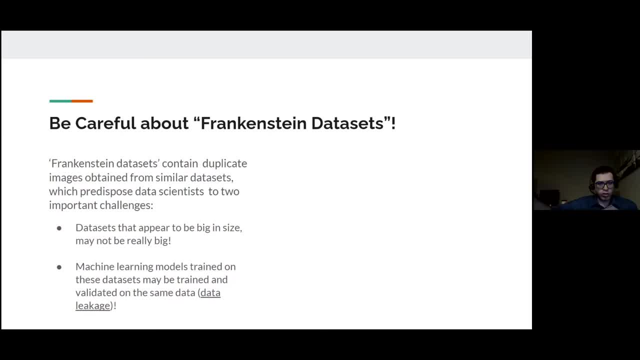 But when we got some Mayo data that we were sure that those were not included in my data, in my original data, training data. my model was doing a very poor job there And we were quite confused. We didn't know what has happened until the time that we came out. 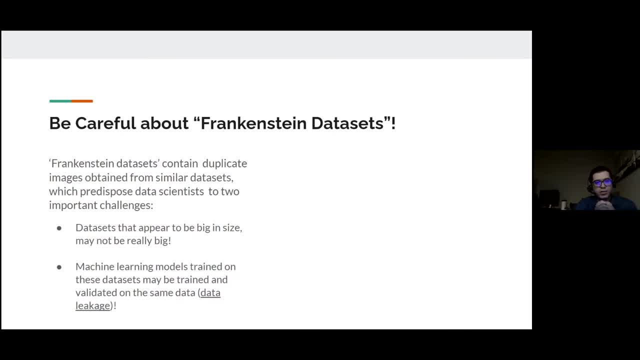 to this problem And we realized that, oh, some of the training data sets that we used had actually some images in common with each other. So be super careful with Frankenstein data sets. Basically, you need to clearly know what patients have been. I mean what patient data have. 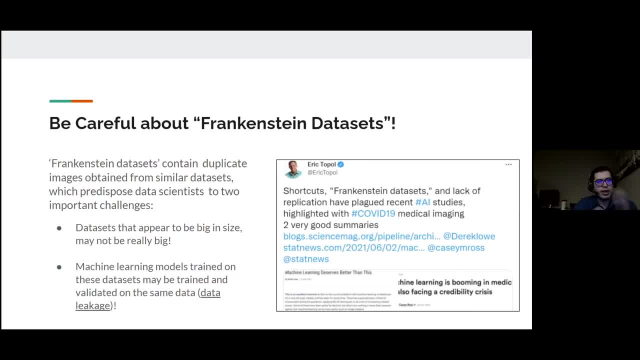 been used for the public data set that you're interested in, And this is something that, a few months ago, a lot of people talked about accusing these data scientists that published paper after paper saying that our COVID-19 models achieved accuracy of 99.9999.. You say well, believe me. 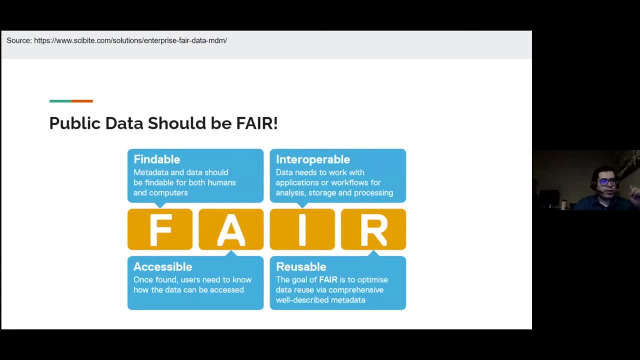 this is probably something wrong right Now. again, I would like to remind you of the concept of fair public data should be findable, interoperable, accessible and reusable, And this probably now makes more sense to you talking about Frankenstein data sets. 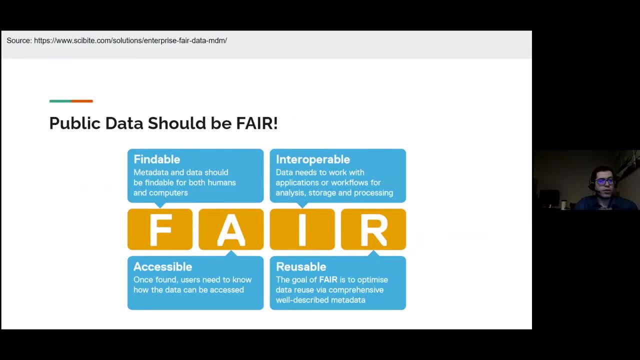 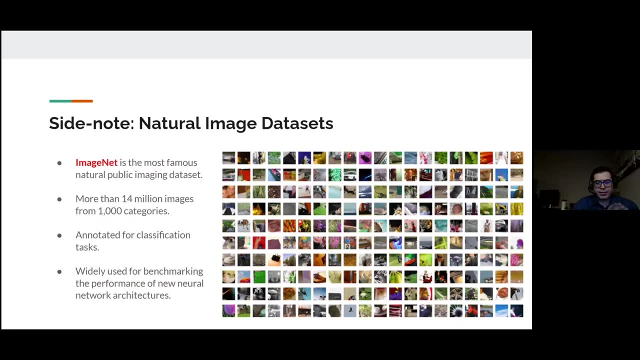 so be careful about working with public data that is fair, And if you are yourself thinking of releasing some data, release it in a fair manner. Now, I believe this is the last slide for this aim, So I'm going to talk about some sort of natural image data sets as well. We are in the 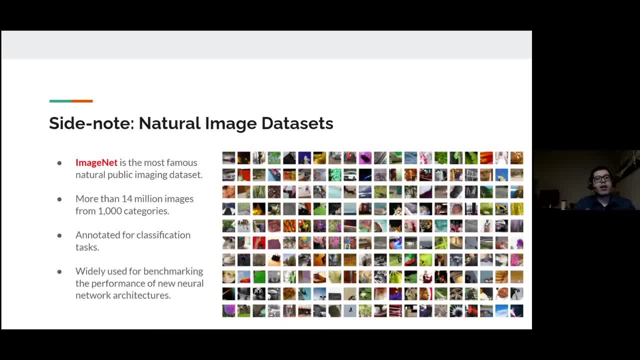 world of medicine and we do care about medical imaging data sets, and there are many medical imaging data sets already published. but it is worth noting that in real computer vision world- non-medical computer vision world- people usually talk about a lot of natural image data sets as 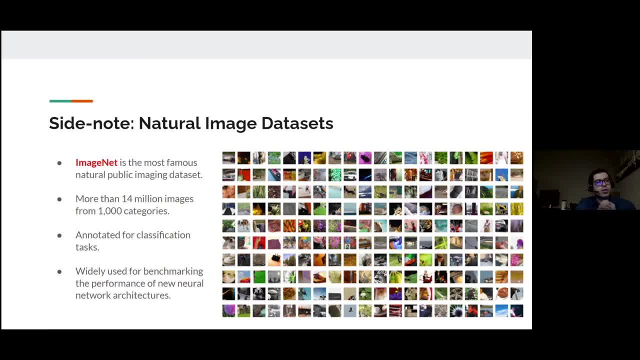 well, And the most famous one is this image that I have put for you here. This is actually the most famous, the most basic and the most, I believe, the new version of that- even the biggest data set that we have, the biggest public data set that we have in the field of computer vision. 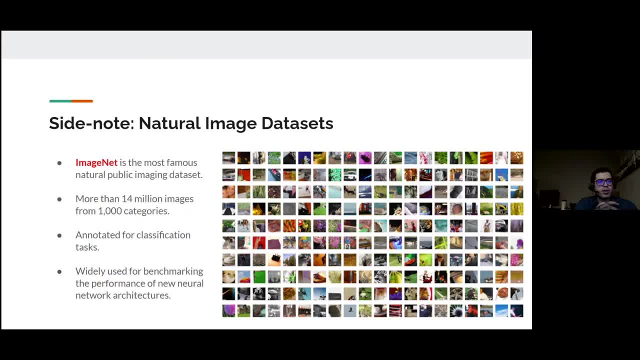 It consists of 14 million images from 1,000 different categories. I believe the new version of that also has 22,000 categories. but you know, the images are like the ones that you see here. Those are not medical, Those are images of people, cars, you know, plants, things like that, And 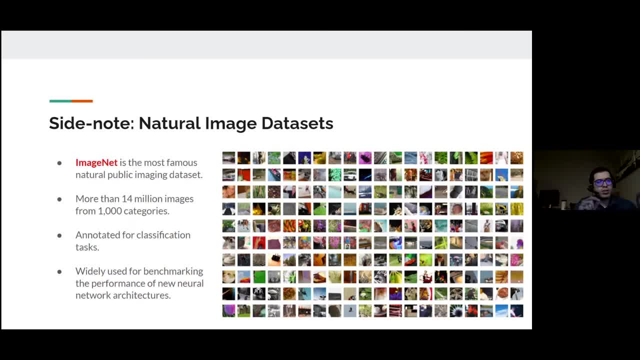 this data set is quite important because it is used for benchmarking the performance of new neural network architectures. What that means is that if I'm a data scientist and I came up with a new neural network that I believe is going to be the site of the. 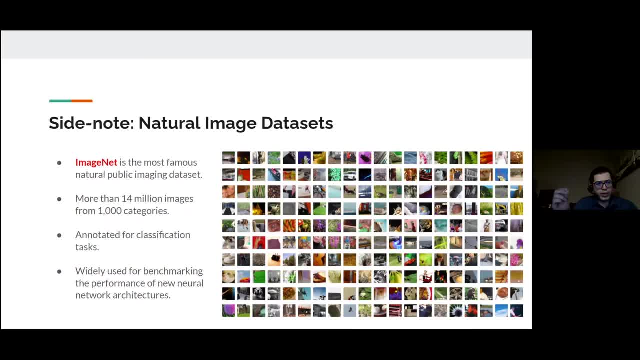 art better than whatever else. I am going to prove that by applying, by training, my new model on the publicly available ImageNet data set and then release the performance metrics for that right, And then these performance metrics could be used, could be compared with other training. 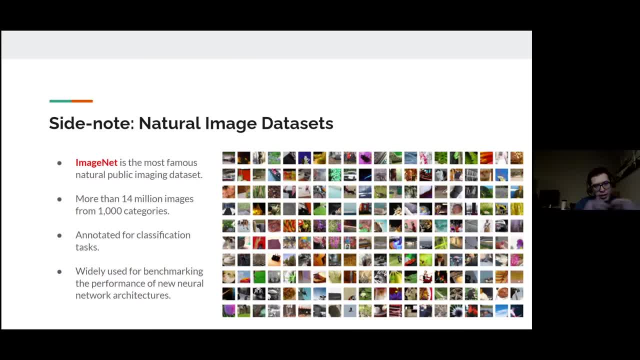 pipelines, other neural networks that have already been there. So this is a kind of a baseline benchmarking routine. if any data scientists come up with some new models or new training techniques, whatever right. So it's good to know that. So I'm going to go ahead and show you the results. 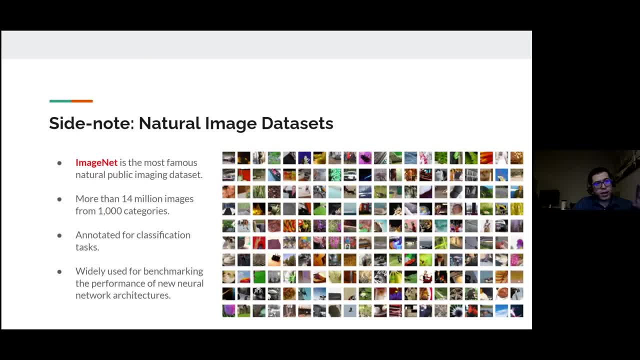 And another thing that I would like to talk about this later, but I would like to briefly mention here, is that this natural image data set of ImageNet is also going to be useful for us as data scientists who work on medical imaging, because of the transfer learning- Now that term. 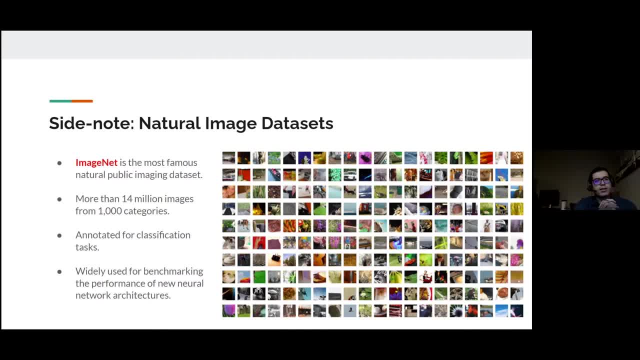 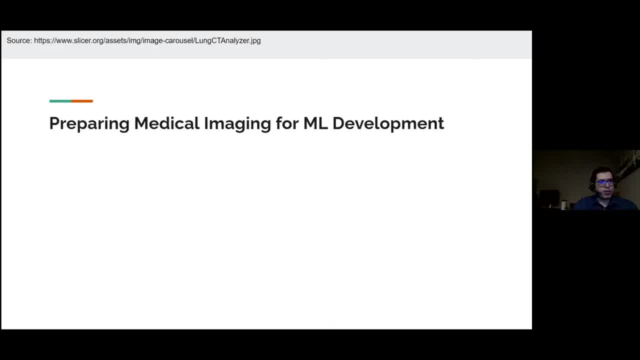 transfer learning you probably already know about, but if not, keep that in your mind. I'm going to talk about that in third part of this presentation. Now pre-pre-medical imaging for ML development. seems that I lied and that was not my last slide for this part, but 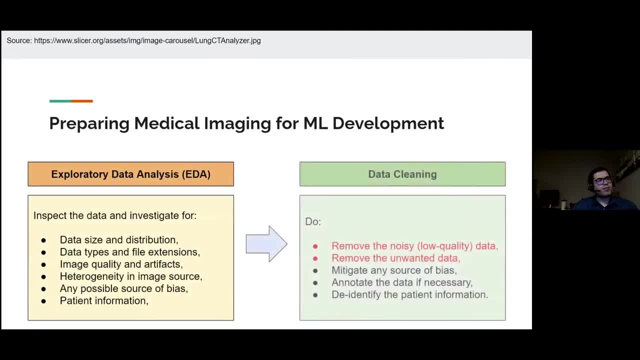 it's probably one of the last. So whenever we are going to prepare medical imaging data for ML development, we are going to go through two main processes. The first one is called data analysis or, if you want the technical term, it's usually called the exploratory data analysis People. 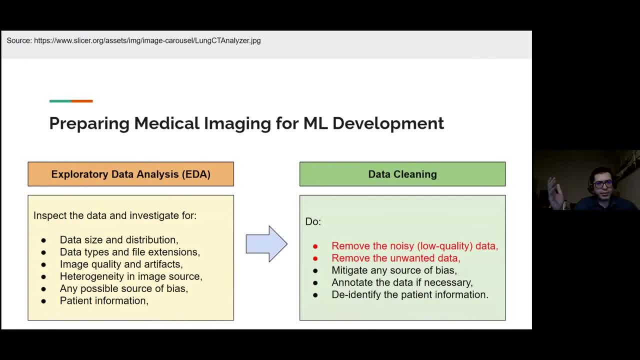 data scientists usually call it EDA. EDA basically means that to look at your data and try to interpret that as much as you can right, Try to understand- you have to realize the data size and the data distribution If your data has has come from. 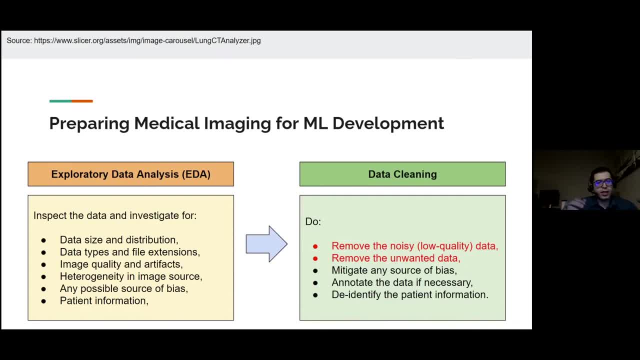 multiple institutes or multiple cohorts of patients. try to understand how many- how many patients from each cohort exist in your data. Or you know if they have different attributes. try to visualize those attributes. try to look at the data types and file extensions. 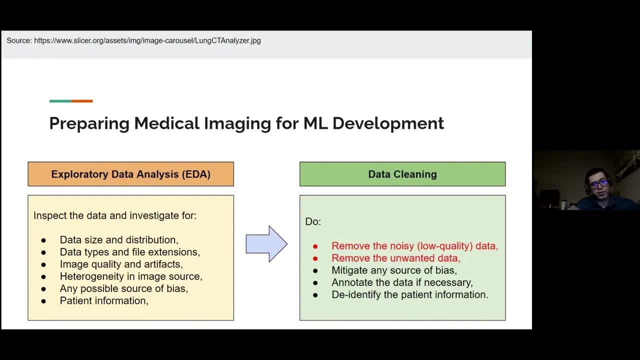 Are all your files in DICOM format, or are some of them in JPEG format, or do you have both of those types available to you? What are the image qualities? Visualize the data by yourself. Of course, if the data set is too big, you cannot visualize each individual image, but pay attention. 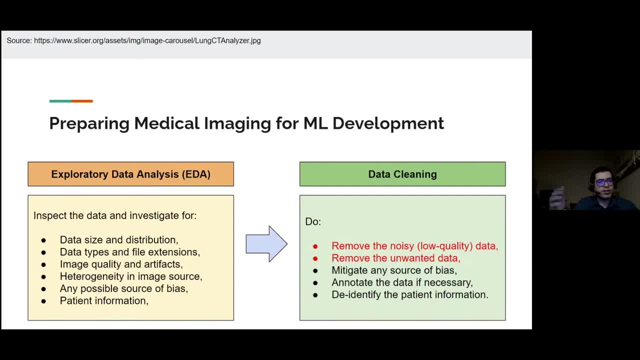 to random subset data. If you have a data set that is too big, you cannot visualize each individual image. but pay attention to random subset data of your image data set and you know, understand the quality and artifact. You know, do you have? 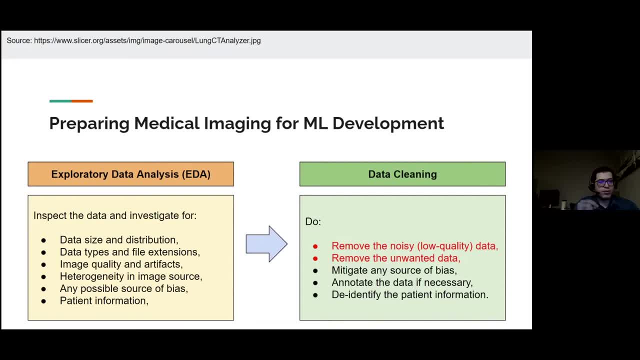 do those images look to you as they should have looked when you first started the project, Or do you have some noise there, some artifacts that you need to remove? What is happening in your data right? Heterogeneity in image source is also another thing that you need to consider, And 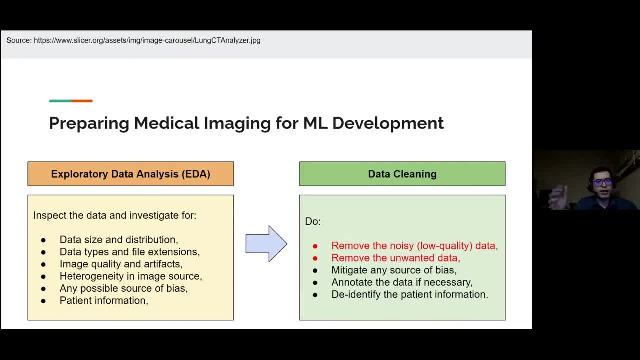 any source of bias. you know this. this is not something that I can provide you with a specific list of items. You need to look at your data and then keep asking yourself questions and questions about what could go wrong with these data. if I train a model on that And then, probably at the end of an EDA, you have some notion of. 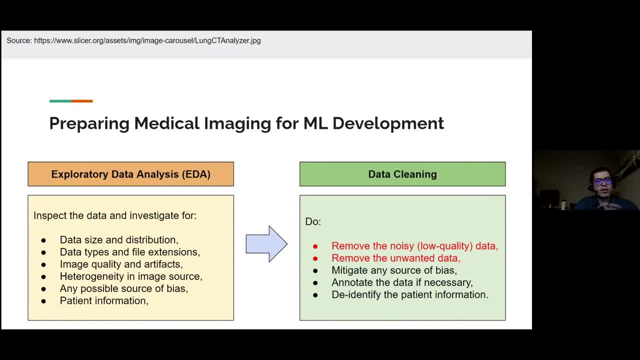 how to clean your data or what kind of noise data to get rid of, And this basically brings you to the next phase. that is called data cleaning. And data cleaning, as we all know, is actually to get rid of the noisy, low quality data or remove the unwanted data. Maybe the data is not low quality. 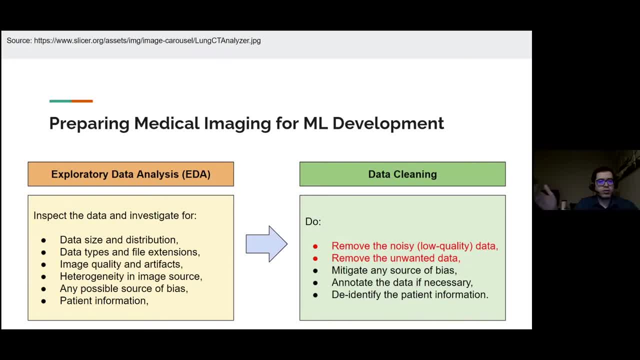 or noisy, but you really do not care about that, right? You don't want it. You know that. you are sure that if you keep that data, you are just going to make your model more confused. So let's get rid of that data. 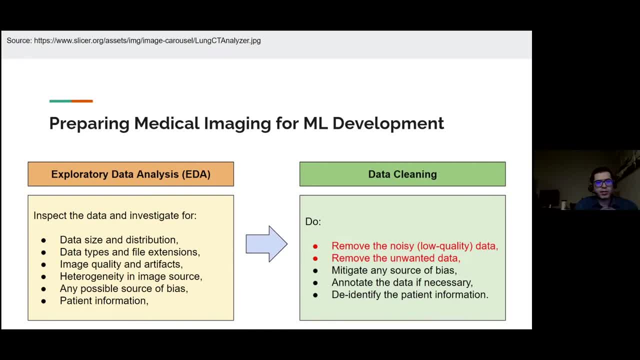 And you know, some people consider annotations separate from data cleaning. Some say that annotation should also happen during the data cleaning. Otherwise, data annotation is something that you need to do after you clean your data right. So this this is important to keep in mind. 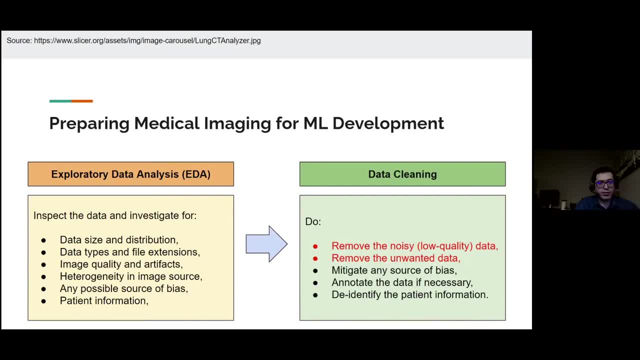 So never, ever, annotate an unclean data set, because you might spend a lot of time on annotation and then realize that part of your annotations are going to be useless because the original images need to be removed during data cleaning And annotating medical imaging data for ML. 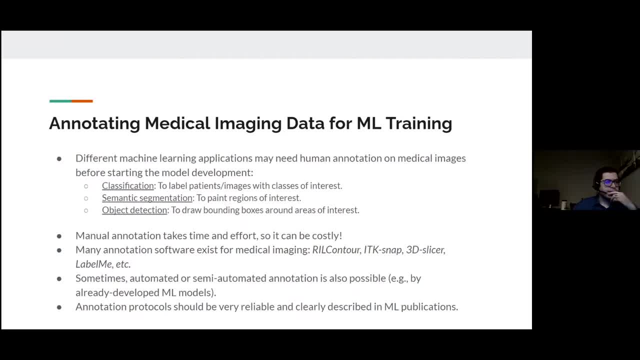 data cleaning you already. we already talked about that, So I just put this slide here as kind of a review. I told you that it takes time and effort. Some software exists for that. Again, the names are here for you. if you want to think about downloading those RealCountry ITK Snap 3DSlicer, they are the 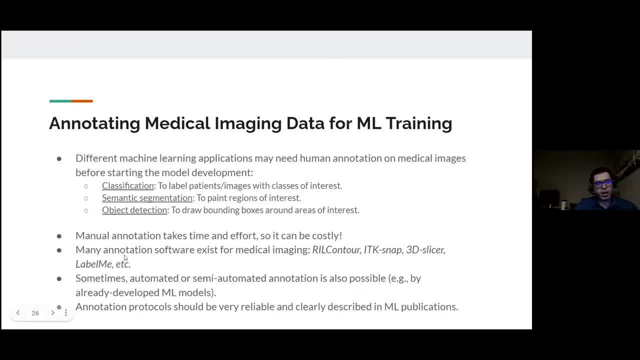 free ones. Labelme is actually specifically for annotating object detection, those red boxes, if you remember. So this is actually one of the software that I like because it usually takes a lot of time. I mean much less time than me than, for example, the other ones here that are for segmentation. 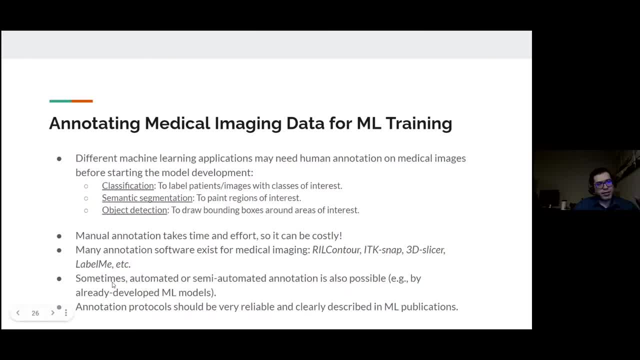 All right. so one point here is that sometimes automated or semi-automated annotation is also possible. So if you have a very hard job annotating something, it's worth consulting someone who has experience with data science to understand if there are ways to semi-automate at least your. 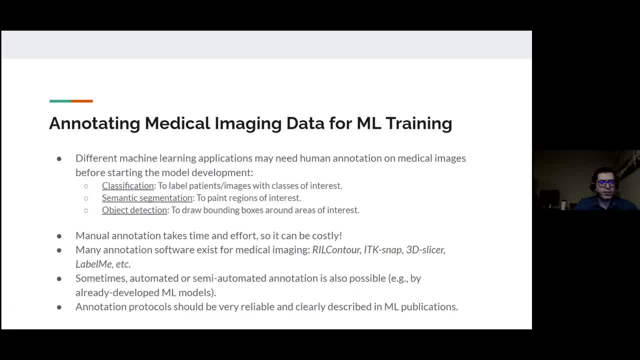 annotation pipeline, which basically means that we are going to use some sort of already trained machine learning models to help you with annotation. Those machine learning models might not do a very accurate job, and this is the reason that we expect to need you as the annotator, but those might make your work, make your building less. So it's good to. 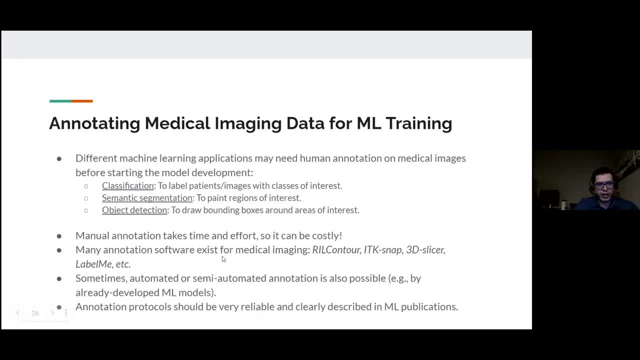 have this point in mind that sometimes machine learning could also be useful for the annotation itself. And again, I'm not sure if I wrote this here or not, but sometimes those public imaging data sets that we talked about- they also really release annotations, right? So, for example, they 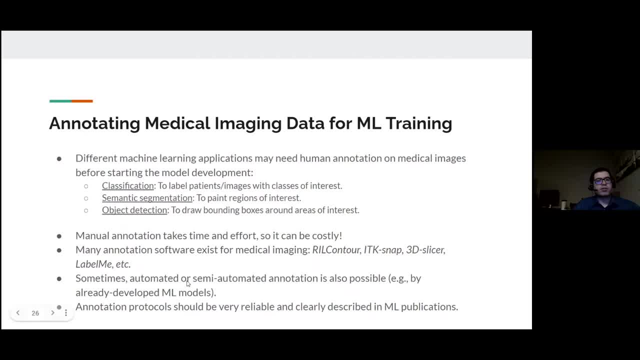 might release classification annotations, segmentation annotations. so almost always you should look for public data first. If you have some public data available, then good for you. you probably are going to have less time spent on annotation by yourself. And this is the final slide of this. 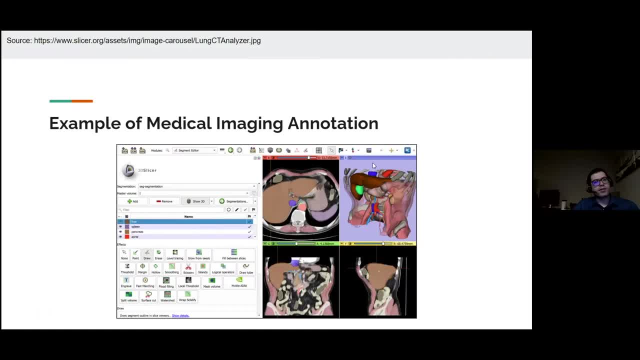 point. This is an example of a medical imaging annotation software. Now, I believe that was, I guess, 3D slicer. So you just feed in your images here and then it provides you with all these nice tools for painting your images, as this is for segmentation. You see here some people. 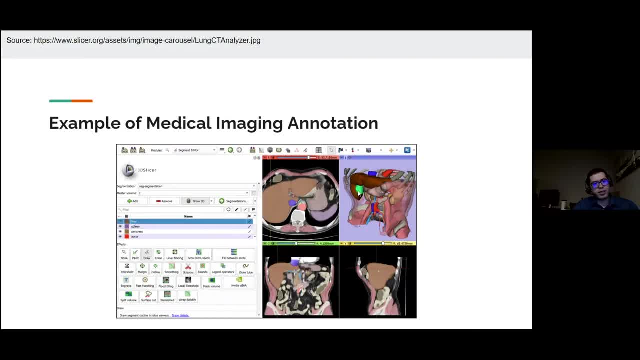 have gone through a 3D volume here. try to segment each organ and you can imagine how much time this this probably has taken from them. But you know, if you fit this to a machine learning model and train that decently, then you probably have a model that can segment all organs this much. 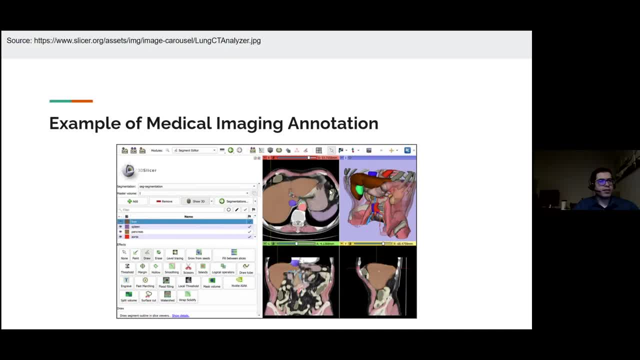 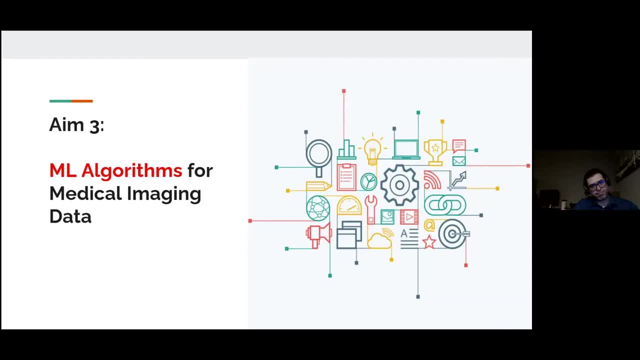 beautifully for you. So annotation almost always pays off at the end of the day. Perfect. Now we are at the end of checkpoint two. So again I would like to pause, see if anybody has questions or comments, Maybe because I have to leave at 2 pm. maybe I'll leave at 2 pm. 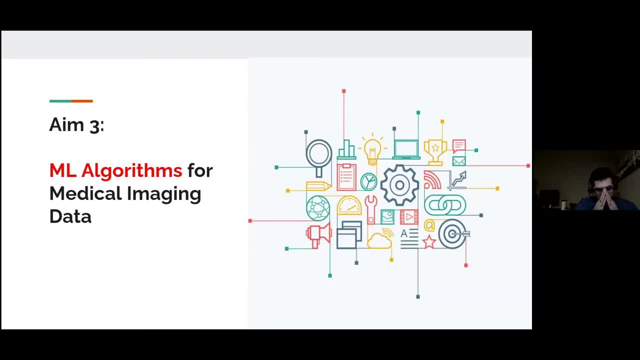 I asked a question, Sure, The question about the computer vision. the first part, and I was just thinking, you know, in the practice right now, is you know, in the osseptic field, for example, you have a tumor, or let's say, you have a spine problem. So you, 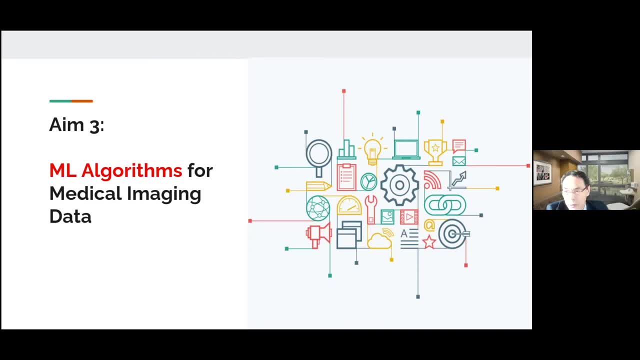 let the patient take a CT or MRI, get the imaging right, Yeah, And then the radiologist would look at the information you provided by the physician and then, based on the imaging, they make a suggested diagnosis and the back to physician. 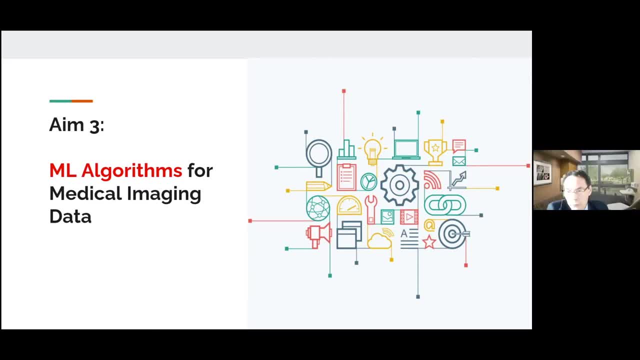 Yes. So we always kind of caution for the physician is: the imaging is not like. let's say this way, the imaging data is not. you cannot diagnose some problem to the purely based on the imaging analysis. for example, make the a good example. the spot. 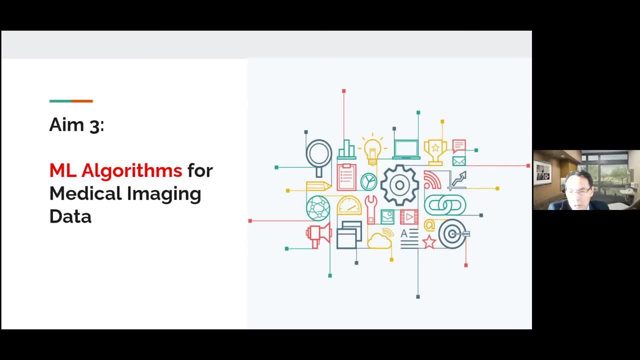 you know a lot of spine disorders, degeneration, diagnosis. you know some patient very worse, very bad imaging. but they combine the clinical symptom or the checking. they cannot establish a diagnosis based on the imaging. so my question is for this: ai or machine machine learning or deep learning? 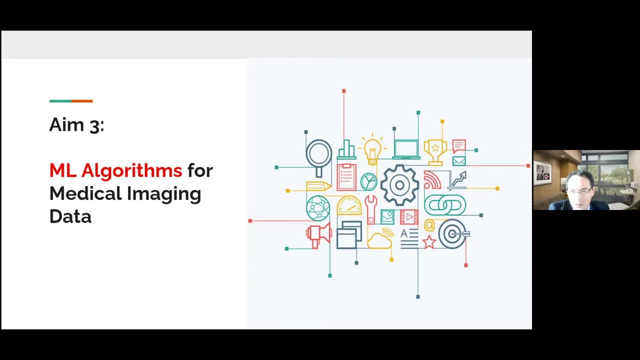 how they can change the practice with this, with the physician, physician, the, whatever the clinical symptom involved, even you know, imaging by this machine learning show. okay, this is the show. the mylarpathy, for example, that's kind of worse, the span problem, and then back to 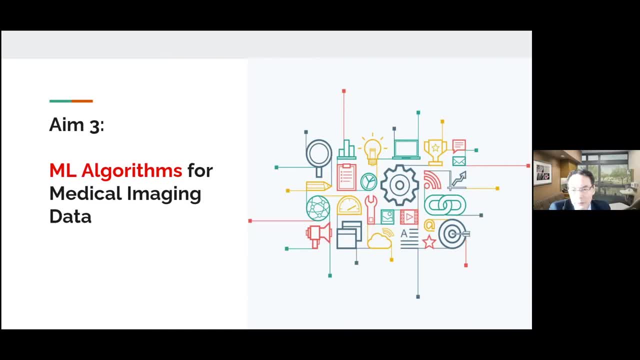 physician. okay, the patient doesn't have any nerve problem. so my block- they cannot be established- is that the ai can have for this yep. so thank you for your question. this is quite an interesting one and maybe something that a more experienced researcher and data scientist like that can provide. 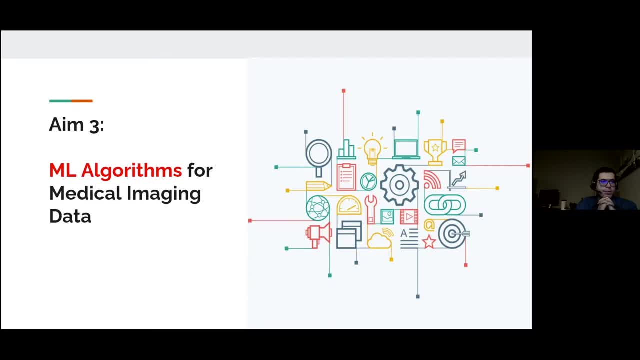 better answers than me, but in my humble eyes, uh, the answer to your question is that it is possible doing that using machine learning and, to be honest, this is something that we all aim for whenever we train models using machine learning. we do not want to have tools that are only fancy. 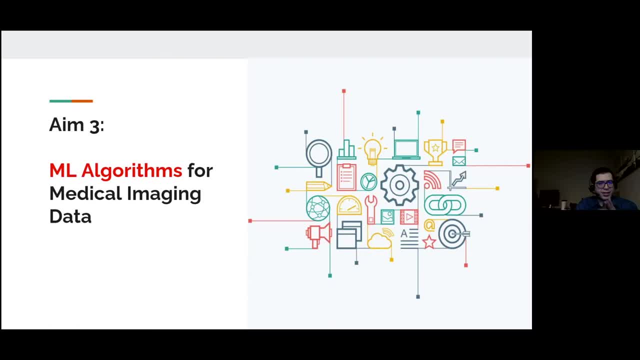 enough to be, you know, to maneuver on in presentations and then in real practice. we cannot rely on those. but uh, training those kind of models that we can really trust in real clinical practice, especially for those kind of hard examples you mentioned, is something that takes a lot of time and iteration. so 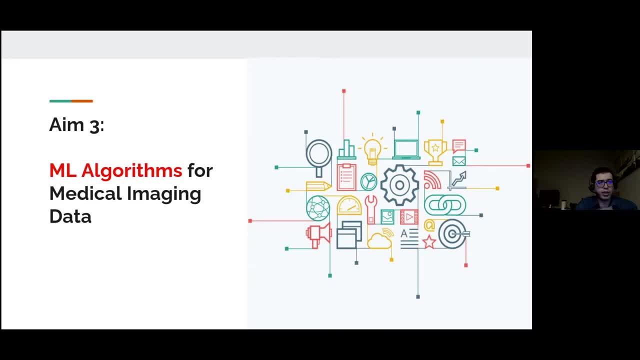 fortunately, we have good examples of those already available and, to be honest, uh, i believe uh in our own labs, both in dr rickson's lab and in dr kramer's lab, we actually uh published a lot of those. so, for example, uh one of the one of the most recent papers that i can uh, you know, uh tell, 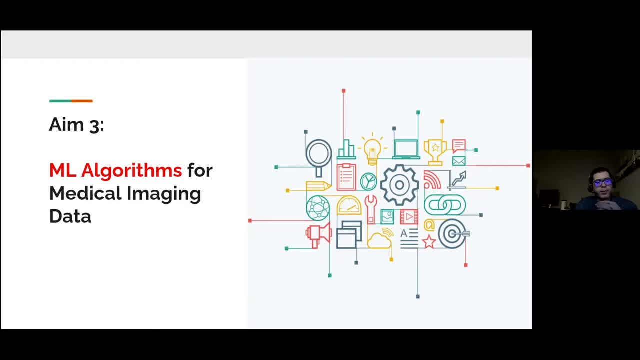 you as an example that we recently submitted to radiology ai uh is from my colleague, dr khosravi, who basically he designed a risk calculator for patients that went that are going through total arthroplasty and that risk calculator is meant to tell the operating surgeon what risk 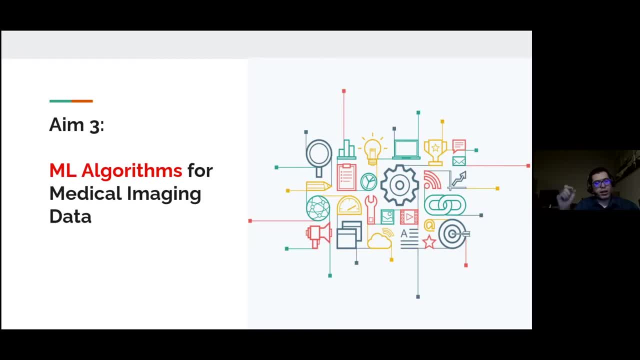 that patient is going to have for this location or, you know, the implant dislocation- i mean sorry- depending on some of the, you know, unchangeable attributes of the patient, like their age, like their sex or even their pre-operative x-ray, and also some of the decisions. 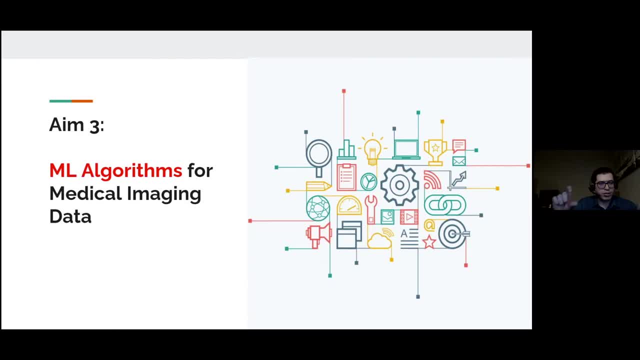 that the surgeon is going to make, like the type of implant is going to he or she is going to use, right, which includes things such as l? ab and blood fe, creative baby CT or his abortion or things like that. so the final, the final application or the final software is actually a very nice graphical. 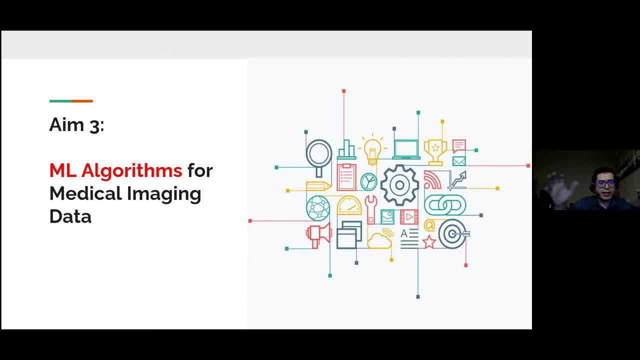 interface that a surgeon should upload a single preoperative lightweight x-ray of the patient too, and then entire, for example the age, the sex and things like that, and then the model is going to make some sort of calculations and then finally it is going to provide some sort of risk estimation. 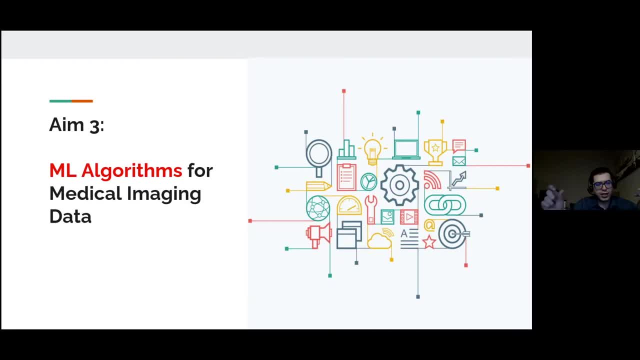 to the that, for example, if you want to operate on this patient using this primaissances model specific implant, they are going to have this much of this, this amount of risk for dislocation and defense right, Something like that. So this is, this is an example of a model that hopefully 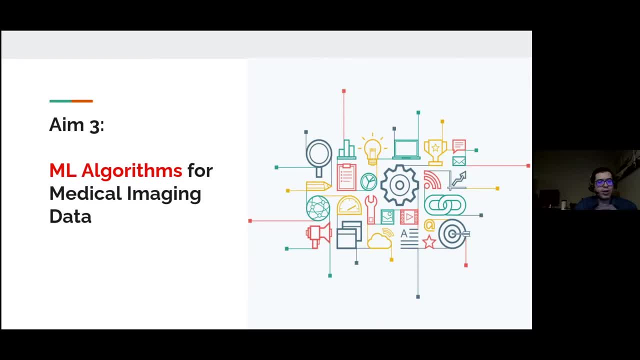 could be put into practice. finally, if- and this probably is going to help a lot to individualize this medicine, right, Because you now can adjust your decisions as a physician based on some features or some, you know, clinical attributes of your patient that you might not already be aware- 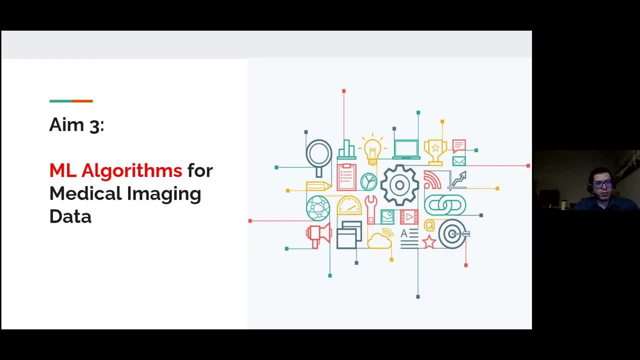 of. And this is what machine learning model actually cared about. because in that specific example I told you, Barrios model actually relied a lot on that single pelvis image that the physician provided to the model. And it is quite interesting because we have a lot of publications. 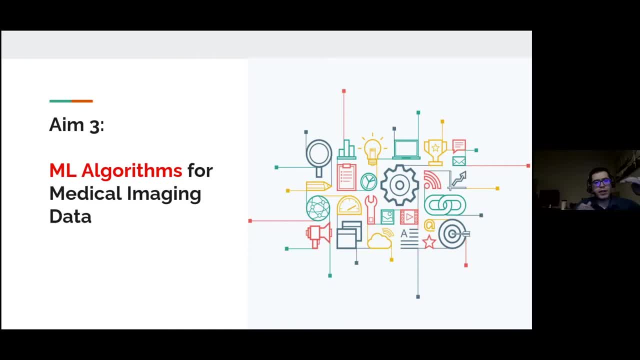 on 20 or 30 clinical variables, saying that you know we can predict the risk of dislocation. looking at these clinical variables that are, all you know, beautifully described in Excel spreadsheets. But what Barrios showed in his work was that a single pelvis. 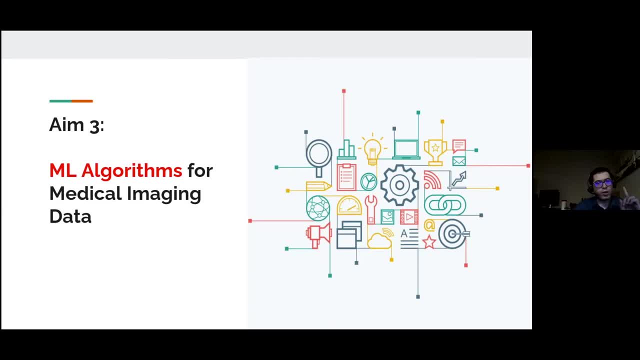 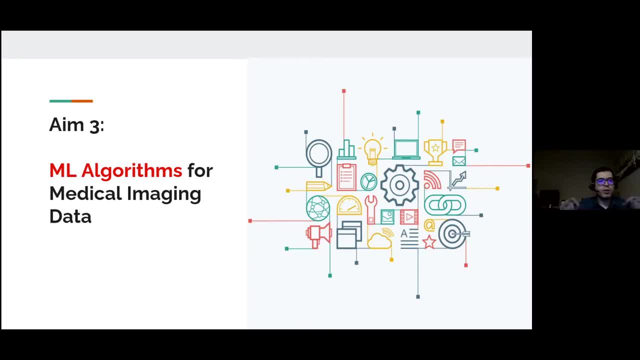 We are not going to lose any data. We are not going to focus on or, you know, be biased towards any modality, But I want to say that sometimes, if carefully engineered, these machine learning models could be as accurate as you described them or be used for real practice. 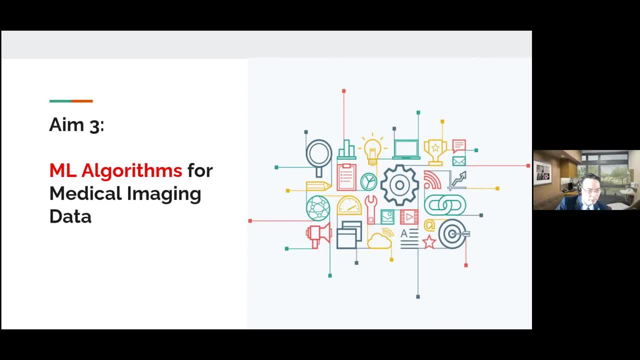 Thanks, Great, great talk, Yeah, thank you. Any other questions or comments? Perfect. So now I'm going to talk about machine learning algorithms for medical imaging data, And this is where things get a little bit more technical. So I try to present more slowly and also pause more often to give you time to ask your questions. 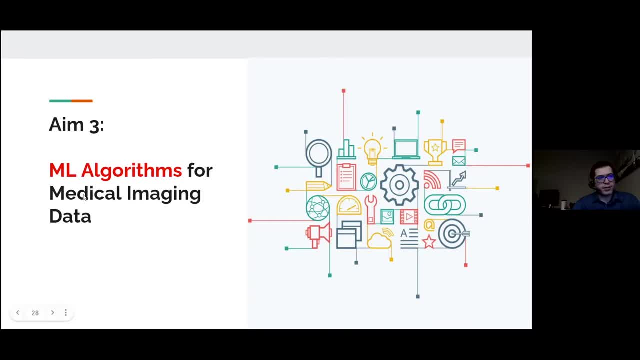 And then also I'm going to do a lot of recaps, right? So the first seven or eight slides of this part is going to be recaps of our two previous workshops, because I believe this is something that you might- not, you might need to know about before we talk about convolutions, right? 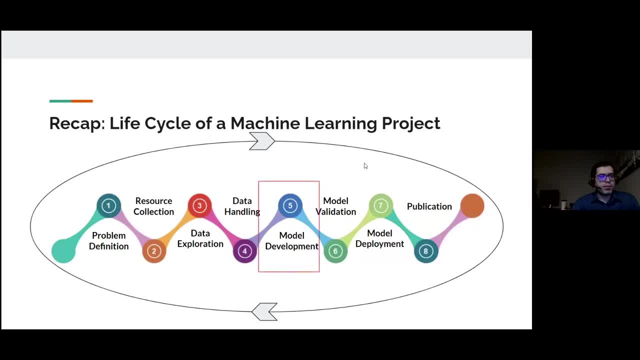 So let's start by reviewing this big picture chart first. So we are going to talk about model development. This entire part three is regarding is about model development. We might also talk about model validation- some of the recaps- but convolutional neural networks are actually a kind of architecture that we care about when we are developing our models. 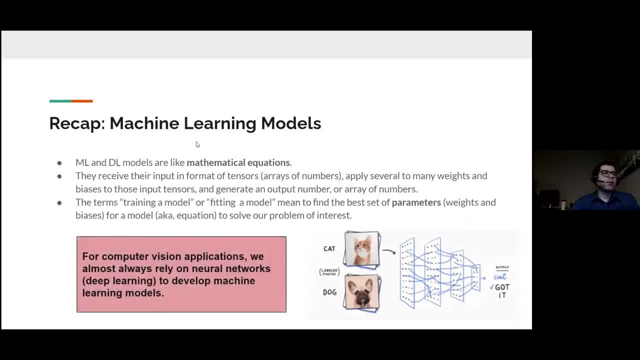 Now let's start with machine learning models in general. So you probably remember that we first introduced machine learning models and specifically deep learning models, as some mathematical equations right, Which I told you that you know whenever you talk about deep learning models or neural network. 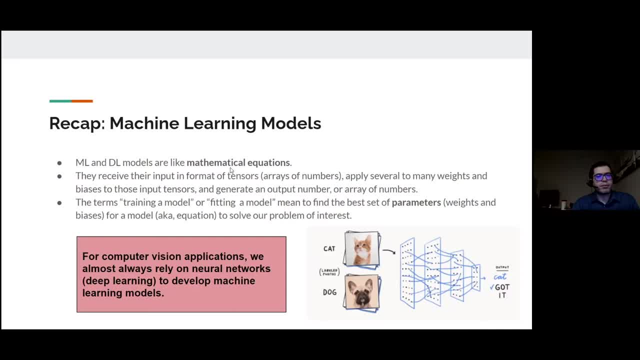 you can naively imagine them as a very, very big mathematical equation that receives some inputs and then does some sort of operations with those inputs. For example, it multiplies the values received from you to some sort of parameters. add them with some other parameters. 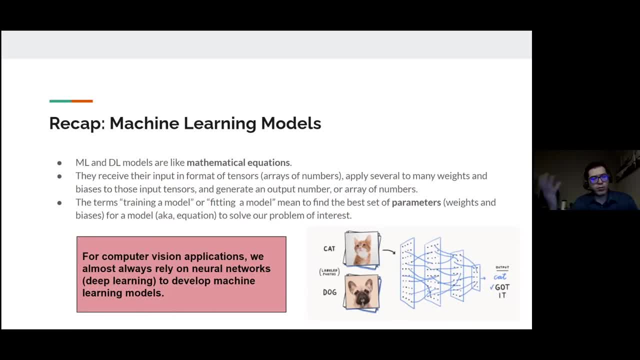 and then finally generates some sort of output for you, So that generated output could be a single number, for example, denoting the risk of dislocation, or it could be a single number, either zero or one saying that this patient has COVID or has not. 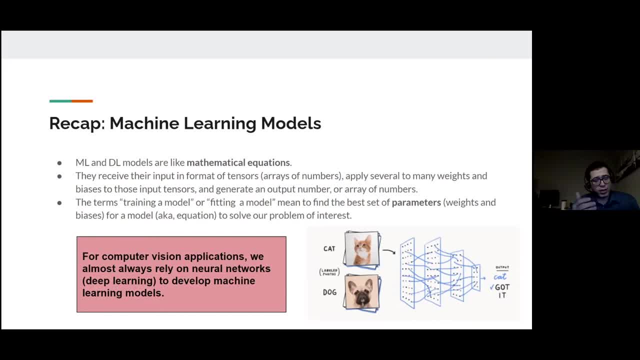 or it could be a complete image in image generation models, right So. those outputs do not need necessarily to be one single value. This could be a lot of values, even a very large set of values as an image itself, right So? but the 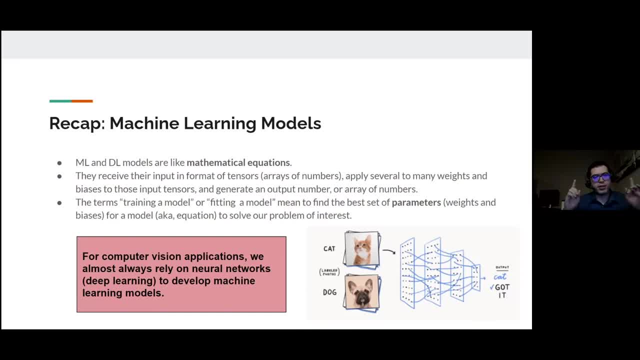 the concept is going to stay the same. Whenever we talk about deep learning and machine learning, we are going to talk about a big equation, And when we talk about training a model or fitting a model, we usually mean to find, or we want to find, the best set of parameters. 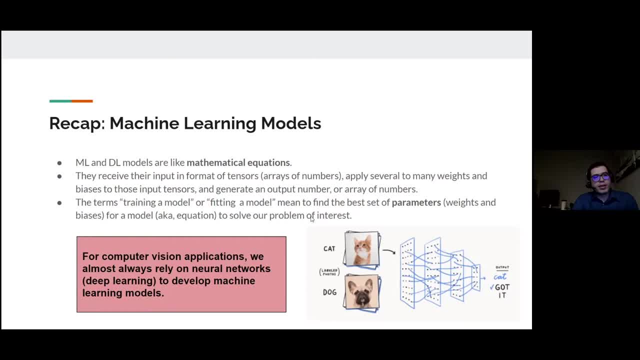 People also talk about them as weights and biases for that specific equation, which basically means that we are looking for those parameters of our equation, that if, for example, we provide it with a picture like this or a picture like this dog, it is going to accurately say the name of this animal inside the picture. 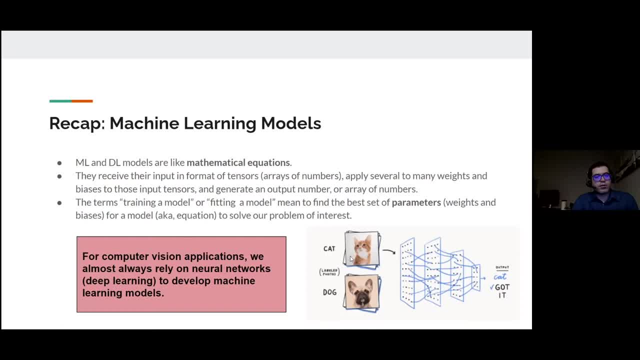 right. So this, this is going to be the kind of model that we are looking for, a model that receives an image and it is able to distinguish whether or not it is a cat or whether or not it is a dog, And for doing so, 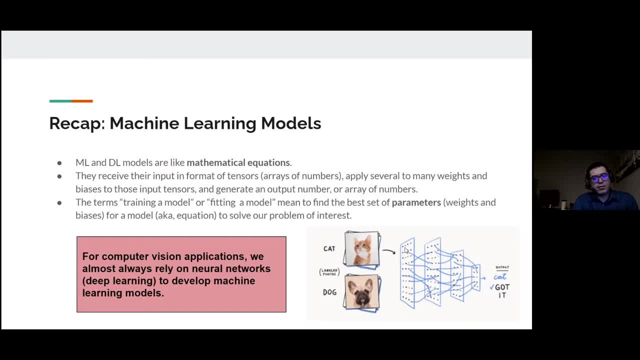 we need to change the mathematical values, the, you know, the, the raw values of all these parameters that our model might have. So this is actually, you know, this is actually called training, Whenever we say that we are training a model. 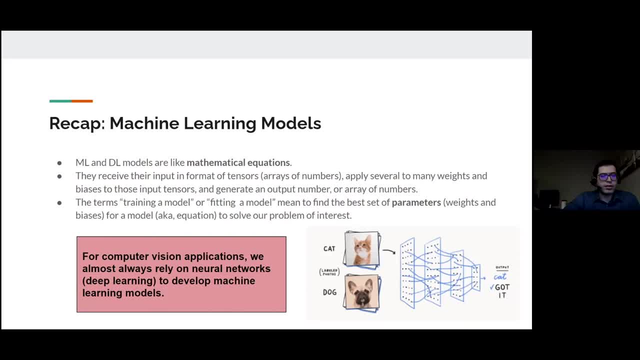 it basically means that we have a neural network or another machine learning model And now we are going to learn what parameter are going to work best in that specific model for us. So, as I told you before, for computer vision applications we almost always rely on neural networks or deep learning to develop machine learning models. 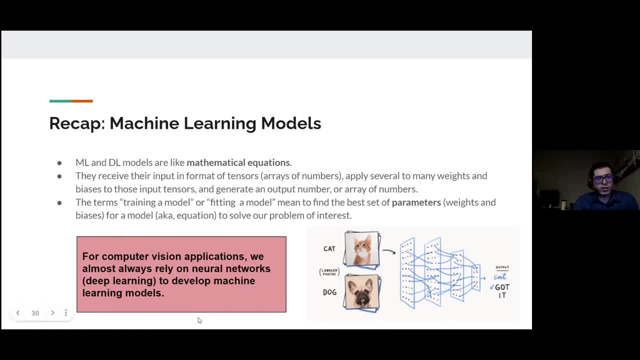 Not to say that we do not use conventional machine learning. Of course conventional machine learning is very valuable, And sometimes the combination of these two work even better than deep learning alone. right, But no, deep learning is almost there, right? 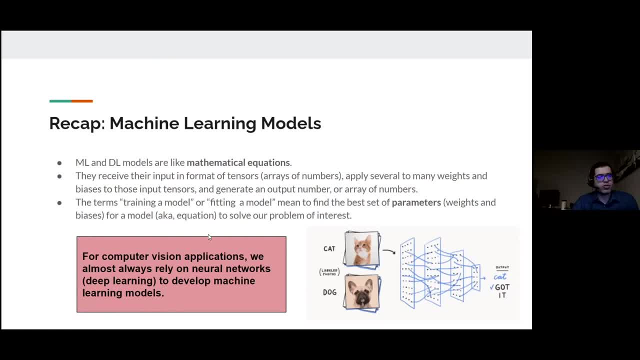 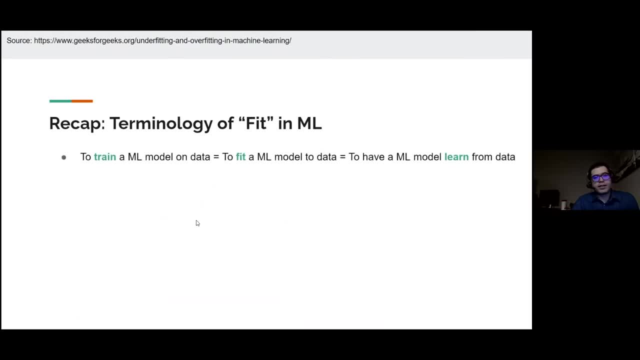 It's always there Whenever we talk about medical imaging. deep learning should be there most of the times. Okay, Now again. the second recap is about the terminology of fit in machine learning, And this is a slide that I had shown you before. 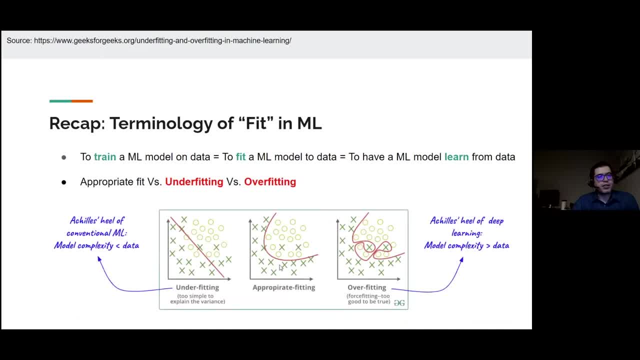 You probably remember that whenever we want to train a machine learning model, we are looking for an appropriate fitting. And appropriate fitting means that our model, first of all, is able to really classify, you know, or to really do the job that we intend it to do. 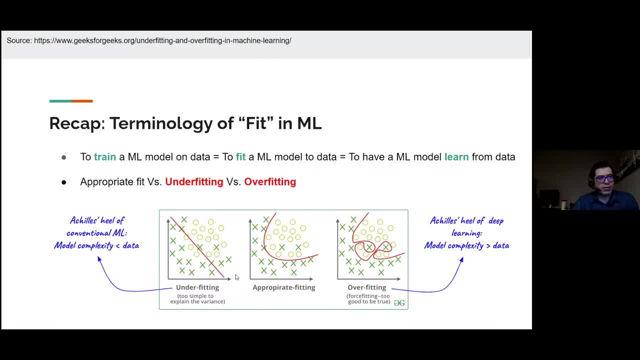 So, for example, this is a kind of a classification task. We want to distinguish these circles from these cross signs, And if we have a model that can draw a line like that, it is probably distinguishing these two classes from each other. If it does a job like this, 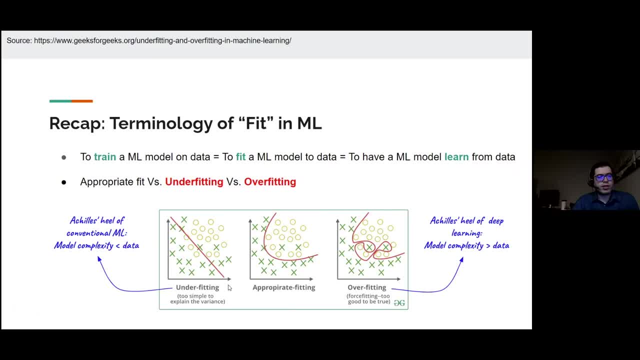 it basically means that it has not learned anything, which we usually refer to as underfitting or right. You know, we said we. we probably see these in cases where our models are too, too simple to learn the complexity in our data. 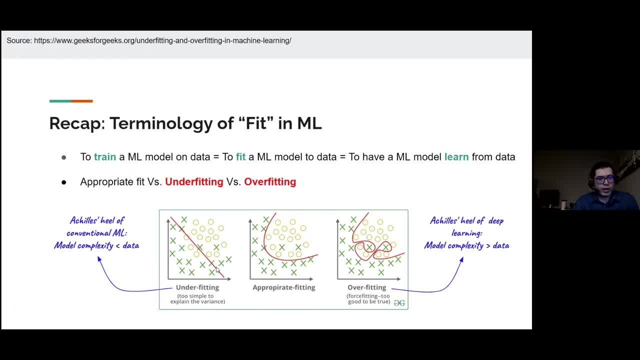 For example, you have a very, very small neural network, but you want that neural network to learn something very complicated or to predict something very complicated, right? This is, as I told you, the actual field of conventional machine learning, because those conventional models are not usually as big as deep learning models. 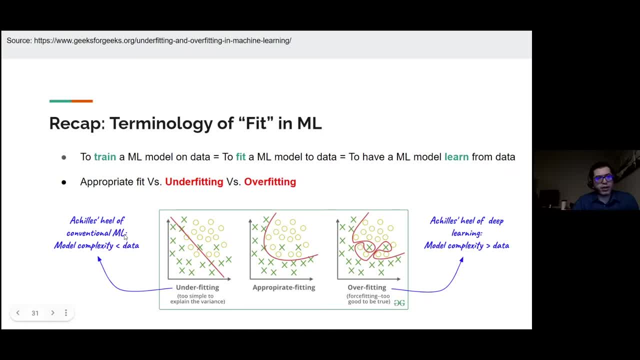 So they usually tend to underfeed the data- or not always, but they usually tend to do so. And then, on the opposite end, we have another unwanted situation that is called overfitting, And this is the auspicious leap of deep learning models. 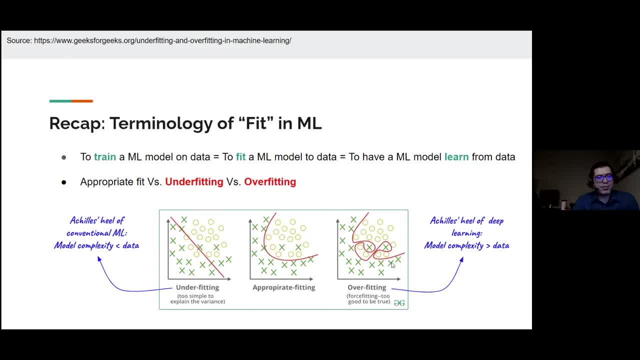 because those are very bigs And this means that they can basically learn to distinguish your two classes like this, which basically means that they have learned the noise in addition to the real signal in your data, And we don't want this to happen. 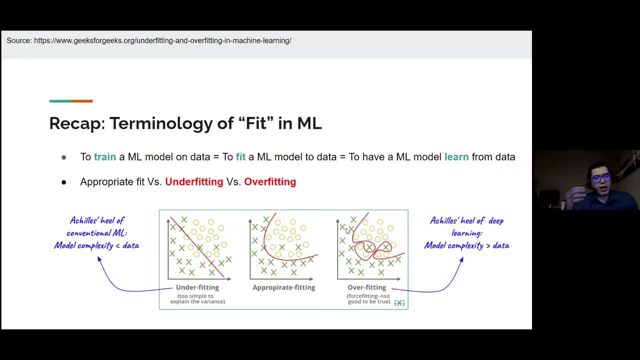 right, Because if a model is doing a job like that, it somehow can be interpreted as this: The model has memorized your data but has not learned anything. So you should be very careful with overfitting whenever you are training a deep learning model. 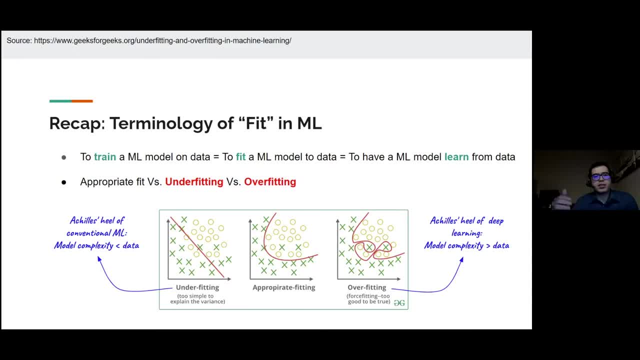 There are strategies to overcome overfitting or at least mitigate that, like increasing the size of your training data, reducing the complexity of your model. I'm not going to talk about those in details here. You can easily find a lot of research about that if you just Google it. 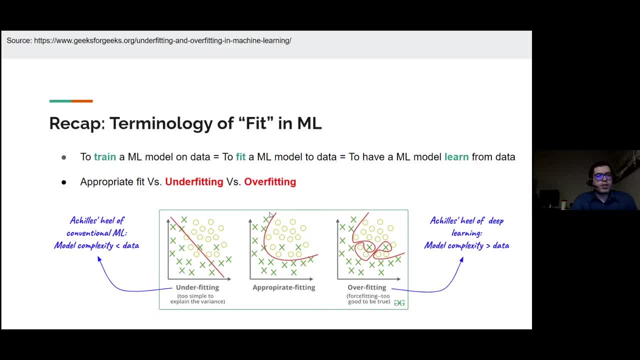 But, for the sake of this presentation, only keep in mind that we are looking for an appropriate fitting. Overfitting and underfitting is something that we do not want to happen, And I'm going to talk about that in a little bit. 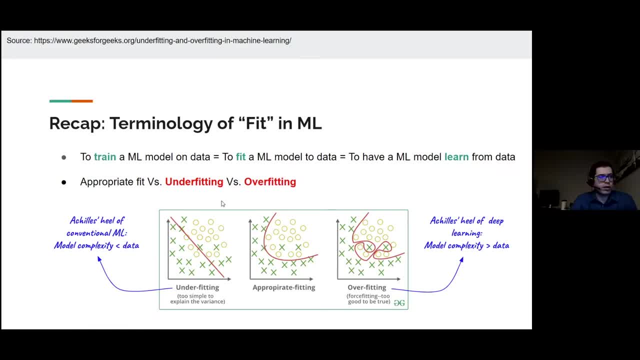 But I'm going to talk about that in a little bit. And I'm going to talk about that in a little bit And I'm going to use this concept later on when we talk about convolutional neural networks. Now, the concept of loss: 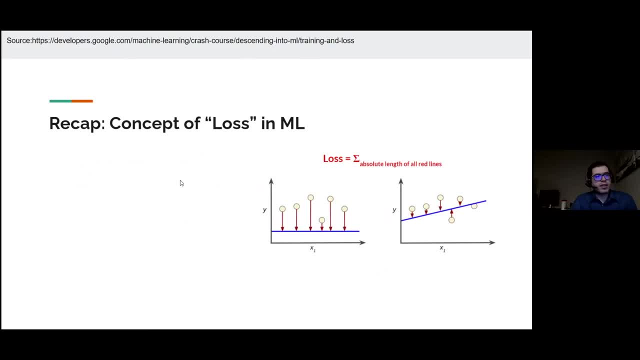 that was something that Alex introduced to you in his last presentation. You probably remember that loss is a measure of how good or bad a model is performing And whenever a model is doing it, or better to say, the poorer a model's prediction or the poorer a model's performance. 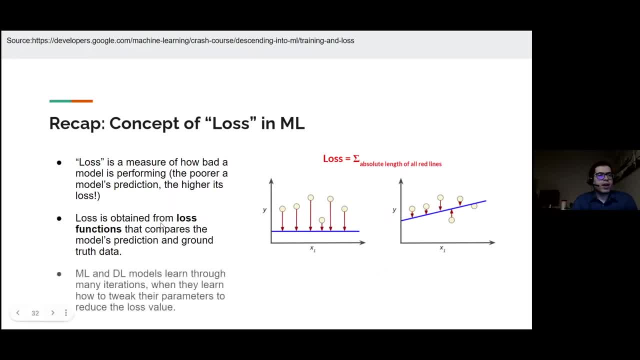 the higher its loss right. So we have functions, mathematical functions, called loss functions, And the way they do, the way they operate is by using the loss function And the way they operate is by using the loss function. And the way they operate. 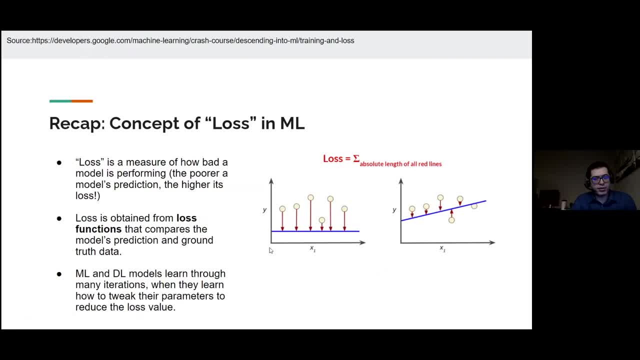 is not that much complicated. They receive the ground truth labels that we really expected the model to generate for us. For example, this could be the labels that your experts annotated for you And then the automated labels that the model actually generated, And we compare these two. 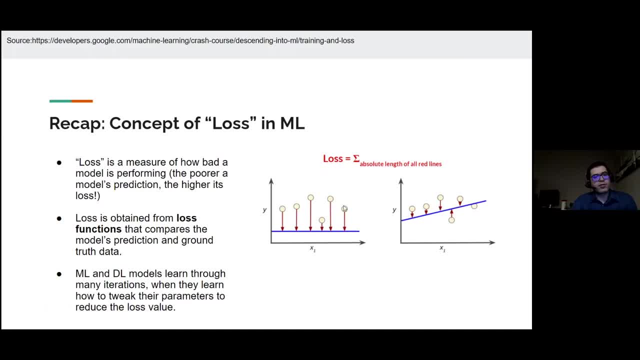 And the difference between the two is called loss. So, for example, look at this image on the right. We want to actually find the equation for this blue line in a way that it can somehow fit this data, these data points that we have on this kind of page. 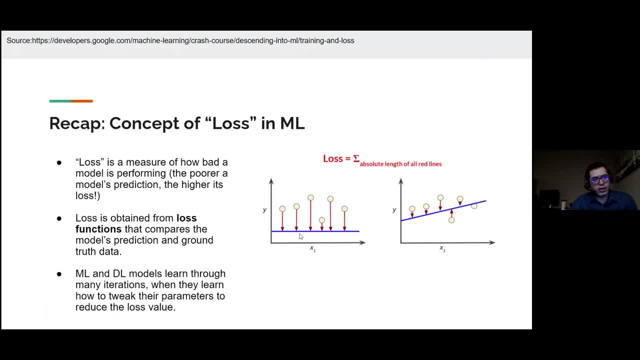 So if we have a model like this, if our line is actually like this, then it means that it is not doing a good job. So one way of obtaining the loss value for this model is that we can, for example, get the absolute length of all these red lines right. 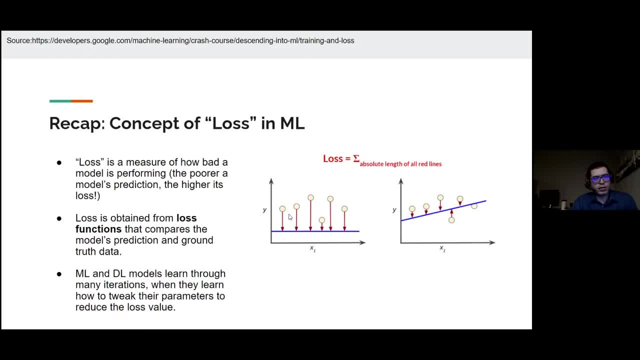 And then try to sum that together or sum the square of those together, And this could be loss. So, for example, if you do the same thing here to this second model, you would probably expect a less loss. I mean a lower loss value, right. 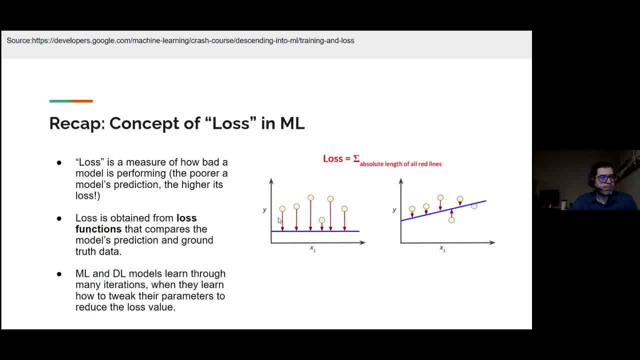 Because the model is actually doing a better job here. So the concept of loss function is something that you should know about, And you know machine learning and deep learning models learn through many iterations, So this is actually how the training happens, right. 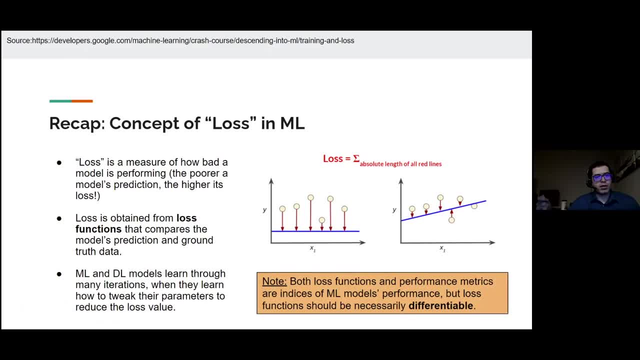 We punish deep learning models or machine learning models and make them make the loss lower to reduce the loss. So if the model is actually- I mean changing its parameters- in a way that loss is actually getting higher and higher than the force, the model using the concept of gradients in mathematics. 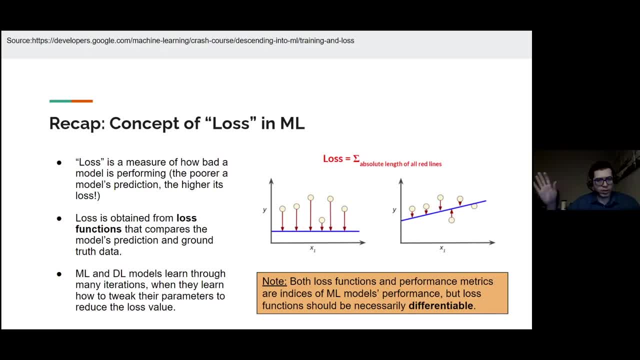 And if you do not know about these or you do not care about this, just forget what I just said. but the magic of deep learning or machine learning usually is depending on gradients and you know differentiation in mathematics, but the force or models to actually reduce this loss value. 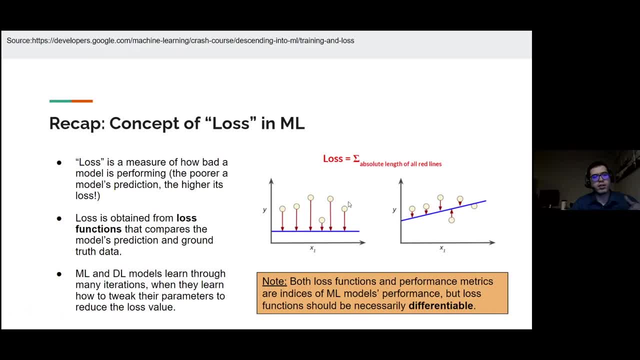 which basically means that we are forcing them to learn how to do the job for us, how to do what we expect them to do, And so the concept of loss is something that you always see right In machine learning publications, or something another concept very close to loss. 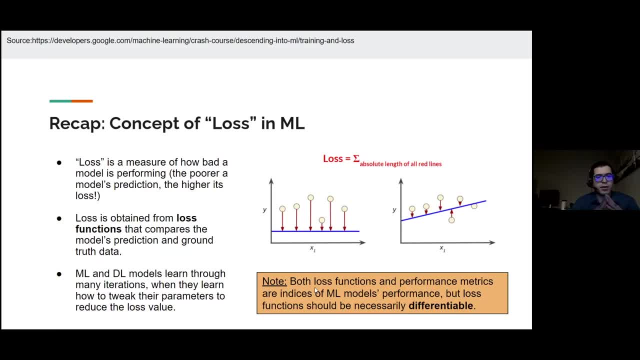 but distinct, I mean distinguishable than that is the concept of performance metrics, which again are indices of how machine learning models are performing. The only problem, the only difference here, is that loss functions should necessarily be differentiable, because we want to calculate their gradients with respect to models parameters. 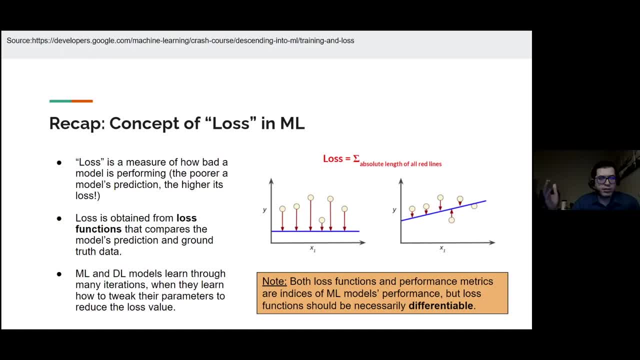 but performance metrics do not need to be differentiable. So if you have a metric that, to be honest, it's something that you just came up with, it works, It's fine, but you do not know- or mathematicians do not know- a way to calculate the gradients for that. 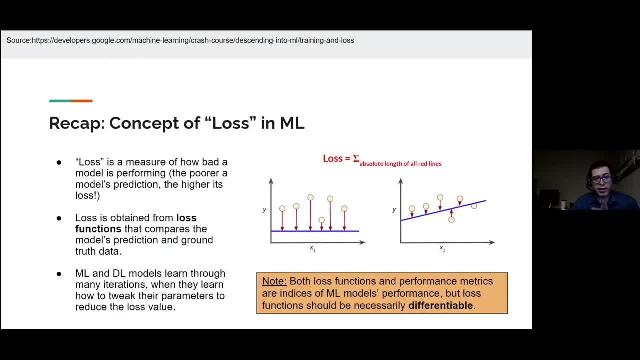 It's fine, You could still use that as a metric. but if you want to use that as a loss function, you definitely need to know how to calculate the gradients for that. That's the reason that we almost all loss functions would also be used as metrics if they have a real meaning to you as a data scientist. 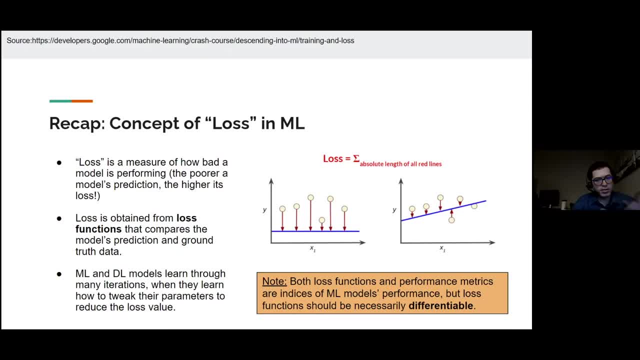 but not all metrics could be used as loss functions. So this is the concept of loss. I would like to pause here and see if someone has questions regarding this first three or four slides. We are only viewing what we have been gone through, Perfect. 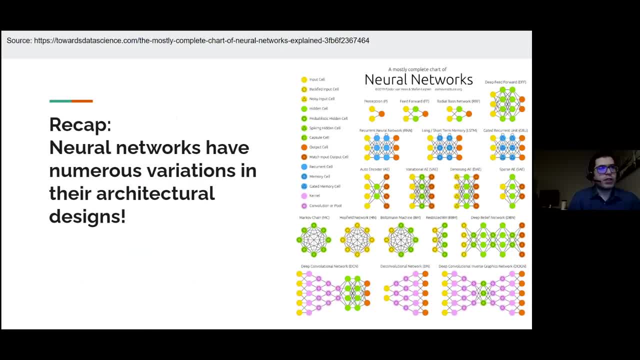 Then let's continue. This is an easier slide. Neural networks have numerous variations in their architectural designs. This is one of the images that I really love, because it shows a lot of architectures. These architectures are quite easy, but, to be honest, it somehow reminds me of the world of Lego and how you can build a lot of different architectures using your Lego pieces. 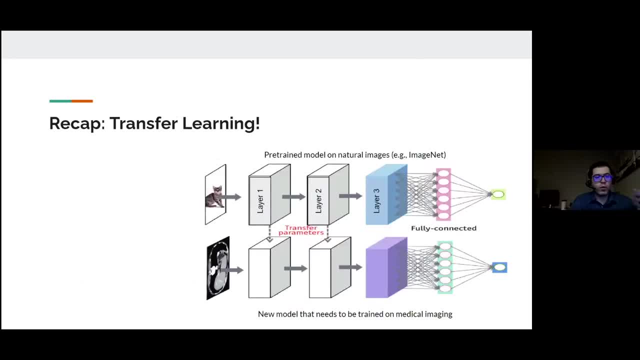 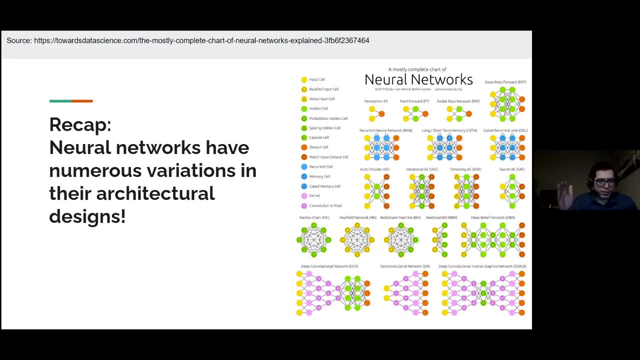 So just just keep in mind that neural networks are not only one type of mathematical equation. We basically can have as many neural networks as the number of data scientists working in the field, because everybody's innovation and creativity could result in a new model or new architecture there. 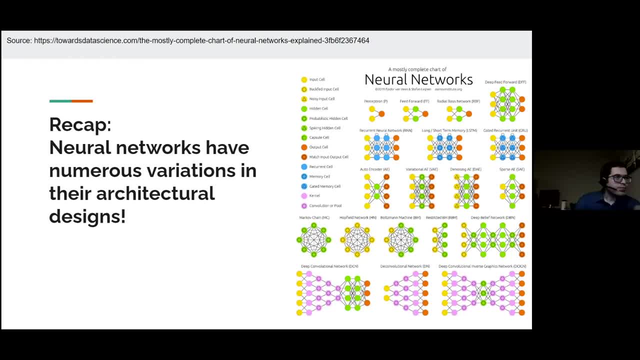 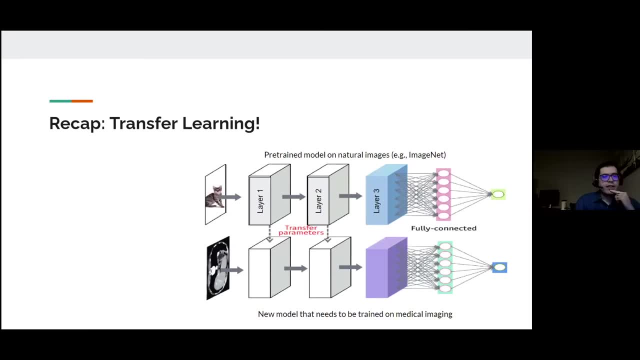 which basically means that to design your equation in a new way. So- and this is the concept of transfer learning that I mentioned earlier very briefly, You remember that we talked about that very big ImageNet data set that only consisted of natural images. 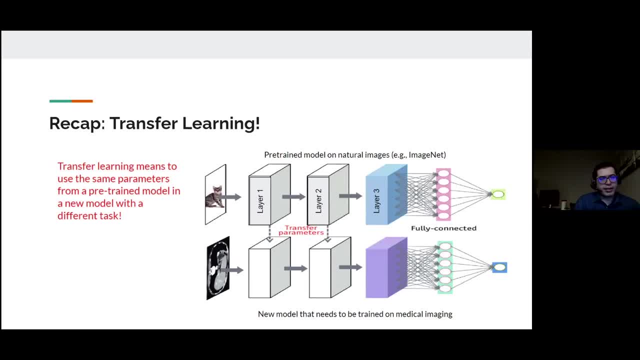 Now, the way that we can use transfer learning is that we do not necessarily need to always start our training with parameters that have random values, because you know in a, in a very, in a naive training, in a standard pipeline, when you are training a model. 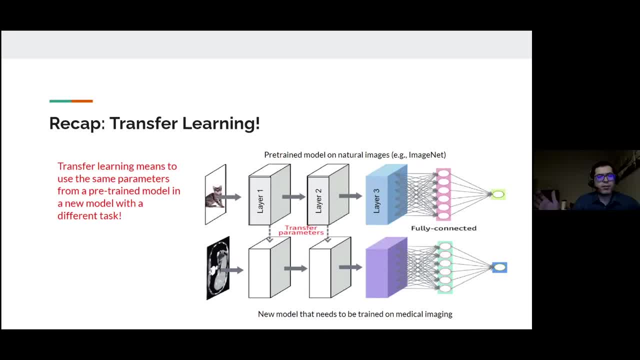 your initial parameters are totally random values. I'm not very random, but no random following a specific distribution, but they are still random, right. So there is a concept there that say that you know if a model was already doing a good job in another task. 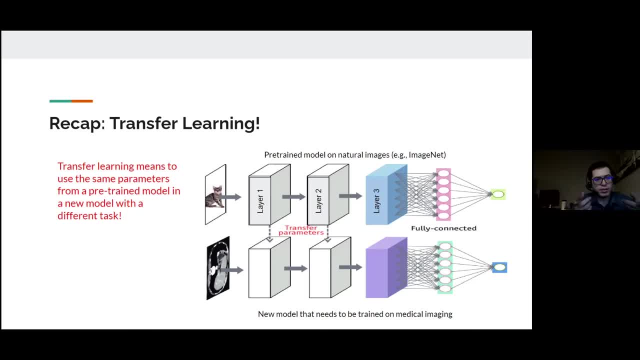 which might be close to what I have in mind to do with this new model. we probably can take some of the parameters of that first model and use those values as the initial values of our own new parameters in this main new neural network that we are building. 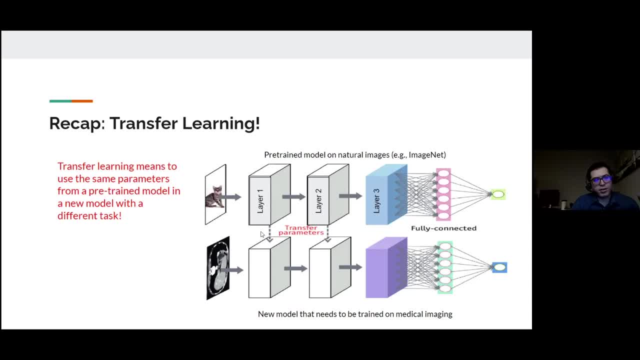 right. So this is the concept of transfer learning: We take the parameters from an already trained and already decently working model and put those as the, as the starting values for the parameters of our own models. Of course, there are some limitations there. 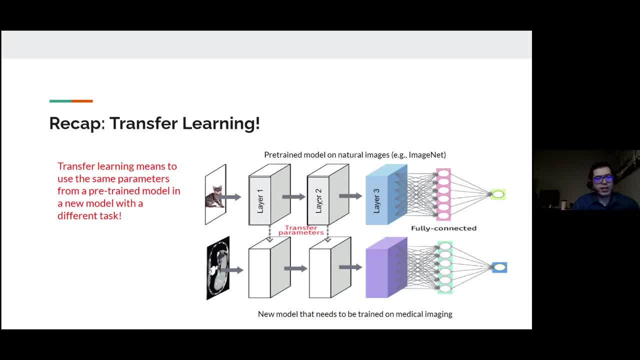 For example, at least these layers that we are transferring the parameters from and to each other. those should have quite similar architectures And you know this is this is something that needs some time for you to understand how to optimize your transfer learning pipeline. 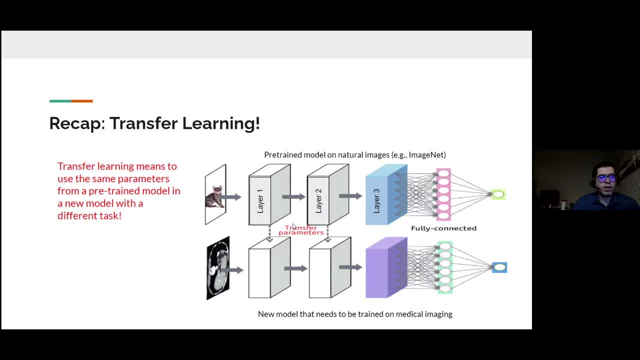 what weights to update, what weights not to update during the training. But the concept, very simply saying, is: exactly what I'm saying, Exactly what I told you. Now you might say that, okay, does that really help if we transfer, learn from a model that had been trained on images like this cat? 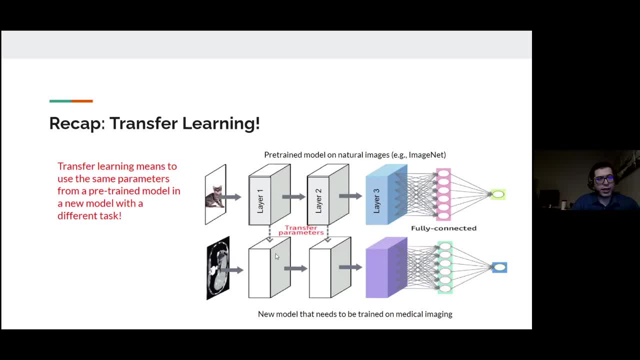 for example coming from ImageNet data set, and then transfer, learn from that to models that we want to train, for example on the CT scan. The answer is very interesting and it is yes, it sometimes helps. Of course, it's always better if you have a model that has already been trained on CT scans and you know that it was working very good. 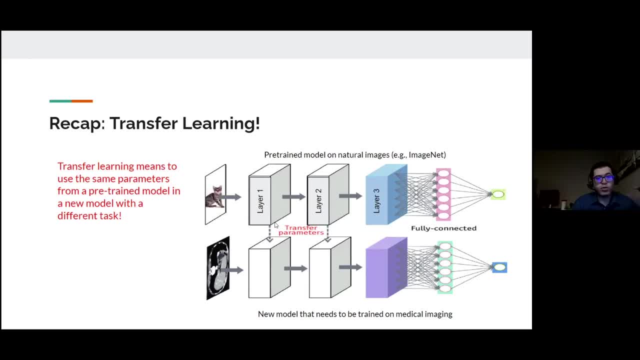 transfer. learn from that. Nobody's going to blame you for that. But if you do not have access to that, what we usually do- and this is our, you know nowadays- baseline practice- is that we almost always start our models with parameter values coming from pre-trained models on big data sets like ImageNet. 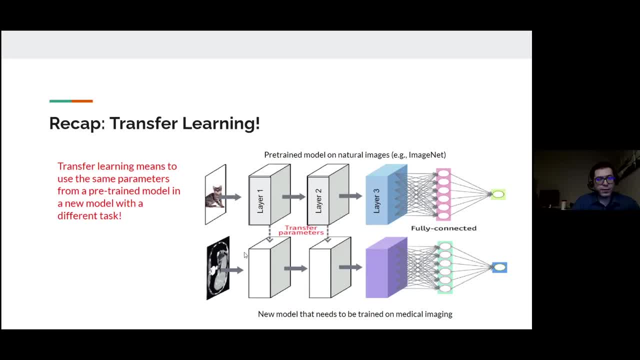 The reason that these models still work is actually the main intention of this part three presentation: convolutions and features that models are going to learn. So keep this point in mind and keep this question in mind. I'm going to return back to this. 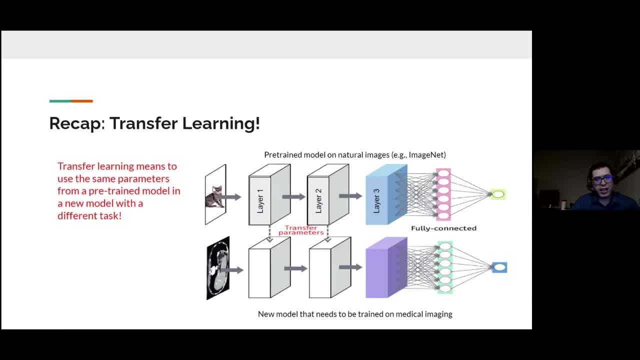 telling you why these models that have been trained on cat images might be useful for training new models on CT data or MR data. Right, So we're going to talk about now reminding you of overfitting transfer. learning reduces the need for training data. 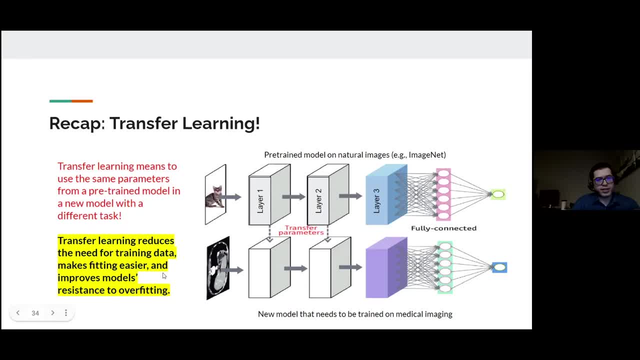 makes fitting easier and improves models resistance to overfitting Right. So basically it means that. so the general intuition for this is, as I tell you now, you are starting your model parameters very close to another model that had an appropriate fit. 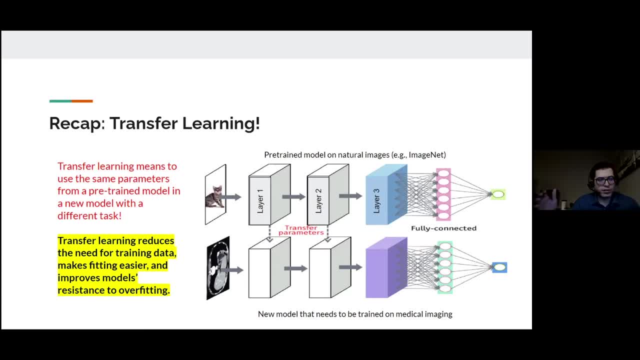 So you will give more chance to your new model to find an appropriate fit right, Rather than you know, living it in a very large world of parameter values that it needs to iterate through and learn by itself what values work the best for it. 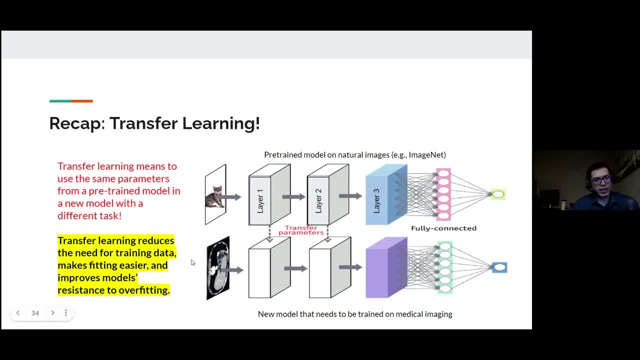 Right. So you basically give it a hand in the beginning of the training. And this is just an intuition, right? So behind the scenes, transfer learning actually has mathematical reasons. that works better for combating overfitting. So have this in mind, right? 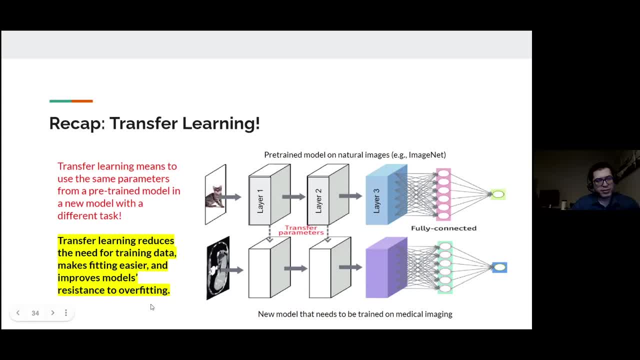 Okay, So this is a very this is something that we do as a best practice, So keep in mind. so, rule of thumb: whenever you could do over transfer learning, we always do that right. This is something that we do as a best practice. 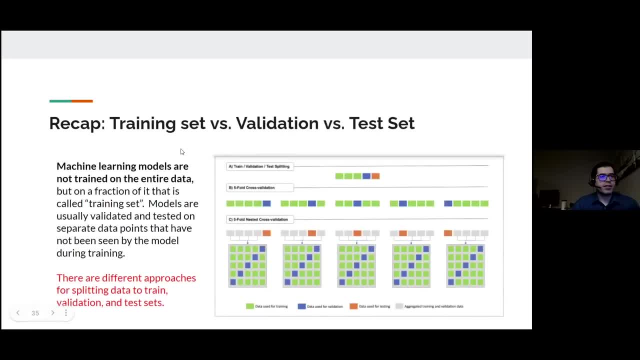 Now training. validation test says we talked about this when we introduced Frankenstein data sets. As I said, we want to train our models and then validate those on separate sets. Sometimes even people tend to validate their models on a set and then finally test that. 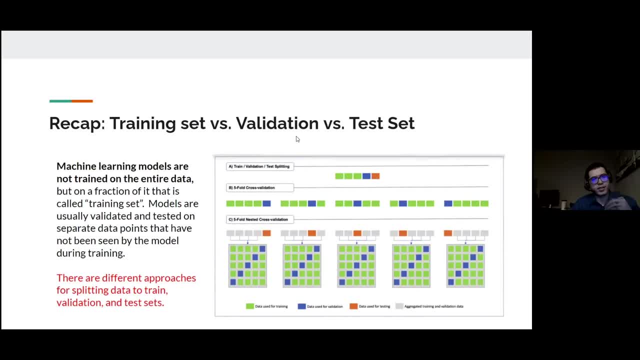 I mean evaluate that at the end of all their iterations on a separate set that is called a test set. Now we have different ways for dividing our data points between these classes, between these sets. The simplest one is actually the train validation test splitting. 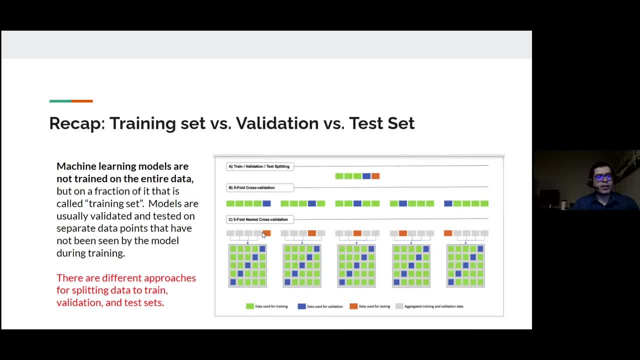 Now we have five full cross validation and we do have nested cross validation that I learned about two years ago from Dr Bart Tremers here. So basically, there are different types of data set splitting here, and the best ones are usually the ones that we have. 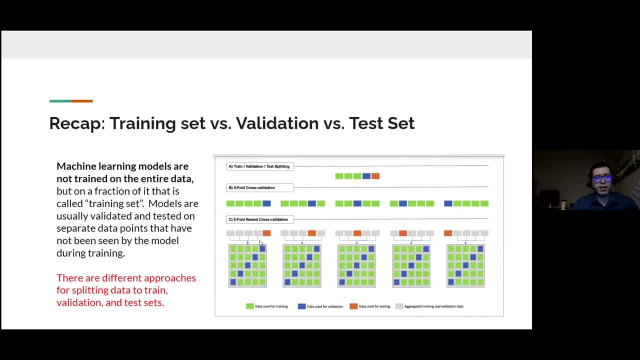 I mean nested cross validation- is usually the best one to do. Sometimes it's difficult to implement in real practice, specifically in medical work, because if you have 10,000 images, most of the times it's not like that that these 10,000 images come from 10,000 different patients. 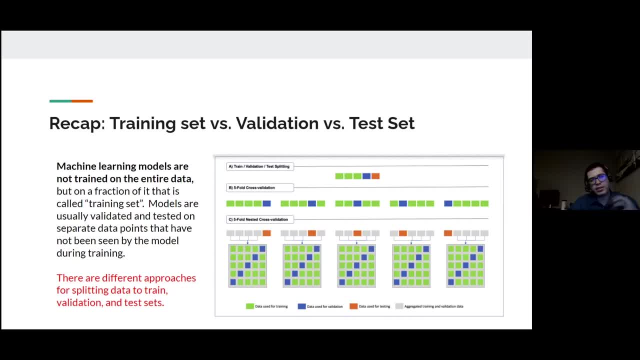 Usually each patient has multiple images And then if you want to split the data to different folds- and too many folds- you will face issues like you know. oh, one of my folds now doesn't have any images from a specific classes, right? 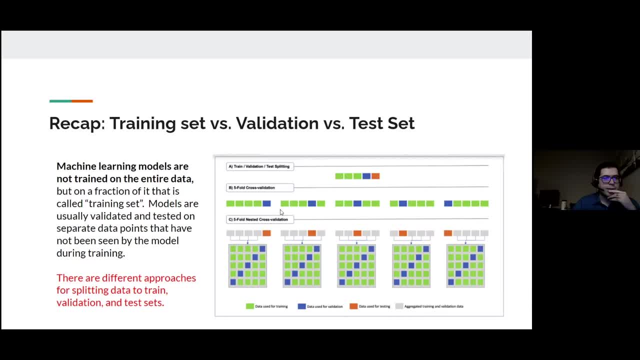 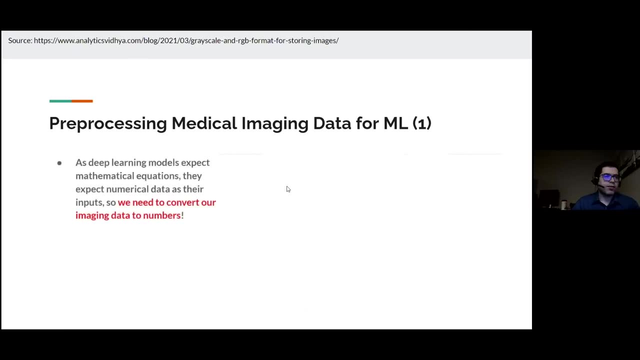 So this is not something always easily implementable, but at least train validation test splits need something That we all need to do as the least minimum thing that we need to be careful with, and data splitting Now. processing medical imaging data for machine learning. 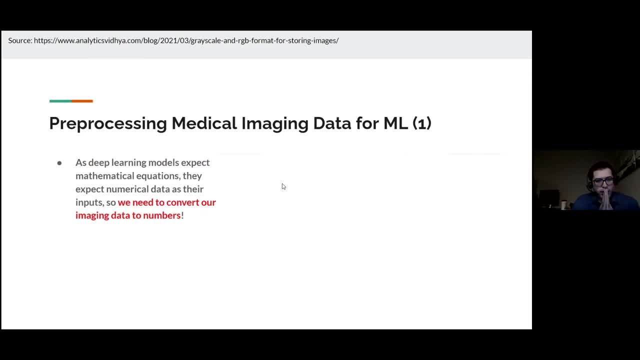 right. So now I'm going to talk about the main issues here. A deep learning model, or machine learning model in general, expects data- input data- to be in format of mathematical values. They expect numbers, They expect quantitative variables. Now you might ask yourself: 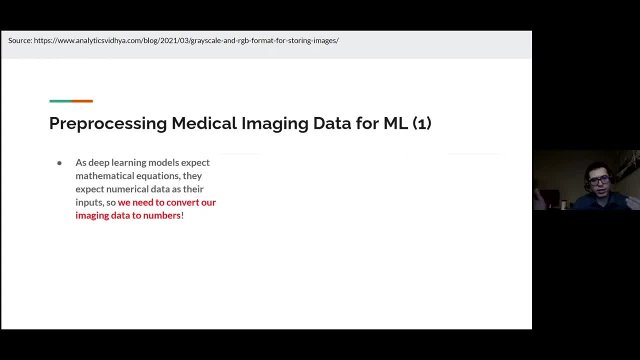 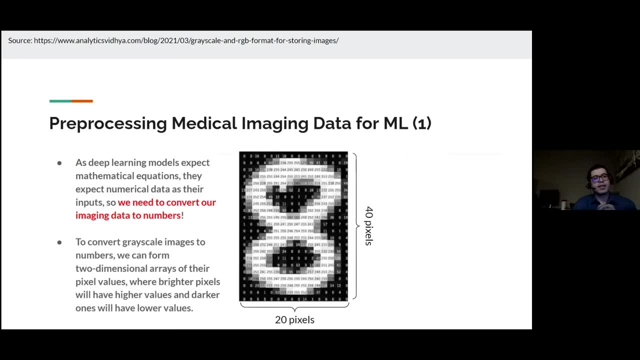 how are we going to convert Our images, natural images or medical images- to numbers? And this is by using the concept of pixel values, right? So, for example, if you have these gray scale or you know black and white image of number eight here, 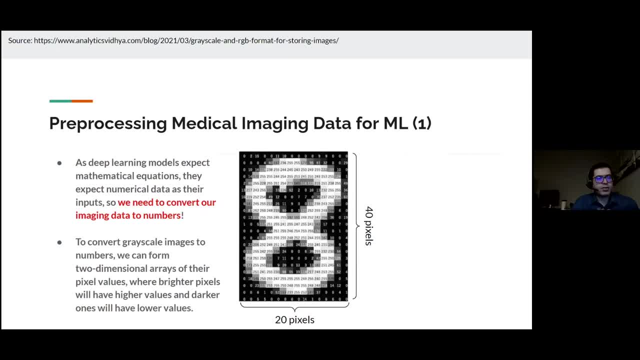 you can imagine that, for example, we have 40 pixels and 20 pixels as height and beat of this image, And what we can do is that we can say we have a 2D matrix with 20 multiplied by 40 elements. 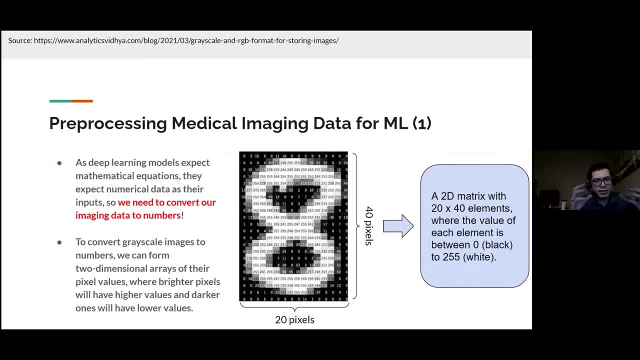 So 800 elements here, And this matrix is now going to represent our imaging data, right? So imagine that each element value is going to be between zero- which zero means black- and 252, 155,, which this number actually means entirely white. 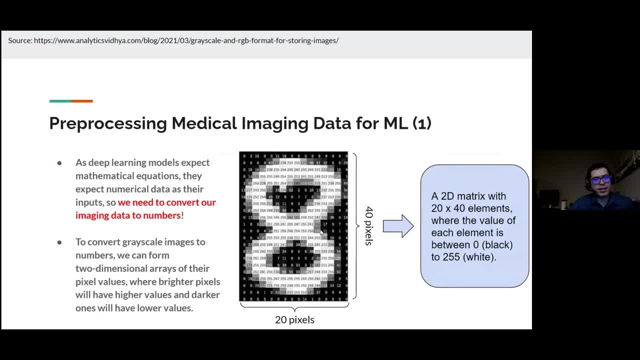 So if you have a value between zero and 255 in this eight bit image, this basically means that it's going to be some sort of gray for you, And this is how we actually build gray scale or black and white images, right? So most of the imaging type that we deal with in medicine. 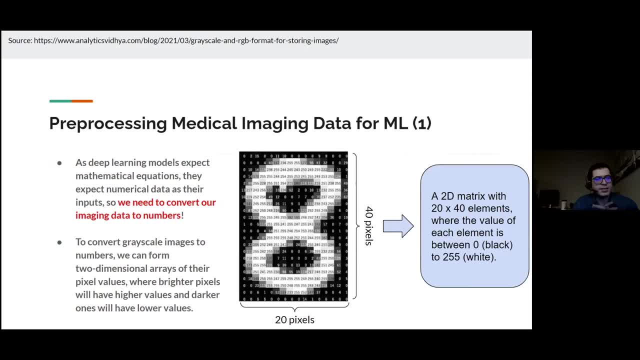 right? So most of the imaging type that we deal with in medicine, right? So most of the imaging type that we deal with in medicine are already black and white or gray scale, like X-rays or CTs, So we do have these type of values. 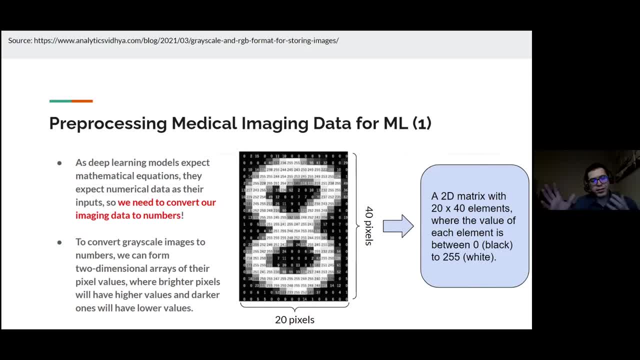 And this is super easy, right? The way that we usually feed our models, feed our input data to the models, is that we take these matrices out of those images. We say that, okay, this is an image. So let's say: 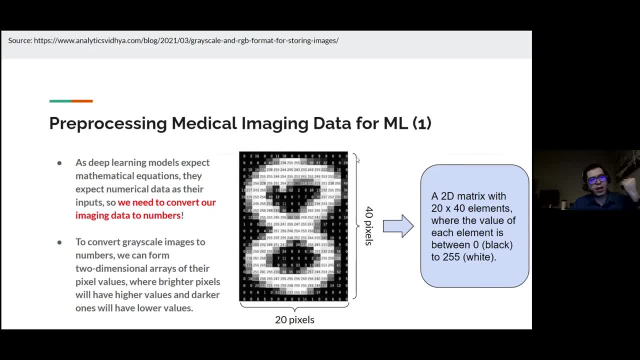 let's convert that, Let's actually get these pixel values out of the DICOMs or out of the JPEG or PNG images and then convert those to matrices that now we can feed to our real machine learning model. So this is the main pre-processing step that we do whenever, once, we want to train a machine learning model in medical imaging. 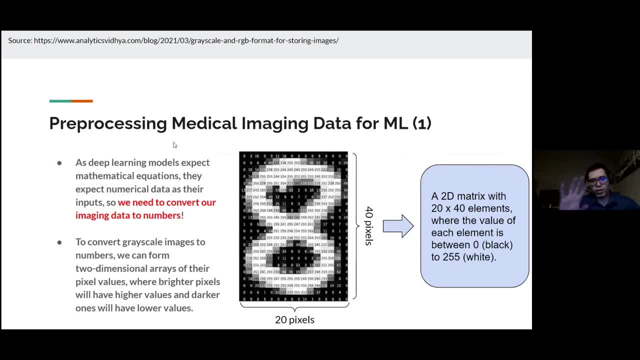 The pre-processing in brief, in general, means that whatever that you are going to do to your data before actually training the model on that data, And the most important component of pre-processing is to convert that data to pixel values, or you know. 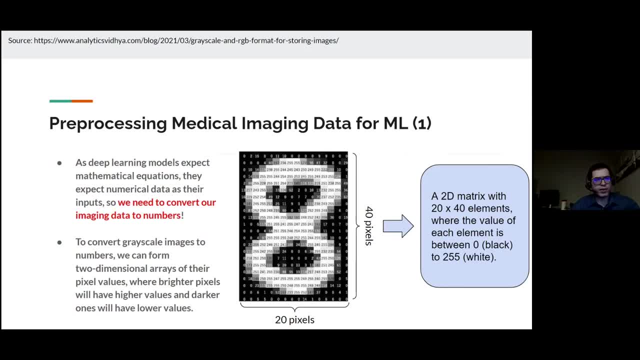 these matrices. Is that clear to everyone here? Do you have any questions about this? Fortunately, clear, Perfect, Now we proceed. Yes, Yes, Question for you. Sure, We keep talking about training, training. Where do you specify your purpose of training? 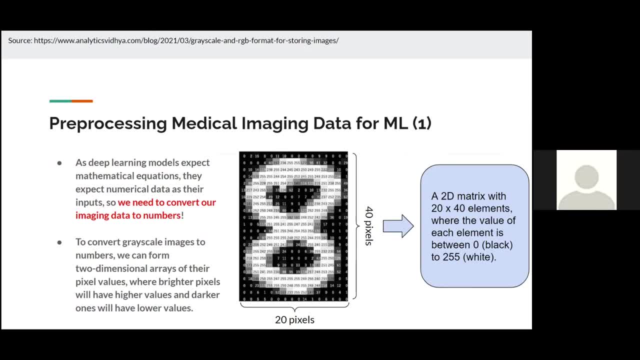 For example, in this case, if you have a set of eight, assume you have another set of, let's say, two image of two. So you have a stack of image like this with a bunch of eight, with a bunch of two. 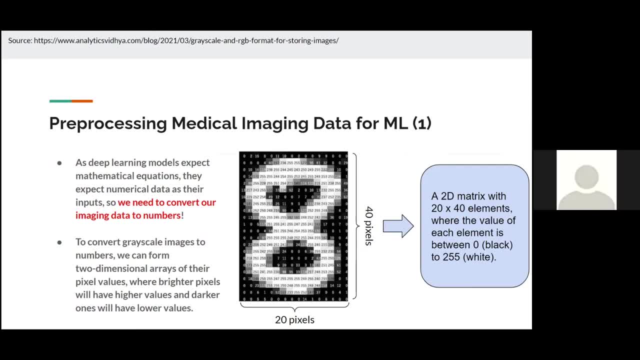 So you want, your purpose is to try to separate them, to train them so they'll be able to differentiate, So something like this: where do you specify that, your model? So because I understand, but I kind of get lost in that. 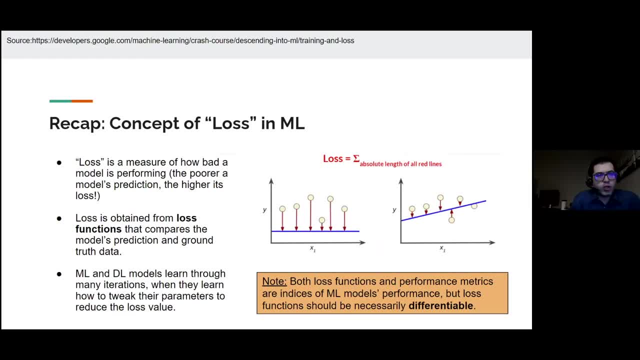 But where do you specify that? Sure, So thank you for this question. Actually, the answer to that lies under this slide. The- I mean our models train by our punishments. right, If I punish my model to force them to differentiate a number? 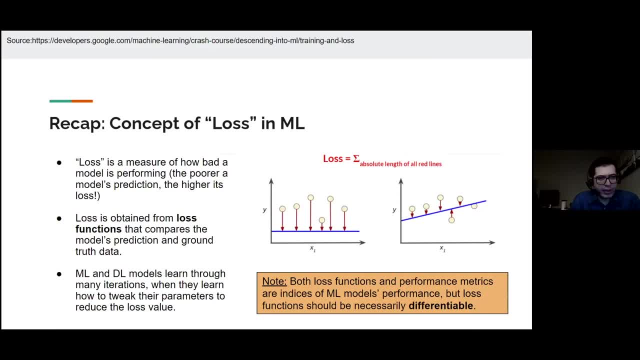 eight from a number two, then they are going to learn that If I punish them or if I force them to learn number eight from number seven, they are going to do that If I force them to differentiate a COVID-19 patient- CXR. 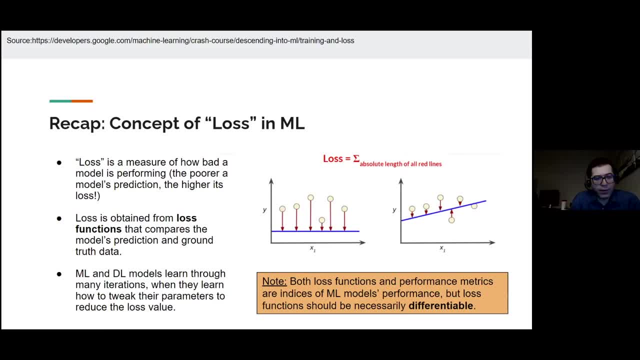 from a normal patient. CXR, they're going to do that, And the way we have for punishing our models are is summarized in these loss functions. So if you're going to train your model for a specific purpose, you are going to have a specific loss function. 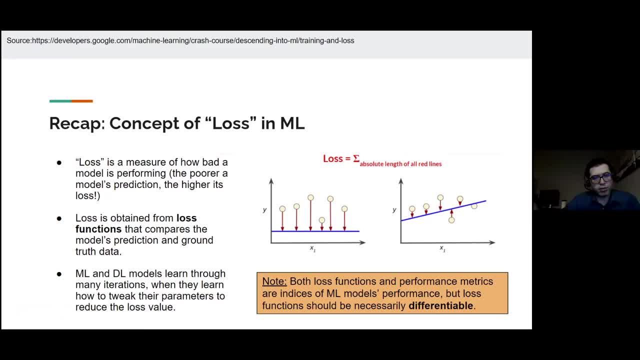 for your purpose. So you'll feed, you'll give your input data to the model and then you have a specific loss function based on your intentions in place that is going to penalize your model for whatever random predictions it makes at the beginning of your training. 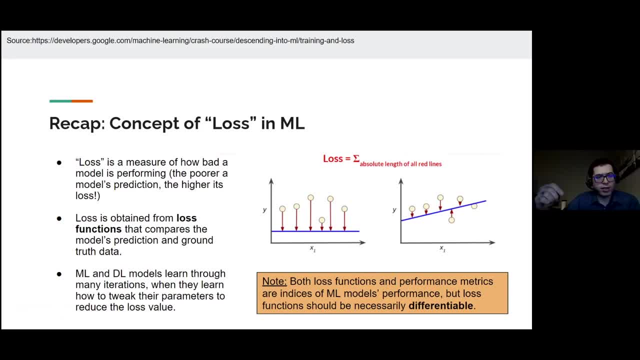 And over time, and after lots of iterations, the model is going to change its parameters in a way that it becomes less penalized, which basically means that it is going to change its parameters in a way that the loss become lower, And again this means that it is going to change. 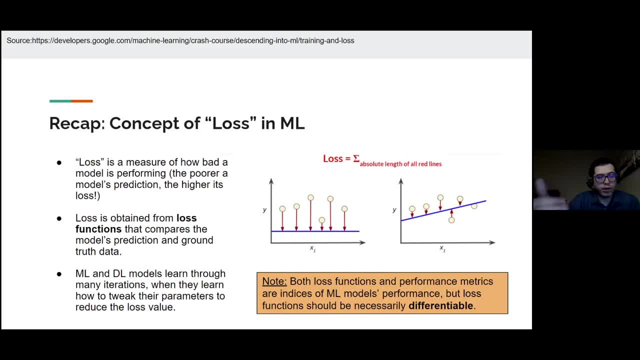 its parameter in a way that it finally learns to do what you wanted it to do. So what we do is that, in your example, we get a bunch of eight images and a bunch of two images. Then we have labels for these, right. 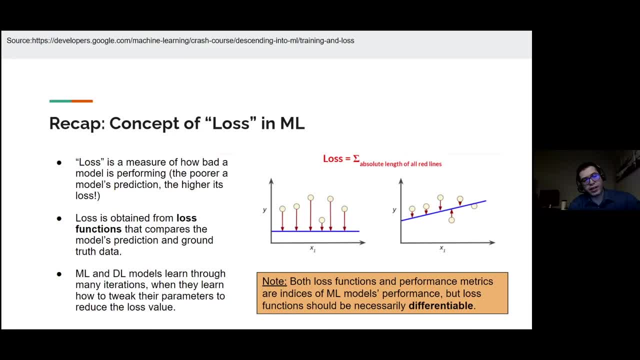 So we know that each image of coming from two side has the label two and every- I mean each of those images coming from the eight category is also have a label eight. right Now we'll feed those images to the model And suppose that we do this one. 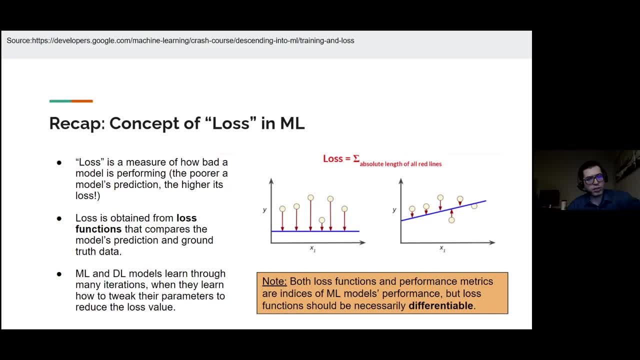 we do not do this one by one in real practice, but let's say we do this one by one. So the first image that goes through is an eight. Now, the real label for this image is eight. Now suppose that your model randomly predicts that as a two. 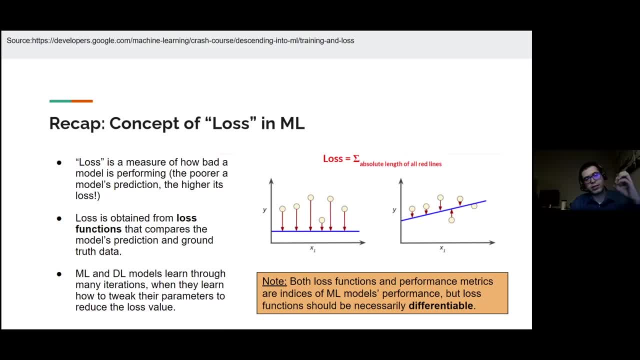 this basically means that now we have an automated, automated, predicted value of two and a real value of eight, right? So in this case, I'm just throwing something out on top of my head, just very easy. Suppose that you actually reduce these two numbers. 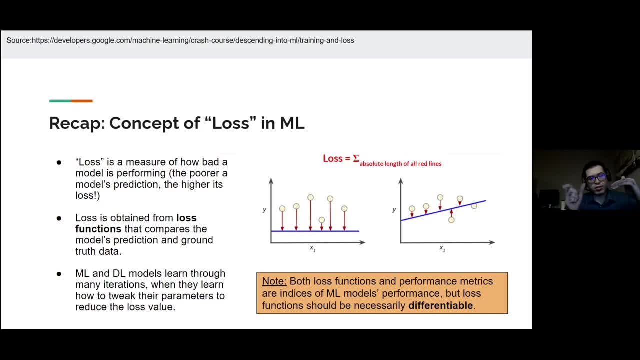 from each other, And then the value is going to be six and do, and then you make that a square, So that would be 36.. And you see that you know the loss for this specific example is going to be 36.. 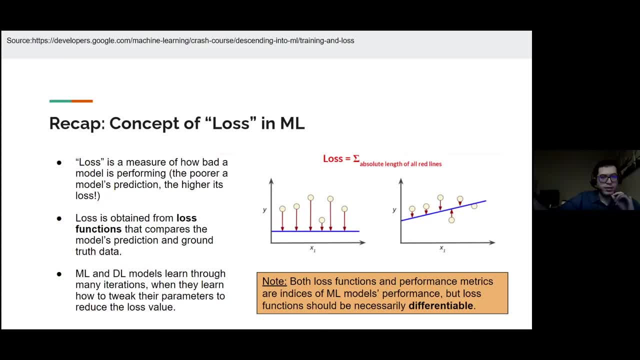 And then you make the. so this is the mathematical part. You calculate the gradients of these final loss value, this number 36, right, With respect to all parameters in your model, with respect to all parameters in your model, And you will have some gradient value. 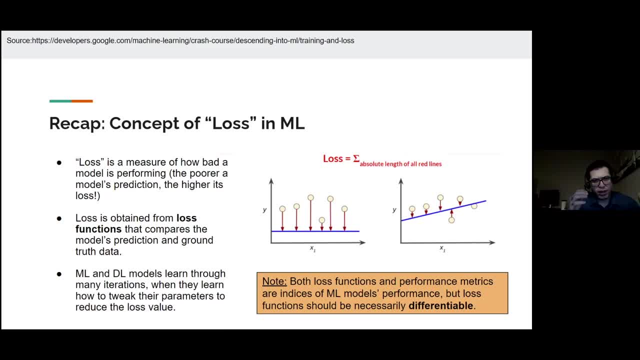 one gradient value for each parameter, which is either positive or negative. And those signs? those signs matter because those signs tell your model that if I want to make these 36 lower now, I need to change, for example, each of my positive parameters more to. 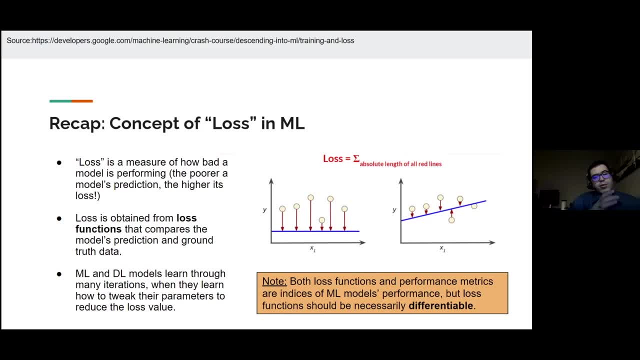 I mean I need to lower them, move them more towards zero And probably I need to move all my negative parameters. move more to our positive side, move them again towards zero. So you change your, you change your model parameters based on their gradients. that were just 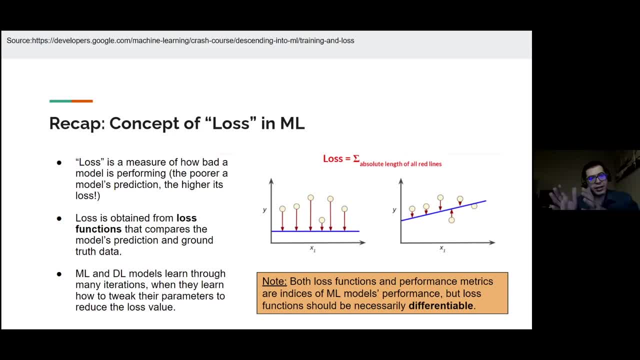 calculated based on your loss, and your loss is calculated based on comparing the ground truth and the predicted value from your model, And this way. so this, this was only one iteration for one example. Now imagine this is happening for a lot of examples at the same time. 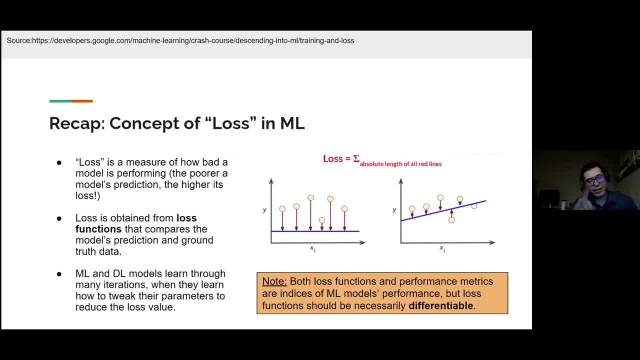 and this is happening for a lot of iterations, right? So, at the at the end of the day, going through all these iterations, one after the other, finally, your model parameters would have values that are going to result in that performance. 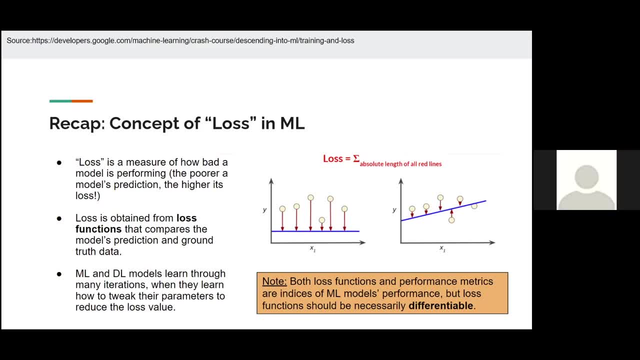 You expected the model to have. Okay. So all what you described for a penalty calculation or those can be specified in the model. Oh, yes, sure, I mean okay. We definitely can specify the kind of gradient operations that we are doing. 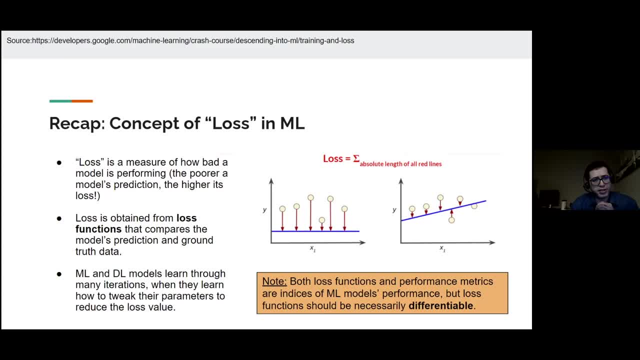 the loss functions that we are providing. What we really cannot do by ourselves, to be honest, is calculating. I mean, we provide, we set the scene for the model, We tell, we tell them that you know you should calculate the gradients like that. 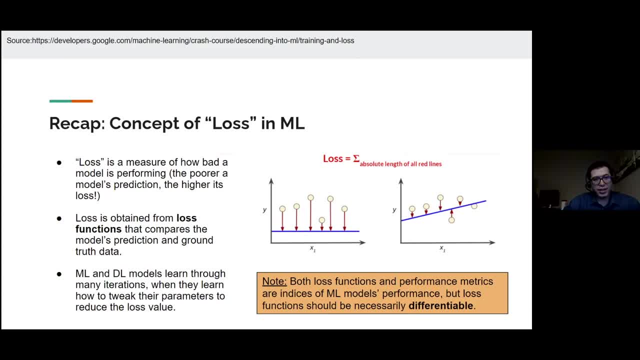 The last function. you are going to use this like that, but the calculations themselves are too much heavy for our naive brains. right, Because millions of operations are going to happen in less than a second, And this is not something that our minds can handle. 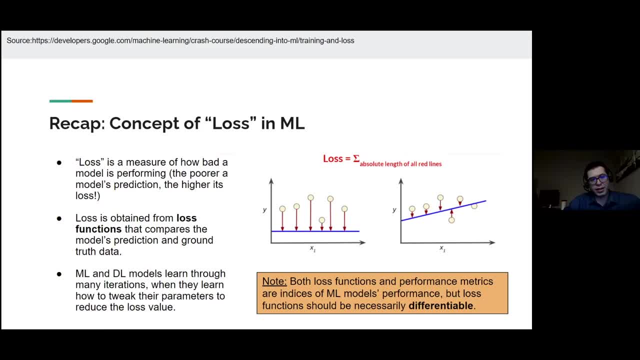 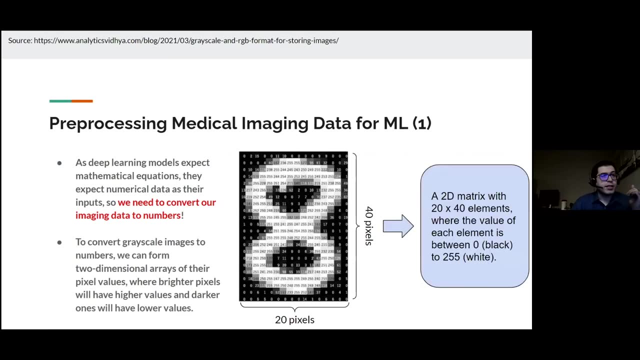 So we we somehow delegate this part to the model and the computer, but we do know what we are doing and how to set up the training. Okay, Thank you. Yeah, no problem, Any other questions? Perfect, So let's proceed to the next one. 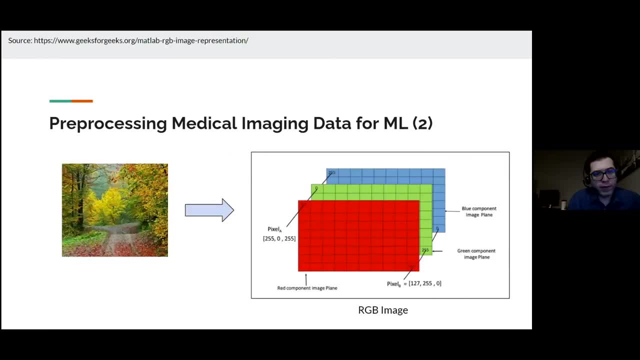 So the same kind of pre-processing or converting of values- you know, images to pixel values- could also be true for colorful images or natural images. The only difference is that you probably know that colorful images are usually RGB, which basically means that instead of one 2D matrix- 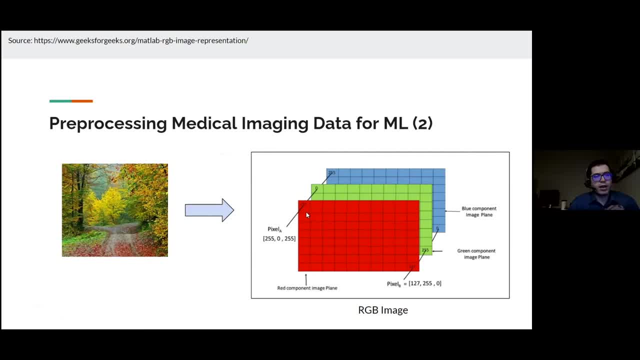 they have three 2D matrix, So one for color red, which basically you know, zero and 255, the range of values there are actually changing the intensity of the red color. Now one specific matrix for green color and one for blue color. 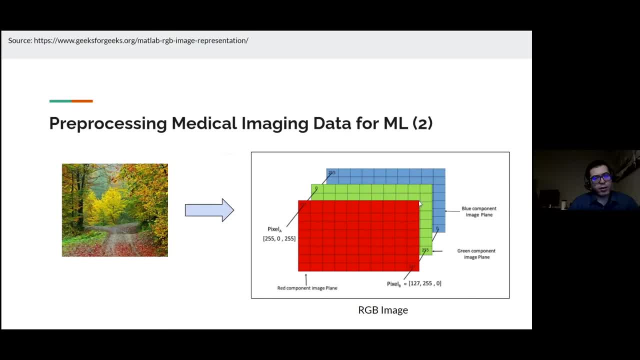 And in data science world we call these type of images a three channel images, So each channel is actually denoting a matrix, a 2D matrix. So if you're going to consider what type of architecture the pixel values of this image would be, 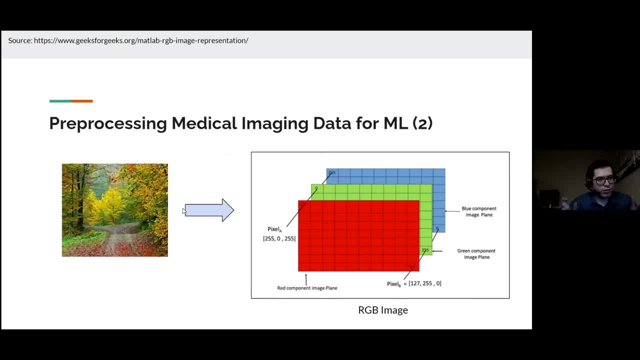 that would be a tensor. That is the term we use for to denote more generalizable matrices, but you can easily replace that with matrix again. So this is a tensor or a matrix that has shape three multiplied by whatever height we have here. 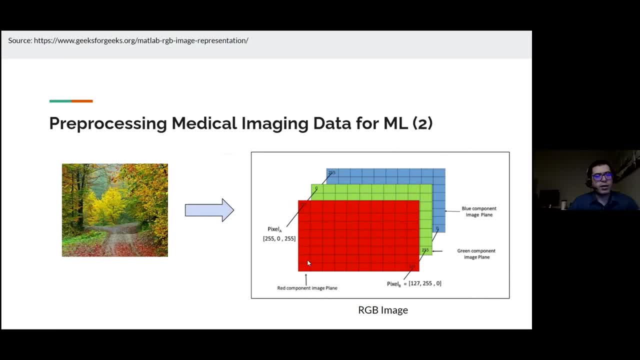 and whatever width we have here, right? For example, if this is 20 pixels in the height and 40 pixels in the width, then the entire number of elements we have here are going to be three multiplied by 40, multiplied by 20,. 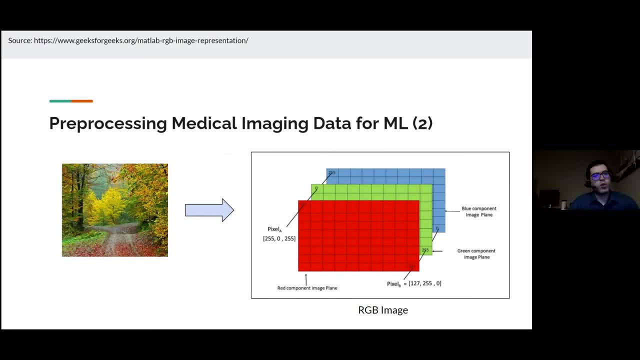 right? So this is going to be a three channel tensor, right? So this is going to be a three channel tensor, right? So this is going to be a three channel tensor, or a three channel or a three dimensional matrix, if you want to say that a little bit better. 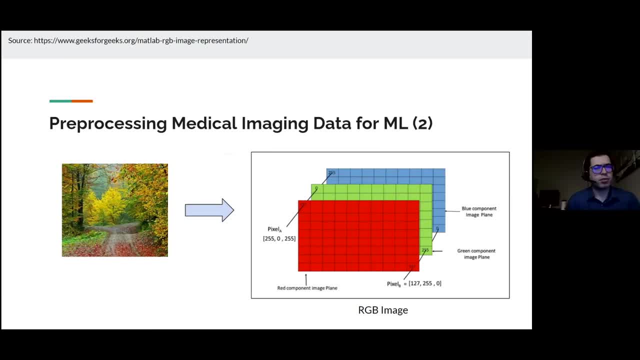 So this is how we convert natural images to you know, pixel values. As I said, we do not most of the time work with these kinds of colorful images. We do care about channels and the kind of data we put there, But most of the images that we usually work with with our models are grayscale anyway. 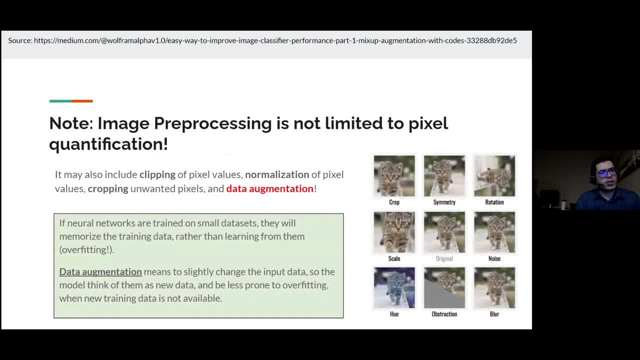 So okay, Now one more thing before we jump to the conversation. before we jump to the conversation, the concept of convolution is that image preprocessing is not limited to pixel quantification or converting your images to pixel values. Maybe I could have put this slide in a better place. 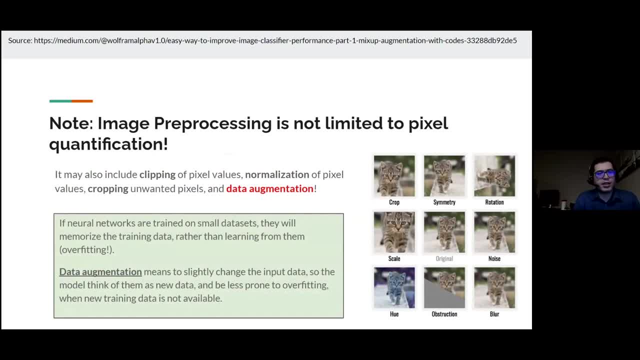 but I just wanted to briefly mention here that you know, whenever we are training our data, we also do something that is called data augmentation, which basically means that you know we try to sell the same images to our model as brand new images. 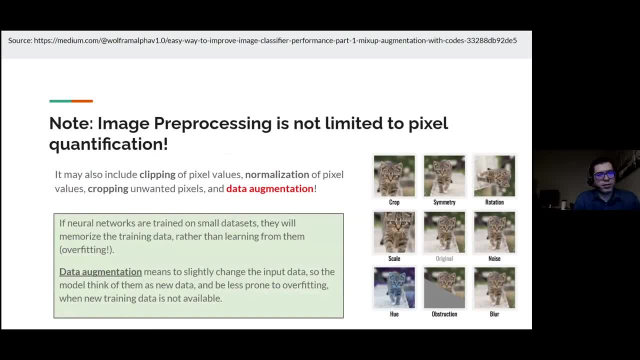 We try to fake them right, We try to play on those models, We. the reason that we do that is that, and as I told you, these deep learning models need too many data, And the reason they need too many data points is that if your data set is a small 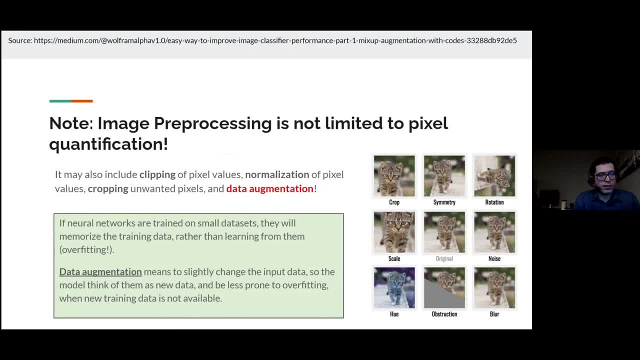 they are quite capable of memorizing your entire data, which is overfitting to your data set, which we do not want, right. So one naive way for combating overfitting is that we increase the number of data points we have in our data set. 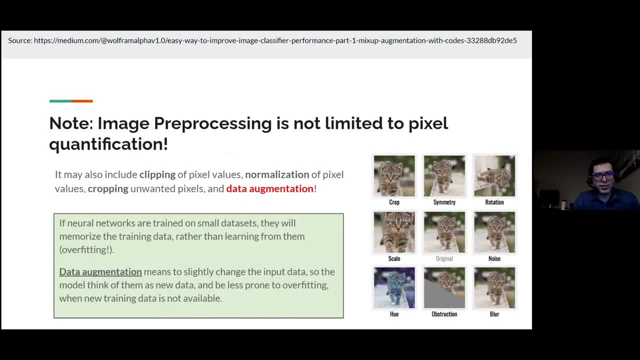 We expand our data set which, as I told you before, is not always feasible for us because we do not have too many patients in medical image right. So what we do as an alternative? you already have heard two alternatives from me. One was to create a synthetic data set using those image generation models. 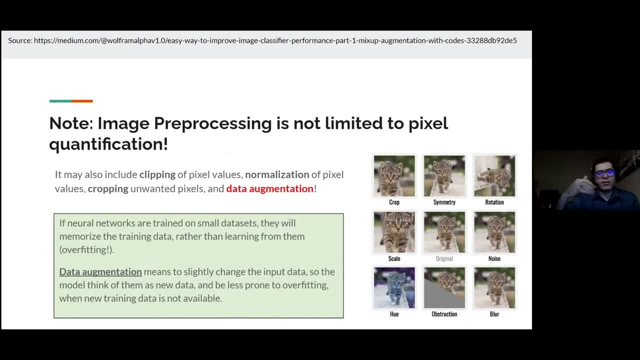 We can definitely do that, but that is super, super complicated, a very, a very complete project by itself. Something quite easier we can do is that we can rely on these programming interfaces. we have to, you know, somehow augment each of our images and feed them to the model as a new image. 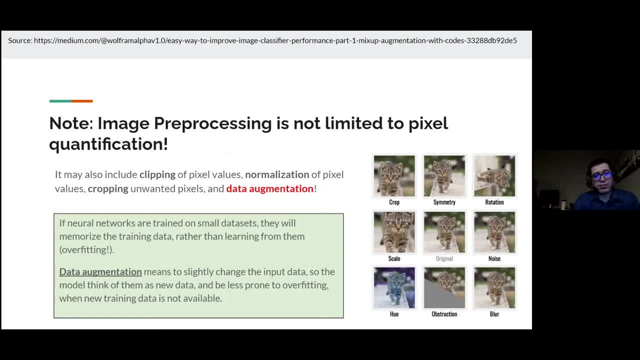 Of course, the model is not going to consider them as brand new images, you know, as as valuable as brand new images, but still this data augmentation is going to help our model to learn better. So by augmentation we can do a lot of things to these images. 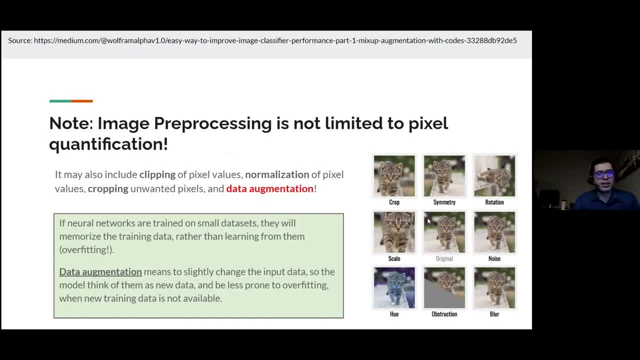 We can crop them. For example, this is the original image in this cat is in the middle row is actually the original image. We can crop a part of that image. We can, you know, flip that. We can rotate that. add some noise to it. 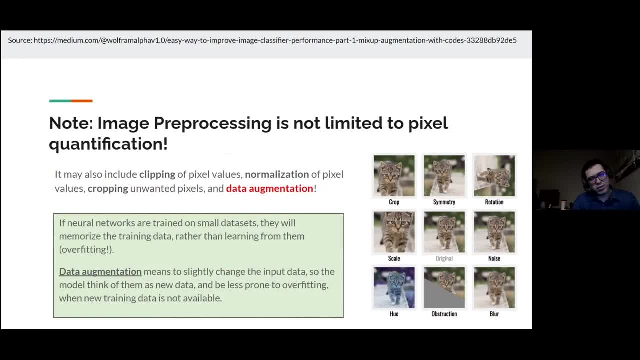 scale it, you know, change the color, whatever, So so you see, the model is going to still see the the same image, but a tweaked version of that, And we hope that by doing this the model has less chance for overfitting or less chance for memorizing data. 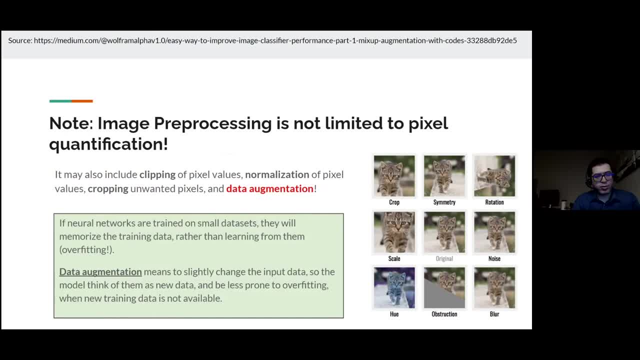 So just imagine that you know you have a very smart student and you are providing a piece of paper to him And then you want the student to understand the paper, not to memorize the paper, but they are quite prone to over to memorizing that because the student is a smart. 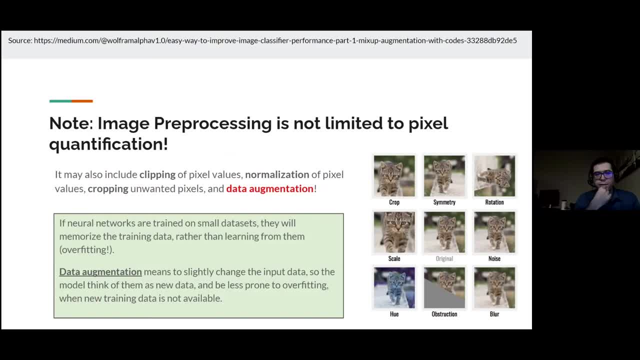 but at the same time lazy. So you just want to make that piece up, to make that portion of paper that you give to that student bigger. You don't, unfortunately have new pages, but you can copy the same page, flip that, rotate that. 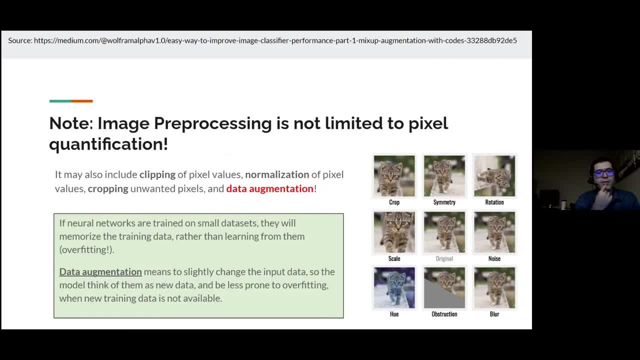 you know, put it upside down and tell the patient, tell the student that you know this is new data, this is new pages, right? So ultimately, the students will understand that this is the old data sold to him in different formats. 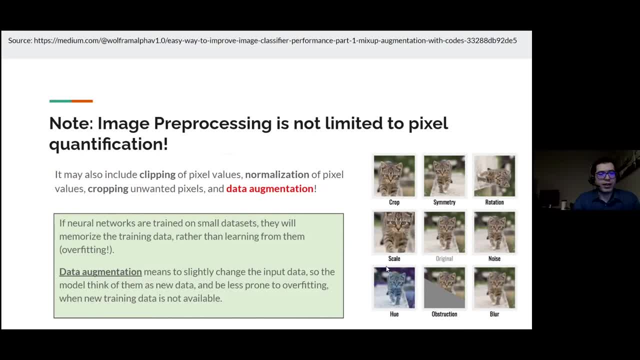 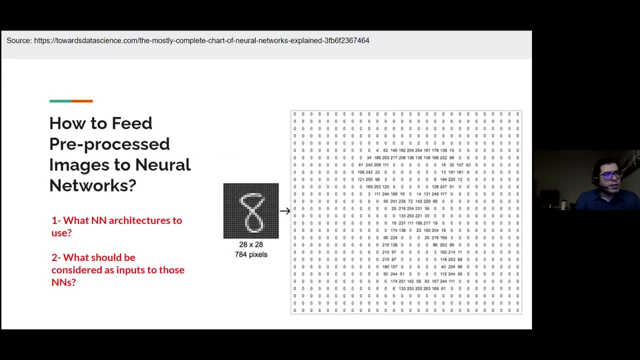 But I mean, hopefully he will finally realize that I'm going to learn rather than memorize this data. So this is an intuition for data augmentation of these models. Perfect Now. I'm going to now talk about the main business here, So how to feed the pre-processed images to neural networks. 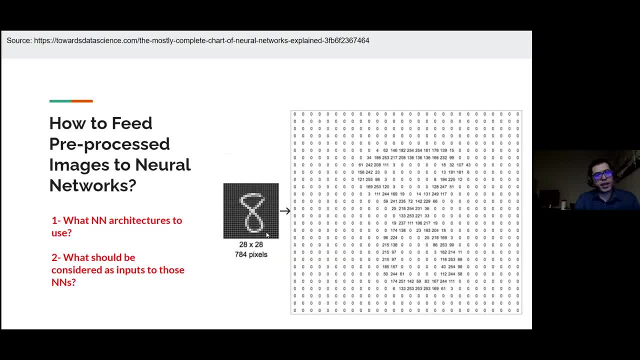 So you already heard from me that whenever we have an image from this eight, this is going to be converted to this very big matrix of values, all elements between zero and 255.. So two questions: What neural network architecture should be used for training a model on this? 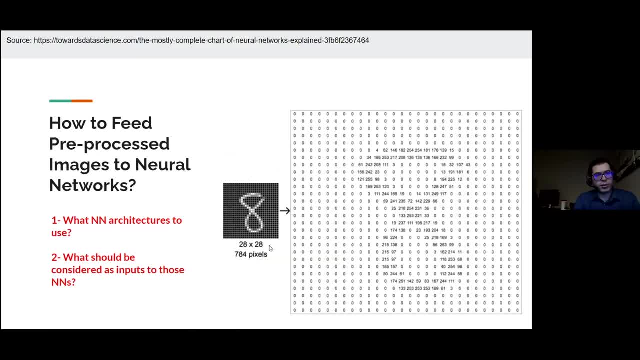 And this is not even a medical image, a very, very naive, 28 by 28 pixel. No medical natural image or gray scale image. And then the main question is: what should be considered as inputs to those neural networks? Should we consider the pixel values or something else? 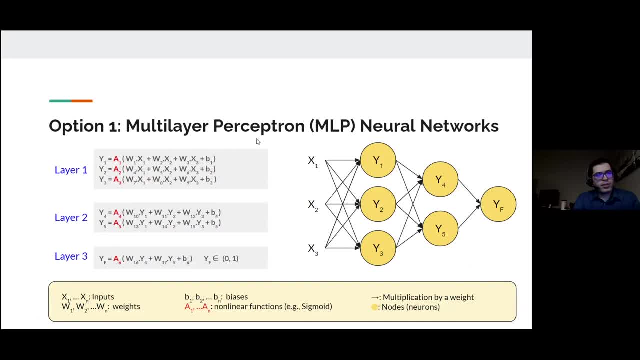 Let's proceed. So I am going to first talk about a specific kind of neural network. that is the simplest one And that is called multi-layer perceptron neural network, or sometimes they all they call it fully connected layers or fully connected neural networks. 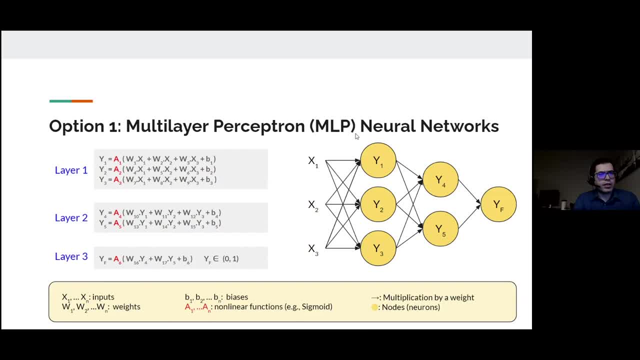 But no, multi-layer perceptron is a more accurate, but it's a much more complicated term And the way that these networks- I mean- work is quite similar to what we went through. So this slide is a repetition from my own slide set in the first workshop. 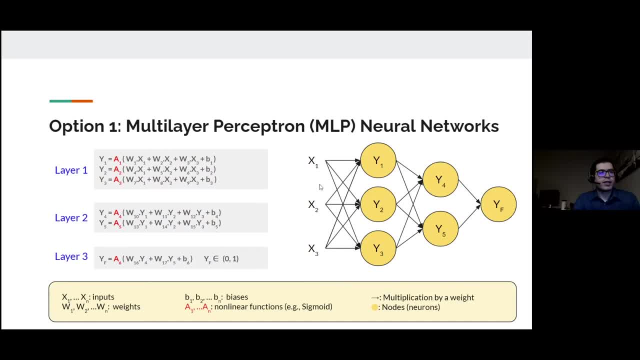 We already know about these things. I'm not going to repeat all the details there. You do remember that we had some sort of inputs here. three values. So this is a quite a simple network, simple MLP network. We have three input values. 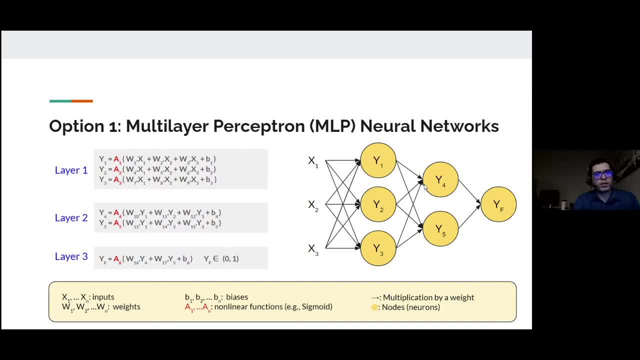 x1,, x2, x3, but we have a lot of parameters here. So y1, y2, y3, y4, and y5, are all parameters and they have parameters. If you see, the way that the final value yf is calculated is by going through all these equations one by one. 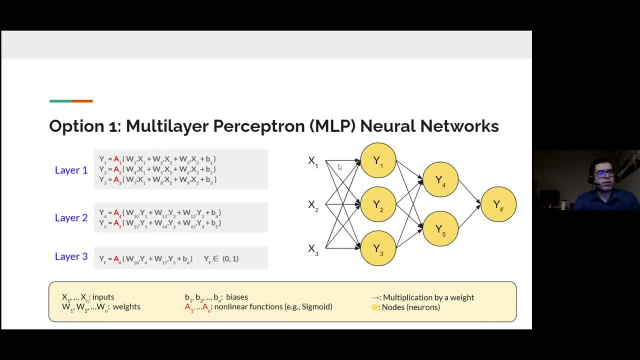 For example, node y1 here has is going to, you know, receive this kind of value here, which is actually made of multiplying different weights: weights from this node, weights from this node and weights from that node to different input values. 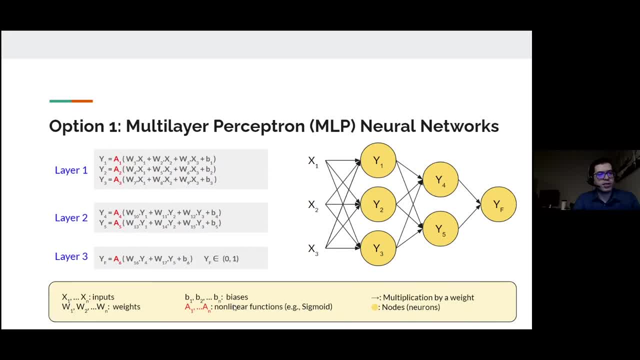 And then summing all together, we also had some sort of nonlinear functionalities here. I'm not going- I know that I'm not pausing and you know- talking in detail about this architecture, but I'm taking this as granted, as you probably have watched my previous presentation and know how this works. 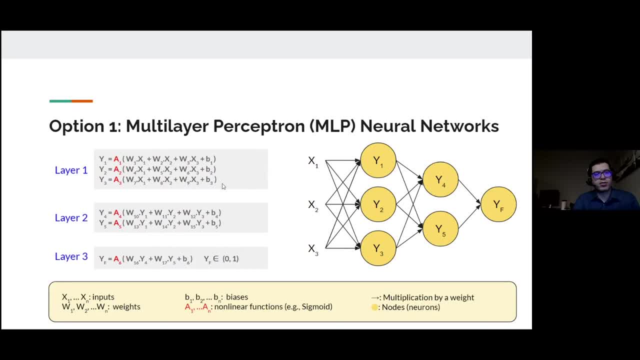 right, We had examples there and we spent about 45 minutes on these two images there in two slides there. So if you need to remind yourself of the details, you can feel free. I mean to watch that presentation, But anyway. so this is a very simple neural network model and 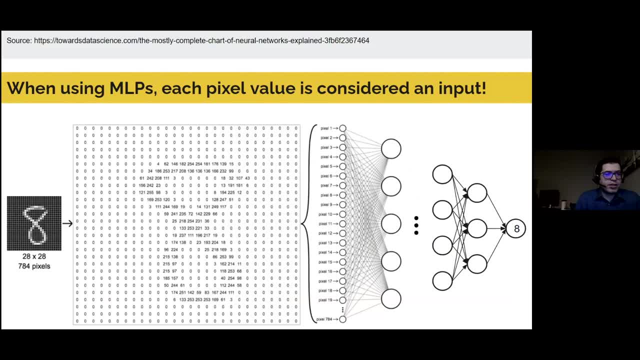 you know where, as a result of this simple architecture, one might say that, okay, if you're going to train a kind of classifier to say, as our previous example, classify or distinguish number eight from number two, we can say that: 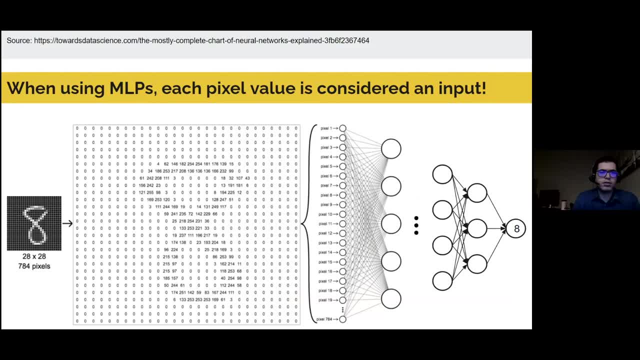 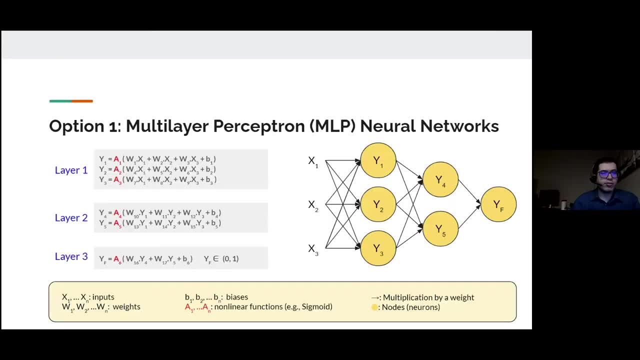 all right, we have this matrix of values and then we are going to consider each of these pixel values as a single input to our model. So you remember this one, this network here, had only three input values. Now we are talking about a very 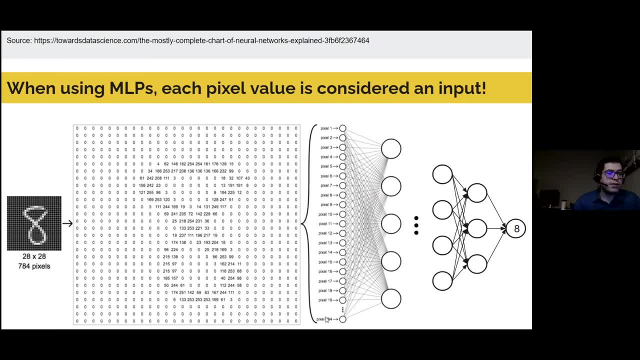 very big network here that has 784 input values, Right, And these values come from only a 28 by 28 pixel, which is quite a small pixel, right? Are you know normal images that we usually look at and they are high resolution. 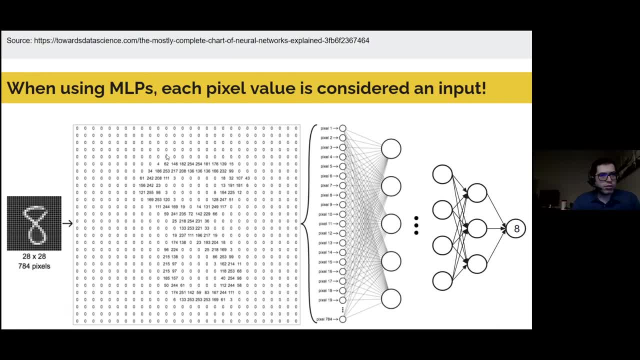 They are 1024 by 1024. So the numbers that could go there are really could be really bigger. But even for a 28 by 20 pixels we could fit all of those as input values to a neural network and then train this neural network. 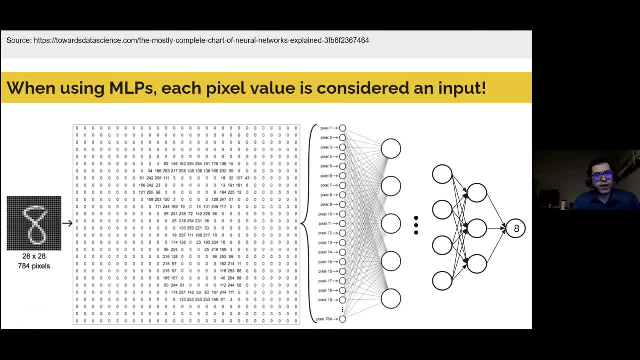 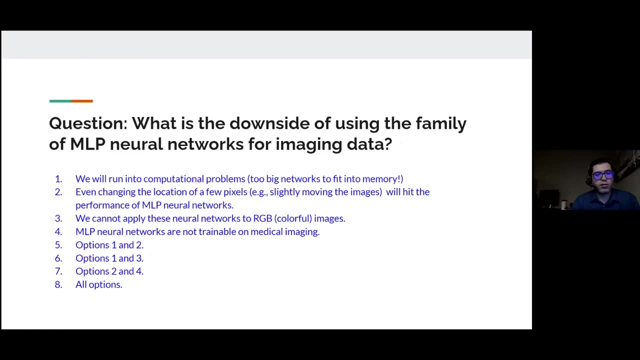 which had the MLP architecture And hopefully the final value is going to be predicted to be eight. So this was actually the baseline neural networks that people came up with And, to be honest, it worked. It worked until a checkpoint that people realize that we should somehow stop working with these MLP models on medical imaging. 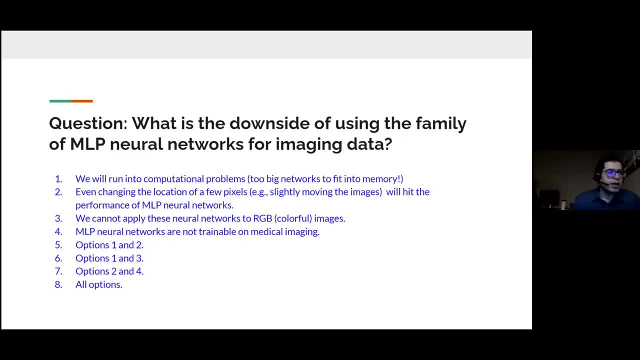 And I would like to give it a pause here for a couple of minutes. And no, I didn't find time to actually create a quiz for that, So put your answers in the chat box, please. What do you think is the downside, or are the downsides, of using this family of multilayer percent? 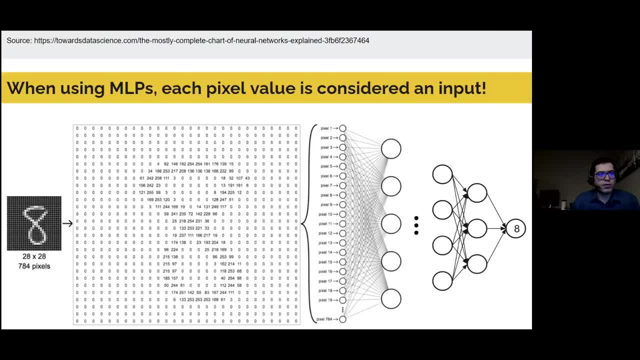 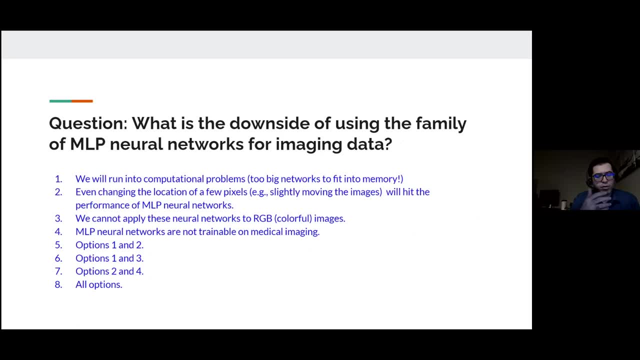 from neural networks for imaging data. So what I mean is that feeding each pixel value as an independent input to our model. what could be the problem with this approach? Do you have any guess? if one or two people want to share their answers, I would be happy to hear them. 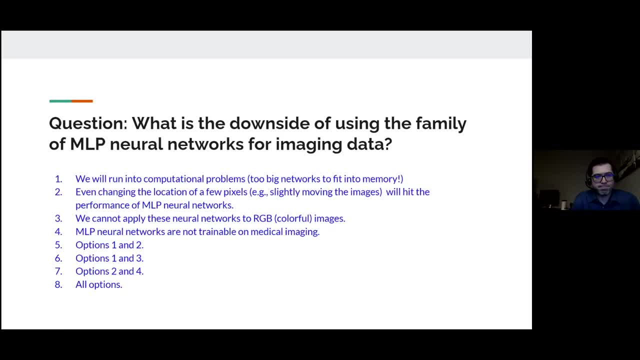 Otherwise, you can also put your answers in the chat box. I'm going to wait for a couple of minutes. Any guess, Was it difficult question to ask? Okay, Dr Wissendorf says five options: one and two. Okay. 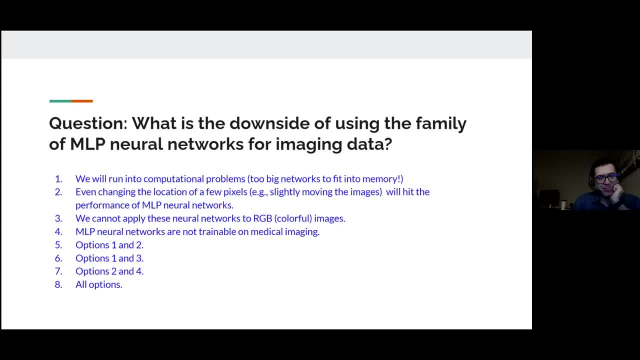 What else? Dr Wissendorf, it seems that you were the only one who dared to provide an answer. Everybody else is doing something else, I guess. so Omar says eight: All options. Okay, Five or six, Five or six. 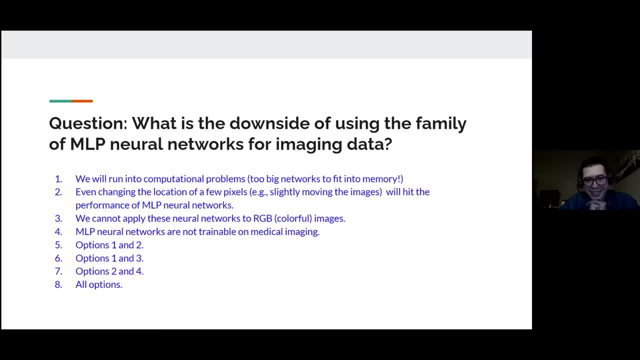 Now we go with some answers here. Okay, Good guesses. I go with five also. Five, All right, Good. And any intuition behind your answers? Does anyone want to share why you think like this? Okay, I'll consider that as guesses only. 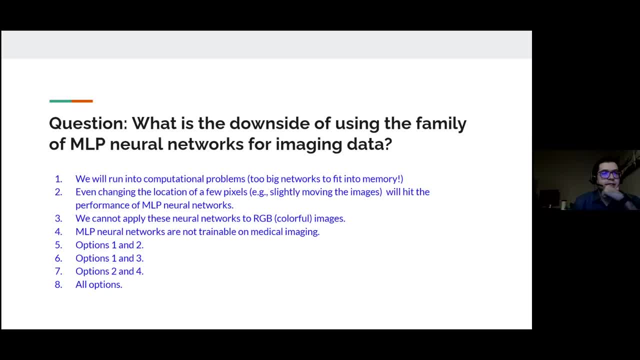 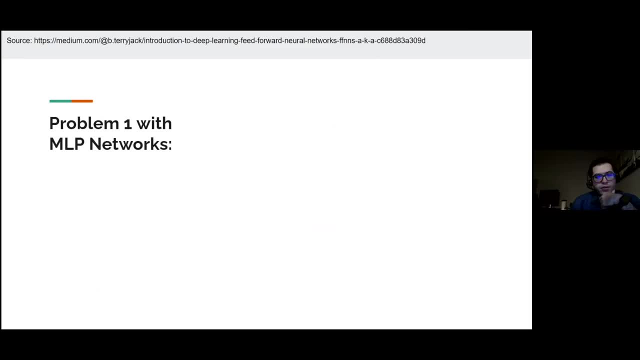 All right. So for the sake of time, I would like to proceed here and not take too much of your time, but only looking at this question. So there are two problems and Dr Wissendorf's answer, to be honest, was true. 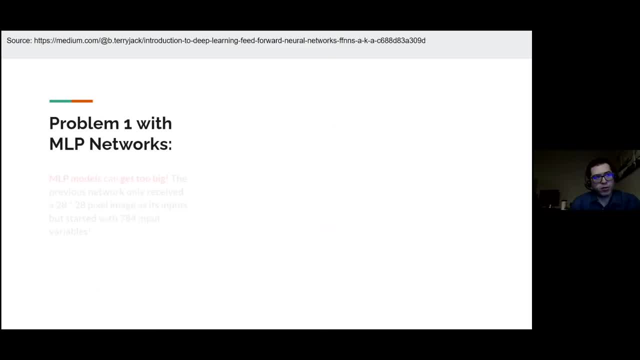 So there are two problems, two main problems with MLP networks. One is that MLP models can get too big. A previous network, the previous network we took a look at, only received 28 by 28 image as an input And it had 784 input variables. 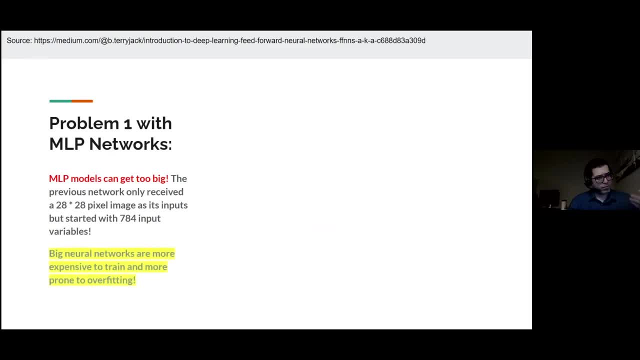 So this is something quite heavy for models And big neural networks, to be honest, are very expensive to train and they are very prone to overfitting. The reason is that the intuition of this is a little bit difficult to explain, but the 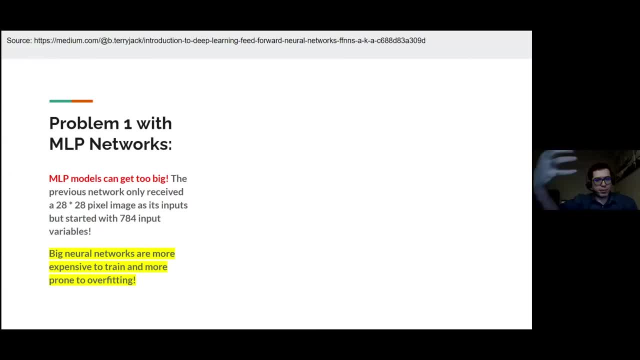 intuition is that? if so, just imagine as the number of parameters, as the size of the brain of that student. if you have a smarter student with a larger brain size and, at the same time, lazy as before, then it means that you need to provide more pages to them to somehow. 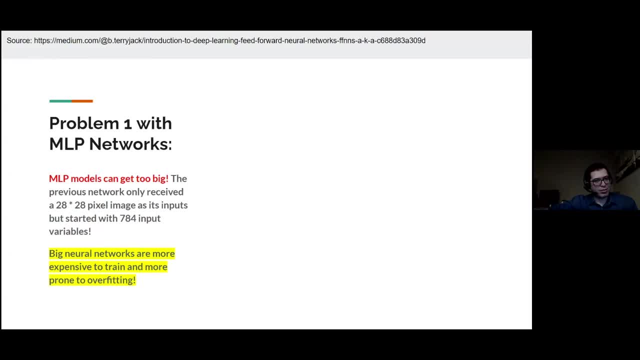 play with them, play tricks on them and say that this is something that you need to learn right. So smarter students tend to be more lazy and memorize concepts much, much more than a less smarter student. So it's good to keep neural networks architecture as small as we need. 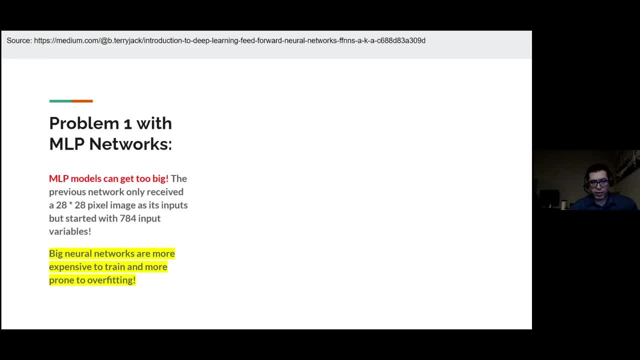 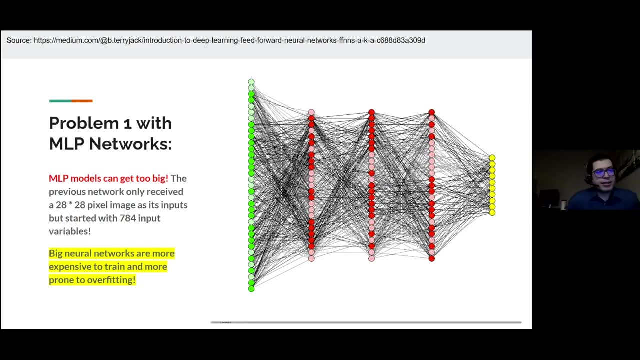 We need to make them big, but not too much big, because if we make them too much big, then they're going to overfit to our data. Now, the problem with this model is that, as you can see here, this is an example network. 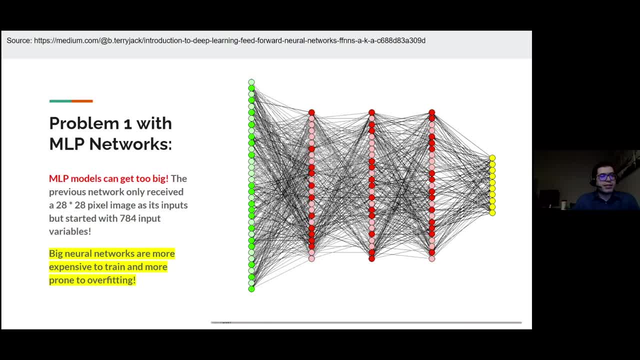 that has no less input variables than 784, but still you can see the number of operations that are going to happen behind the scene, and poor computer cannot handle all these. So if you're going to feed in a 1024 by 1024 image to your model, then you can possibly. 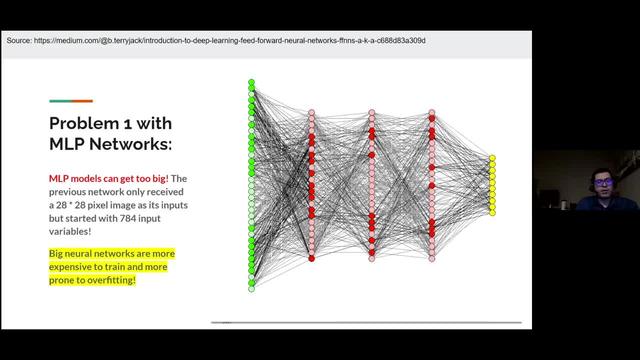 guess what is going to happen, how long it is going to take from the computer to actually predict your final prediction, Right? So, basically speaking, we rarely nowadays work with MLP network, And the reason one for that is that we understand that these models can get too big if we want. 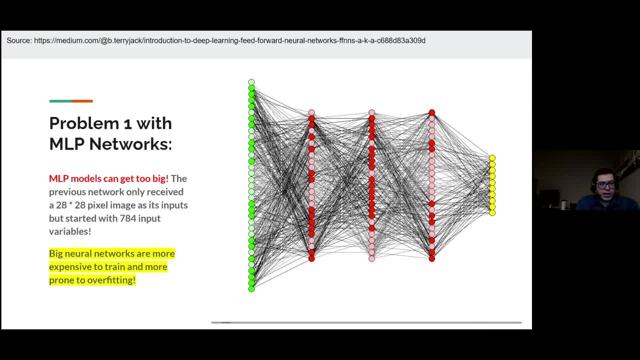 to make the input data a little bit complicated, which is actually almost always the case with real data, right? So these models can get very big. Now let's proceed from this fancy animation to another one, right? So we have a second problem with MLP neural networks. 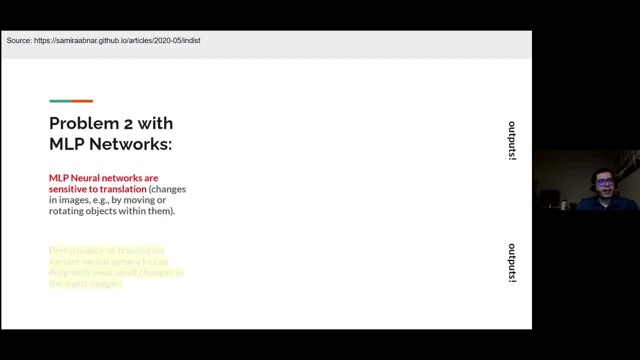 And this is that you know. they are sensitive to translation, which basically means that if you change, if you shift, you know, just imagine that you are shifting your entire image, one pixel to the right, one pixel to the right. So, or in a more generalizable experiment, here you are changing the location of this number. 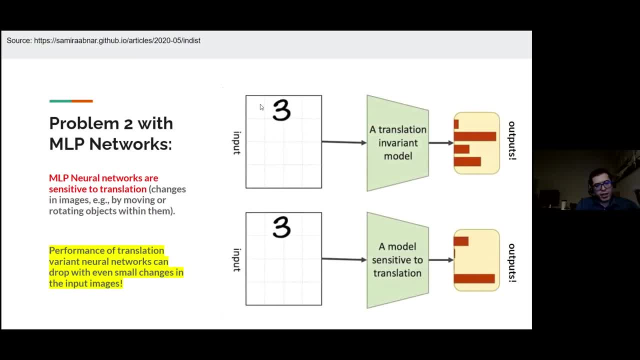 three in your image. Now an MLP neural network cannot realize that this is the same shape moving in the image field. It will say that, oh, even if you move that one pixel to the right or left side or top or bottom, it says that, wow, that is a new concept. 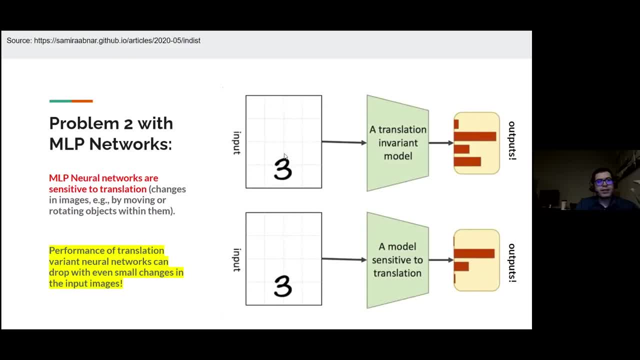 That is a new class, That is a new tree. MLP neural networks are not capable of understanding. things can be the same regardless of their actual location in the image. And this is a very huge problem because, you know, to be honest, we cannot really regard. 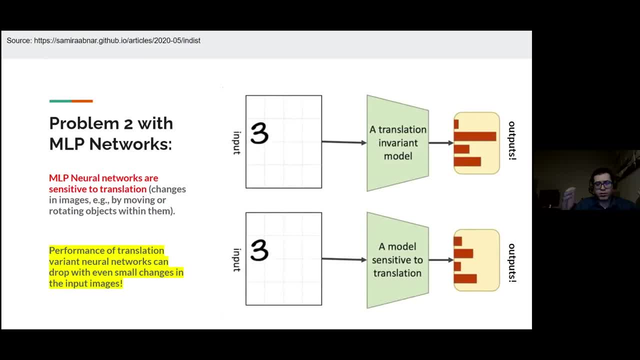 these kind of models to do some sort of real work. In old days, people tend to preprocess their models a lot. They tend to do a lot of cropping, for example, because this tree was always in the middle of the screen, in the middle of the image. 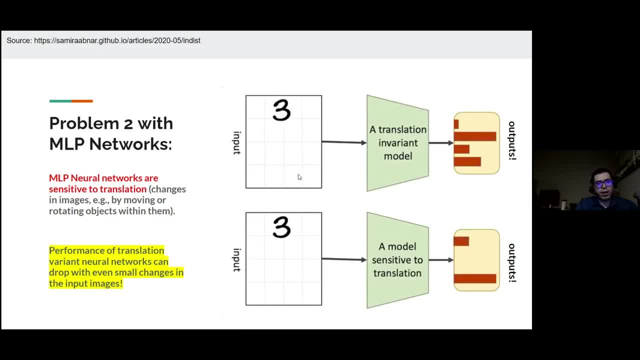 And now, when people wanted to really apply a model to realize what number is three or what number is eight, they did a lot of preprocessing to crop the images and put the tree exactly in the middle of the image, just for the sake of MLP models not to be confused. 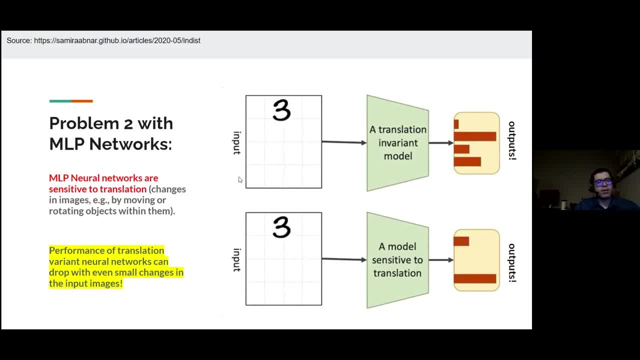 And this is a lot of waste of time and energy. So we've seen that We really didn't want to keep working with these translation invariant- sorry, translation invariant- or sensitive models. So we really want these models to not change their outputs when the position of the objects 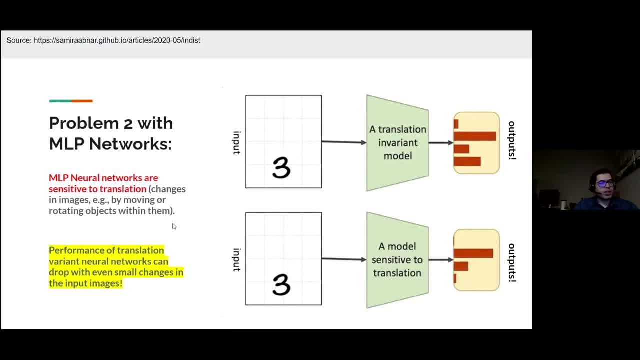 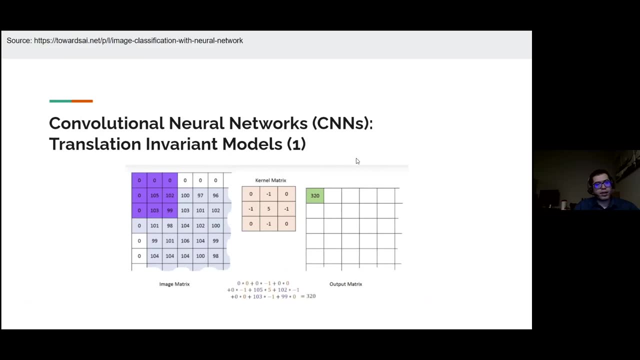 in the image changes. So we actually rely on these two big problems with MLP networks and then go through another class of neural networks that I'm going to introduce to you, and they are called convolutional neural networks. Now I'm going to go through eight or nine slides, one after the other, and this is the. 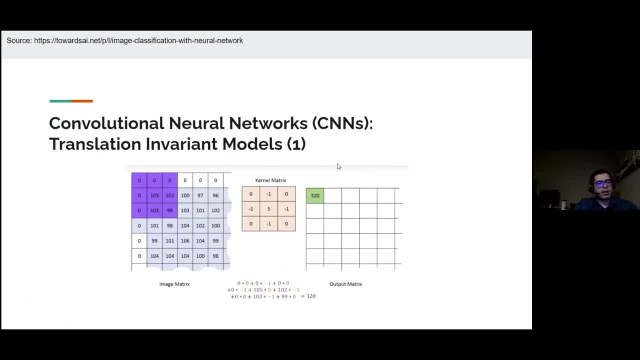 last part of the workshop, ignoring that last resources for further understanding that I am going to talk- And this is full of animations- You might have a little bit of difficulty understanding what is happening with the mathematical concept. I try to tell you as simple as possible, but if you didn't understand, it's just a matter. 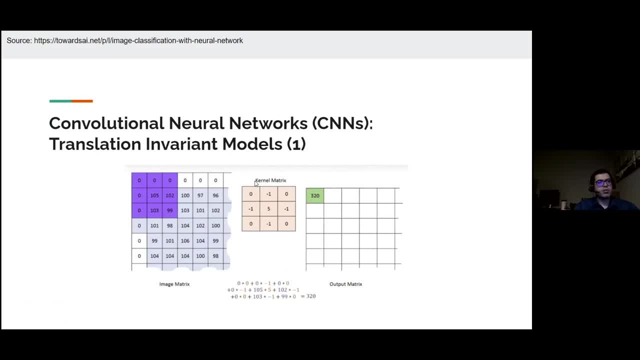 of Googling. We have a lot of good examples out there to help you understand, and those are quite written in easy language. So let's start. So let's start with the meaning of convolution itself. So convolution, in simple language, is a mathematical operation and the operation is super simple. 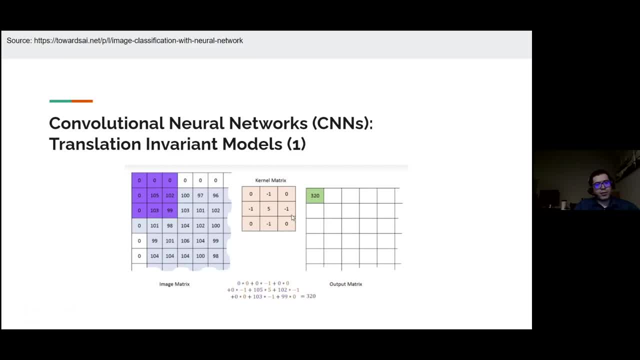 You have a matrix, you have a smaller matrix, and these smaller matrices are called kernels. right, At least for the purpose of this presentation, you could always regard these kernel matrices to be of size three by three. right, In real applications matrices, kernel matrices could have different sizes, but here we can. 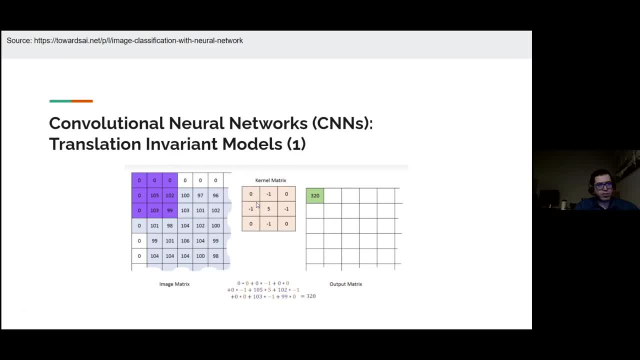 consider them to have only three by three shapes, right? So what you do is that you put this three by three matrix. you overlay that on the first part of your image, starting from the top left side of your image. right, You put it there. 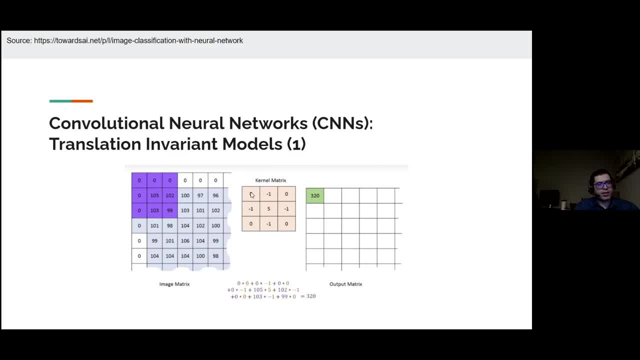 And you see that I am going to multiply each element of my kernel matrix to the same element, to the same position, element of my input matrix or image matrix, And the result is going to be my output value, the value that I'm going to put in my output. 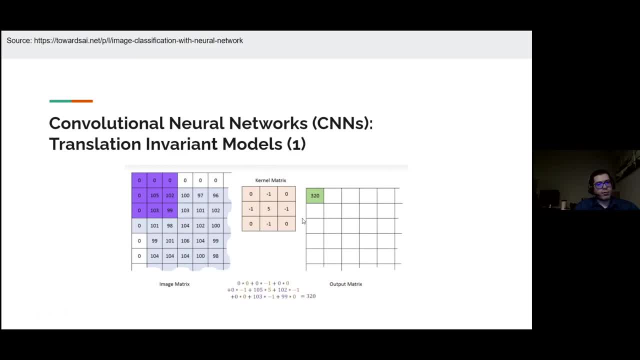 matrix. So, for example, here I am going to- oh sorry, I just made a mistake there, So I'm going to do that- And then I'm going to put each of these values here. So, for example, zero by zero minus one multiplied by zero, this goes to the second range. 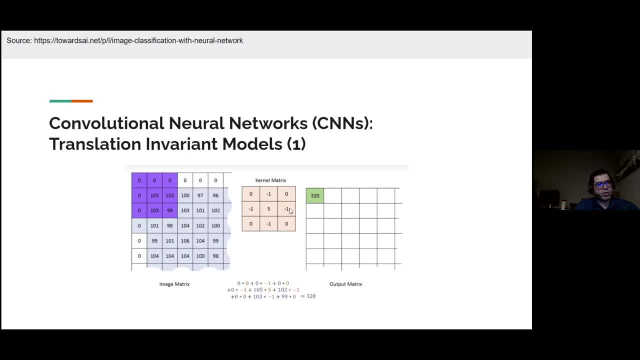 Zero multiplied by zero, this goes to the third value. And you do this for all the nine values. And what I made a mistake about was that you are not going to add all these intermediate values together, add up them together. So first you are going to sum all these nine different values that were made by multiplying. 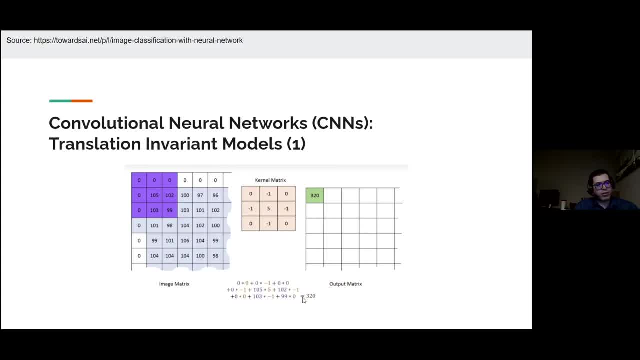 elements once per years And the result is going to be 320.. The result is going to be put into this output matrix. So you could see that by applying this three by three matrix on this first three by three placeholder of the image, We are going to have. 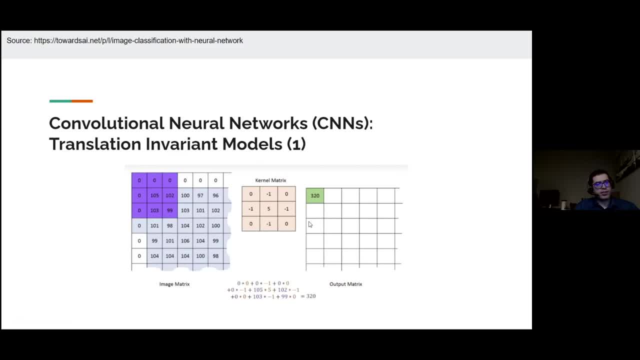 We are going to have a number there. So for this slide, I just want you to understand the meaning of kernel matrix and the convolutional operation. So this is actually a convolution. What we did there was running a convolutional operation, which means that we had a kernel. 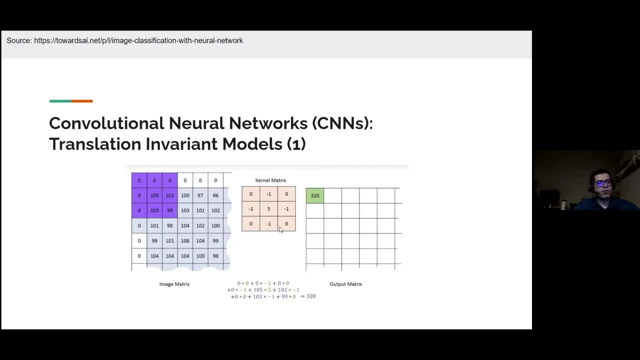 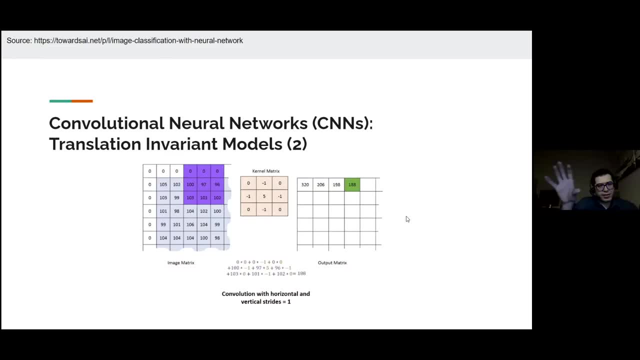 matrix. We applied that on an input matrix and we got an output value. So let's take a look at an animation of that and see how this happens in the future. So this kernel matrix keeps moving onto your original image. We move that. 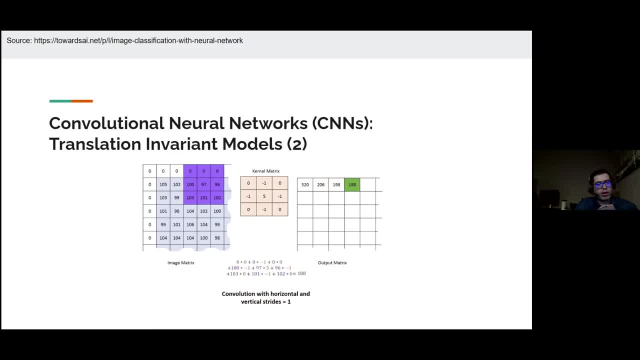 We shift that, We shift that, We shift that And we do this till we actually overlay the kernel matrix on the entire regions of the input image. And you see that whenever- I mean each time- that we overlay the kernel matrix, we do the. 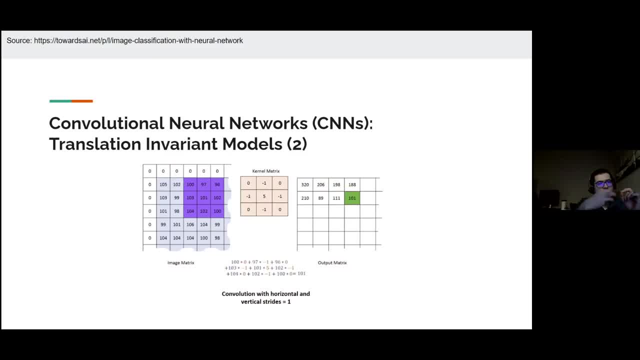 convolutional operation and we get one final output value And this is how we actually create our output matrix, Right? So you can imagine that, given an image matrix and a kernel matrix, and forget about the size variability and how they should be matched with each other. 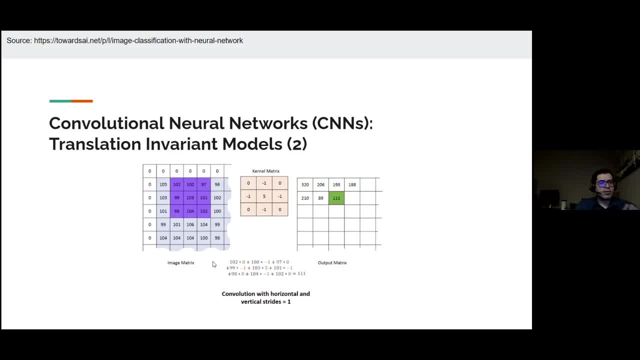 Forget about that for a second. But you just see that You know an image matrix as an input and a kernel matrix as an input can come together to this output matrix that is created Right? This is how the convolutional neural networks are actually work. 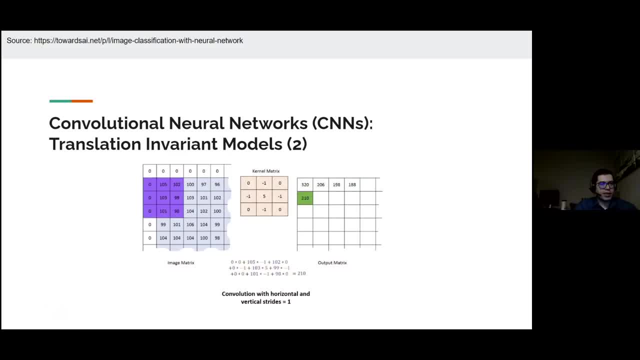 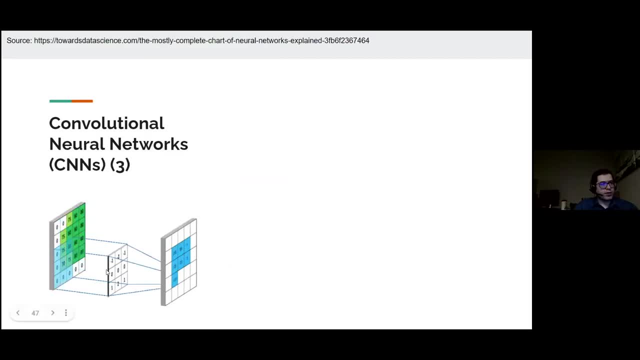 They are based on this convolutional operation, which is actually a very simple mathematical operation. All right, Now let's look at this one. This is another view of the same operation that we talked about And I'm going to now. I mean based on this concept that we went through introduce CNN. 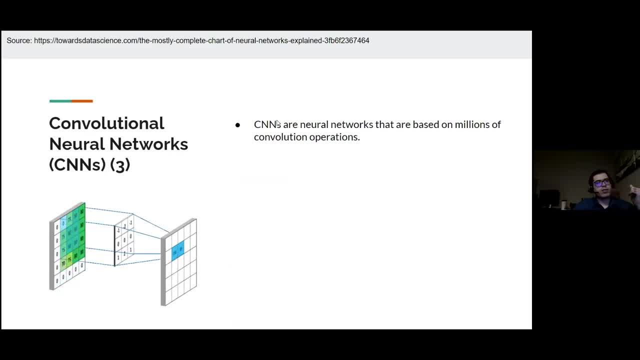 or convolutional neural networks. So CNN means convolutional neural network. Almost everybody in data science world use this term CNN Convolutional networks are too much long to pronounce, So I'm going to use the same term here as well. So CNNs are neural networks that are based on millions of convolution operations. 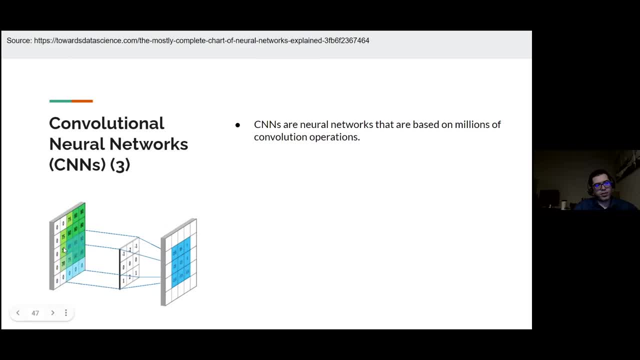 You are just seeing one. I mean five or six convolution operations here. But in real practice, in real neural networks, we are going to work with millions of CNN operations Now. in each convolutional operation a kernel matrix which is usually three by three, as 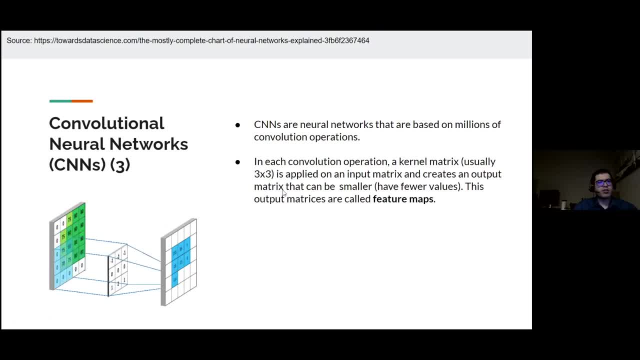 I said before, is applied on an input matrix and creates an output matrix that can be a smaller, have fewer value. So look at here. You see that when the kernel matrix goes through all these parameters, all right, you are going to have a final output matrix that is a little bit smaller than this input matrix. 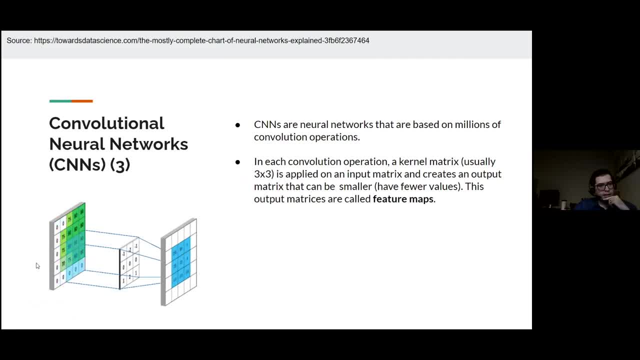 Now, what I'm saying here is not always true. in real deep learning, Right, We can trick these kernel operations to generate output matrices with the same size as the input matrix. But for the sake of this presentation, let's assume that these convolutional operations 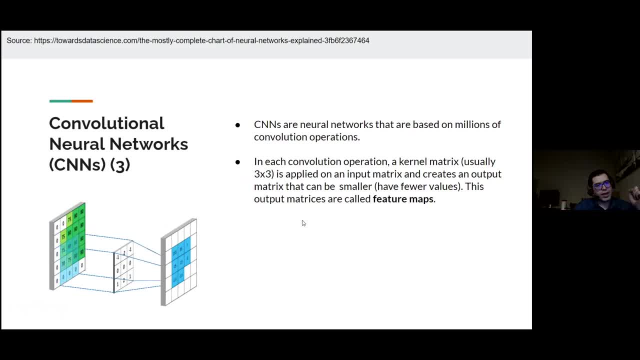 always result in a smaller output matrices. Right, And this output matrix, to be honest, has a fancy name: We call that a feature map. So whenever you have an input matrix, you apply a kernel matrix to that using convolutional operations. 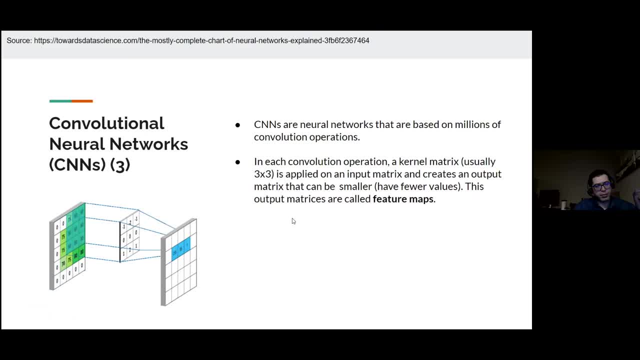 You are going to have an output matrix that is called a feature map, And the reason we call that this way you're going to see very soon. Right Now in CNN's convolutional operations are built on top of each other. That means each output feature map, like this one now, is going to be the input feature map. 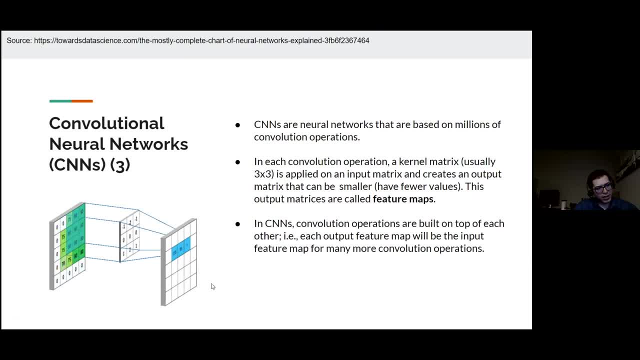 for many more convolutional operations, which basically means that another kernel is going to be applied on this image Right. And this is how we actually use all the pixel values of an image Right. Imagine that you have 512 by 512 images as inputs. 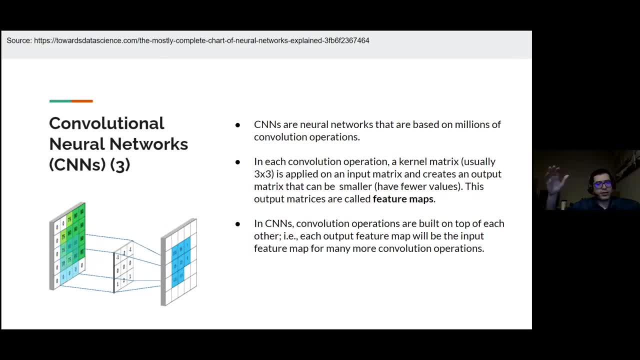 You are going to overlay kernels on them, And maybe after the first round the output feature map is going to be, let's say, 480 by 480 pixels. In the second round you apply another set of convolutions and then you will have an. 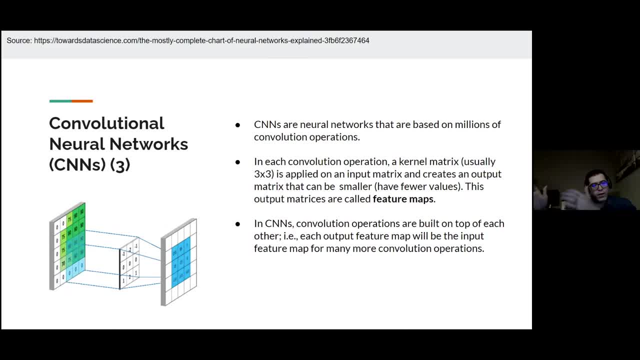 output feature map that is smaller, And you keep doing that, keep doing that. Finally, you may come up with, you know, maybe an output feature map of three by three, something like that, Right, Something that, as you see here, 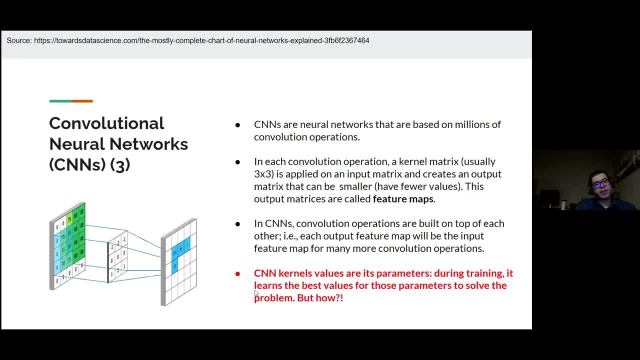 And the important point is this: So the fundamental difference between MLPs and CNNs is that, in CNNs, the parameters of the model, those parameters that we wanted to learn, those parameters that we took, the gradients of loss with respect to them, are actually these values of the kernels. 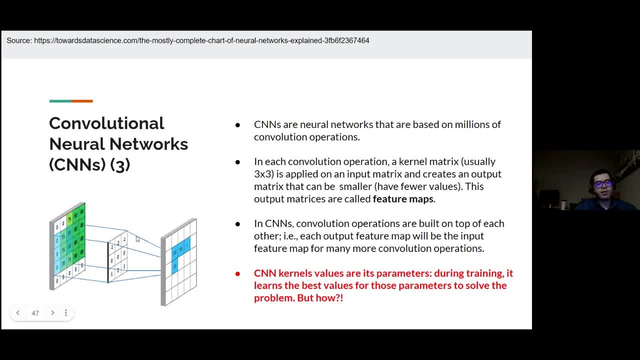 So you see this: minus one, minus two, minus one zero. So these are the parameter values. So the number of parameters of a CNN is actually the number of values existing in different kernels that that model has Right. So whenever we are training a CNN, we are actually looking for the best set of numbers. 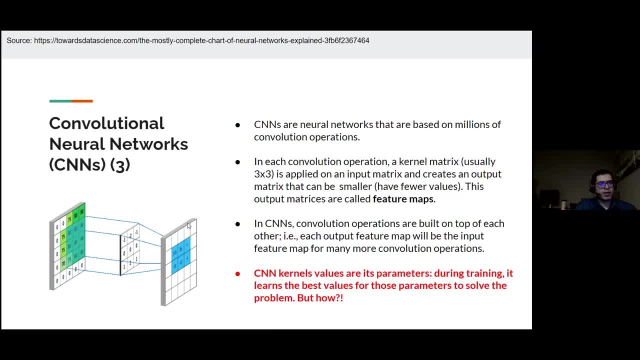 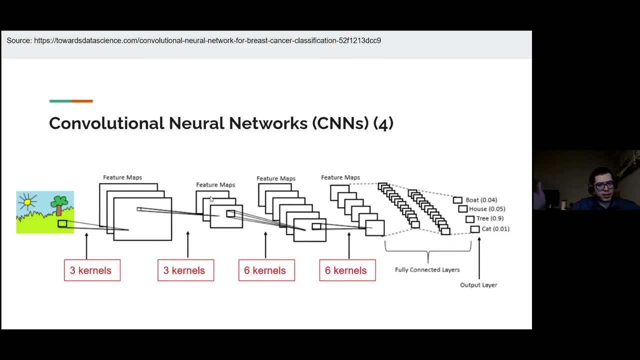 for these kernel values. So this might not make that much sense to you at the moment, but let me proceed and you will probably understand better Now. let me first give you a big picture of what is happening here. So this is exactly what I told you. 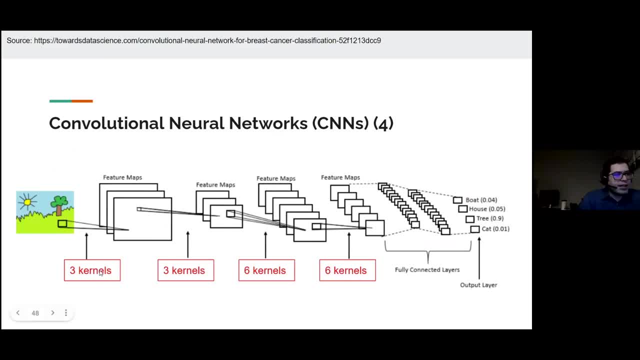 We have an input image, For example. let's say that we apply three different kernels to those. So three different kernels. Each kernel has an input, Each kernel has a different kind of value. So three different, three by three matrices, And each of those kernels is going to create a feature map or an output matrix for us. 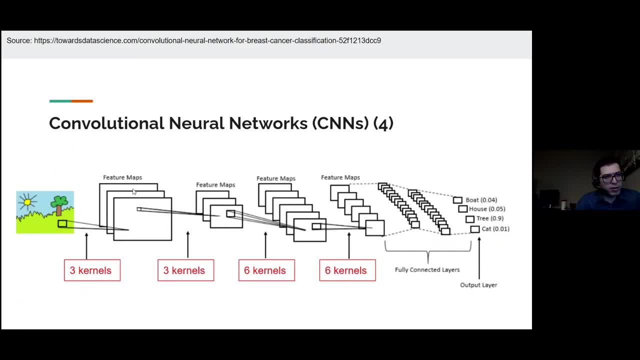 As far as we had three kernels, we are going to have three output feature maps, And now we may add each of these three feature maps to another set of kernels. So three new kernels come here Right Now. you might wonder: why didn't this result in nine feature maps? 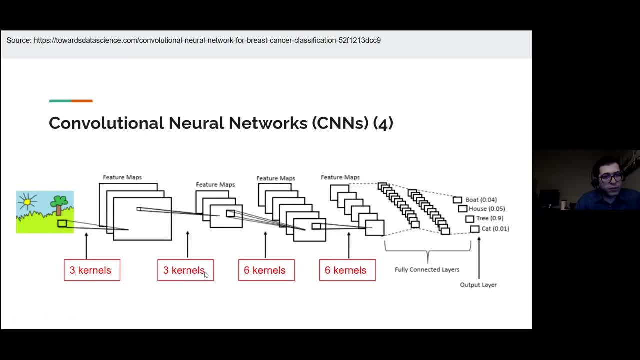 Three input feature maps, three kernels. This should be nine output feature maps, right? So this is the trick here. Convolutional neural networks don't work that easy. They somehow. so each kernel, each new kernel, applies itself on each of these input feature maps. 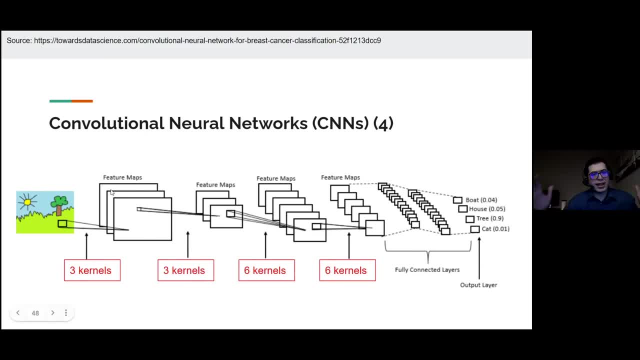 But the final values for each of these feature maps are actually stacked on top of each other, So they are summed together. So for each kernel, for example, if this value is one, this value is two, this value is three. So suppose that I am going to, you know, apply a kernel that has value two on the equivalent value of its size. 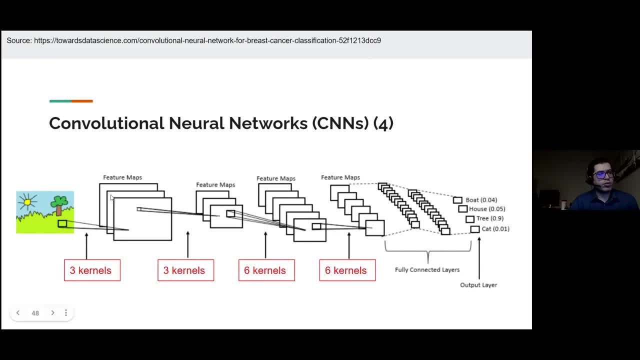 So this is going to be now: one multiplied by two equals to two, Two multiplied by two equals to four, And three multiplied by two equals to six. So we have now values two, four, six. The way that convolutional neural networks work in practice is that they sum these values together. 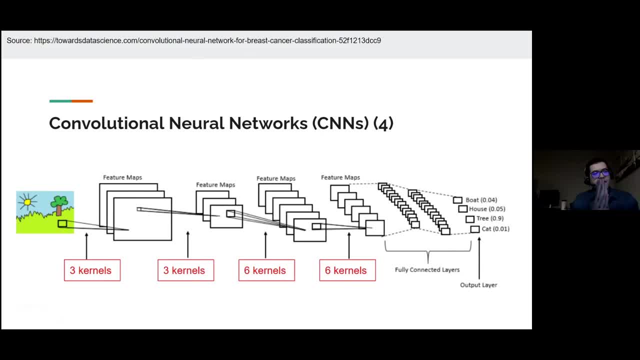 So they actually overlay, overlap these. you know, three generated feature maps on top of each other. Sum their values and say that now this is going to be my main feature map. This is going to be ten, for example. If you didn't understand this part that I mentioned, just ignore that. 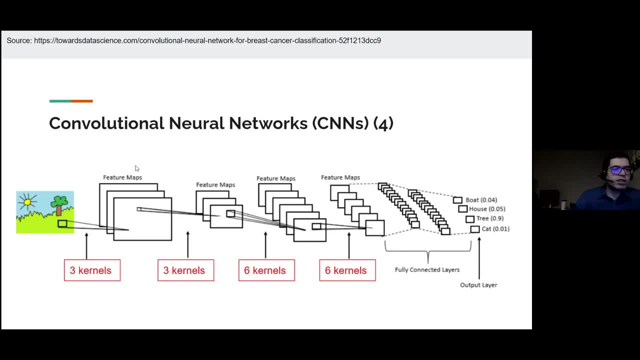 I mean, this is not important for understanding neural networks. What I really want you to understand is that you know convolutional neural networks are kernel operations. They work on each other's output and consider those intermediate outputs as inputs for each other. right, 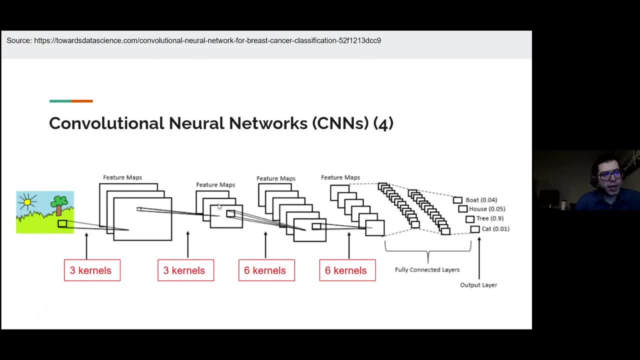 So, for example, these six kernels here work on these feature maps as their inputs and then create new feature maps, right? And we continue this pipeline until the very end when we now play the role of these MLP layers. So these fully connected layers, as I told you, are fancy names for multi-layer perceptron. 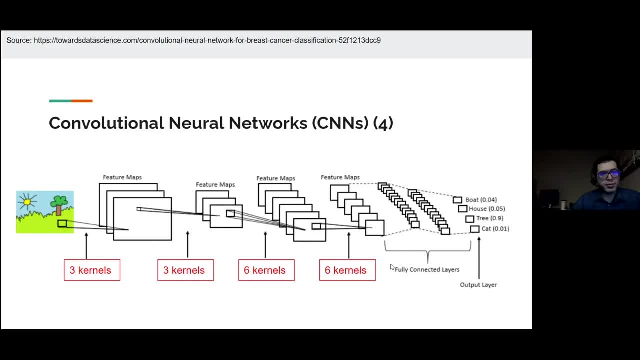 Those simple neural networks that, if you remember, I told you had a lot of problems. They have a problem, They have huge problems, But we can still use them on top of convolutional neural networks. So convolutional neural networks have a lot of convolutions. 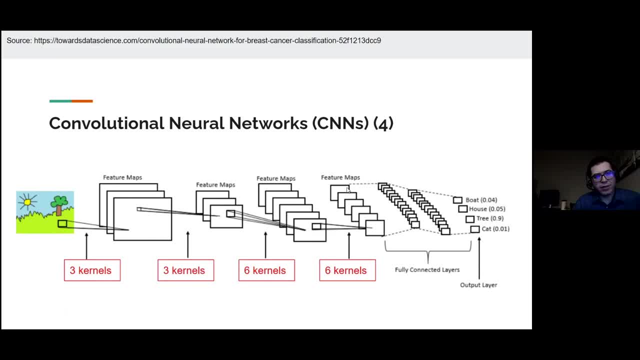 But usually at the end they finally. So the values of these final, The values of these final feature maps are now fed through, you know, some fully connected layers, the way that we fed that eight image pixel values to that MLP layer. So this is going to be something again very simple here. 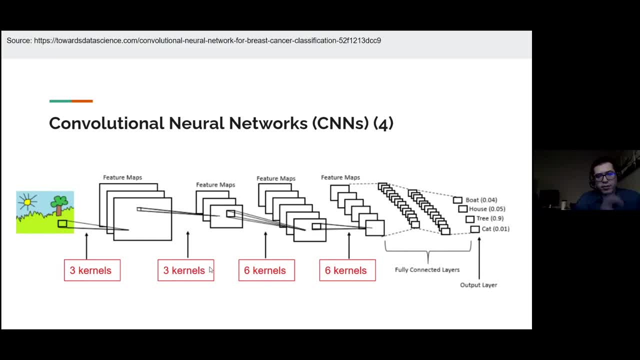 And this is the big pipeline. So do you understand this image here for now? Because for now we have covered almost the main part of the convolutional neural network. I have more fancy animations to share with you, but the main concept is what I just told you. 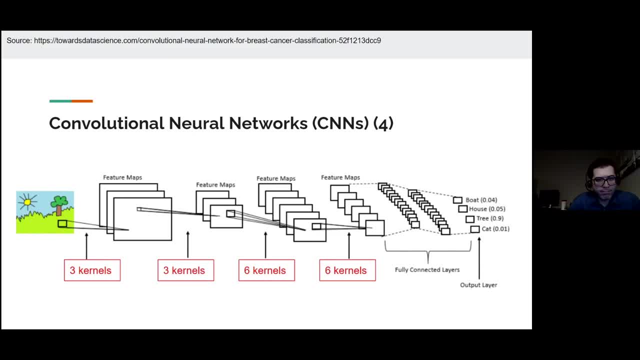 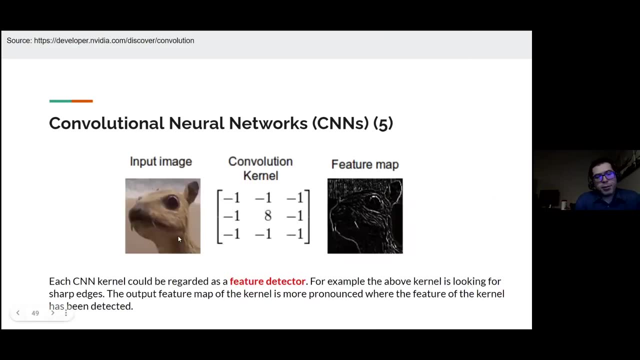 Any questions about these convolutions? Okay, I take it as a good sign and proceed to show you more animations, But then we probably can come back to questions again. All right, So let me now give you an intuition. So we went through the mathematical meaning of applying a convolution operation. 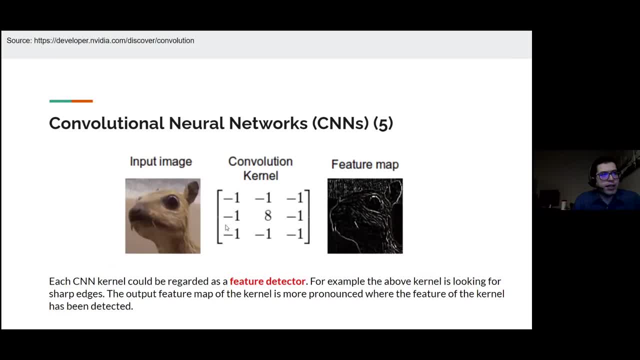 I would like to give you an intuition of what these operations mean. Each convolution kernel is actually searching an image for a specific feature, And for this reason these kernels are also called feature detectors. And now you understand why we call this output matrix coming out of a convolutional operation a feature map. 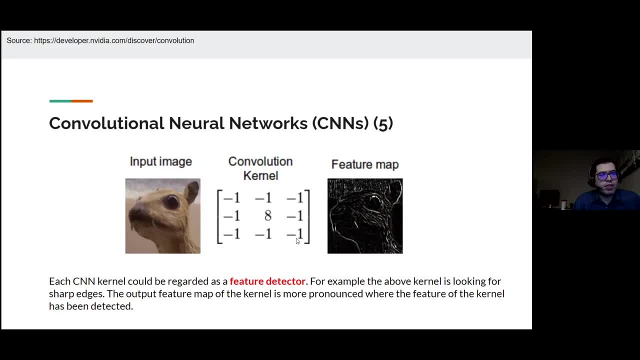 Now, this specific kernel that I put here is actually, for example, looking for sharp edges. Now, these values that I put here, this output feature map is not, if you look at that it is. it has very high values which are, you know, not very high values. 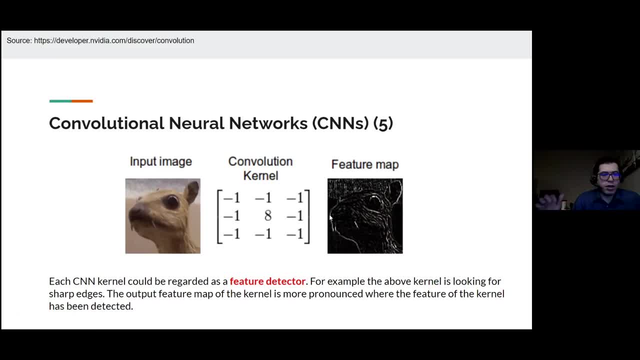 It is very high values, which are, you know, near to white, because, as I told you, values are. if values are higher, then the visualization is going to be more white, right? So if you look at where had been highlighted on this image, they are exactly the edge areas of this camel right. 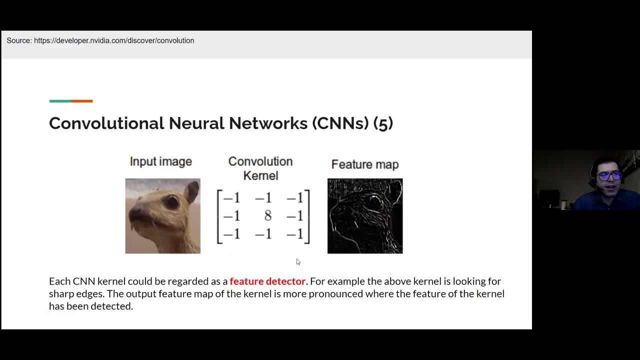 So, basically, this kernel specifically was designed to pick the, you know, the sharp edges of the images, of the input images, And that's why you see here, sharp edges are actually highlighted in this image. Now you might say: how do we know that this is specific convolution? 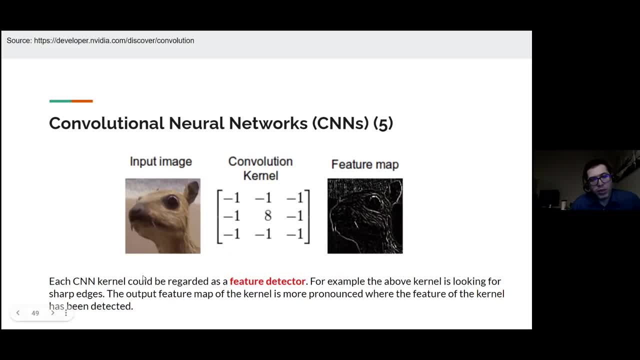 How do we know that this kernel could detect sharp edges? Well, people have spent a lot of days in image processing- you know literature- and they came up with different kernels And they understood what kernel could pick, for example, sharp edges. what kernel could pick angles, what kernels could pick- I don't know- for example, circles. 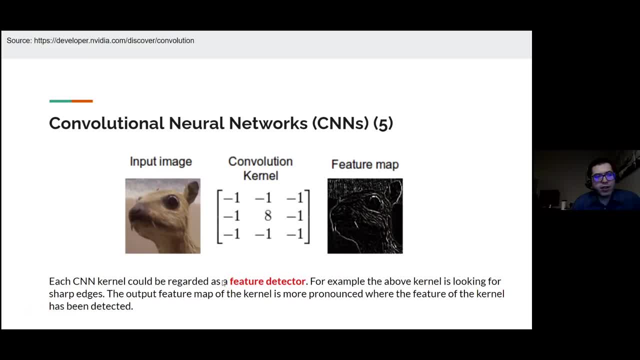 So we do have kernels for specific features that we are interested in, And by features I mean things like edge angle- you know small tiny things in images or things like that. So you see here that this kernel- specific kernel here- is actually detecting sharp edge and then generated this feature map for us. 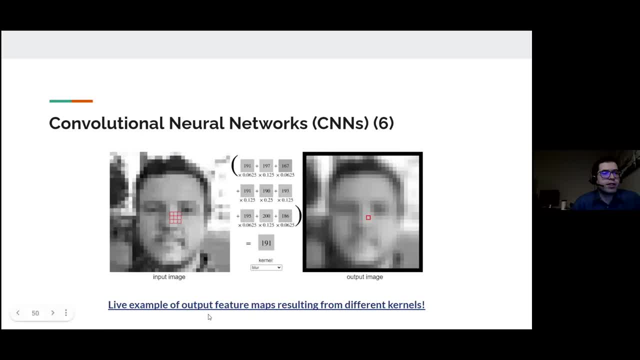 And let's look at another example. So this was a live example that I guess we do not have time to watch now, but the link is here. So go there and try to play with this value of the kernels and see how changing of these kernel values could result in different feature maps. 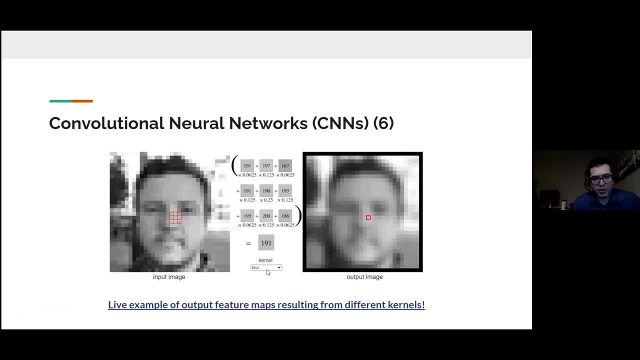 So this one, for example, is a kernel for blurring an image. It's really interesting, right? So you just apply a kernel to an image, Right, And you make it blurred. So this is how image processing works, right? 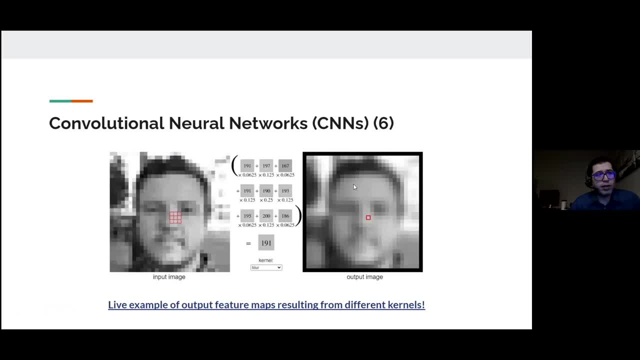 Even applications like Photoshop, if you want them to blur a part for you. what they do behind the scene is that they usually apply a kernel- pre-specified kernels- to your images And this is how they know what kernels work the best for blurring, what kernels work the best for making it sharper, and things like that. right. 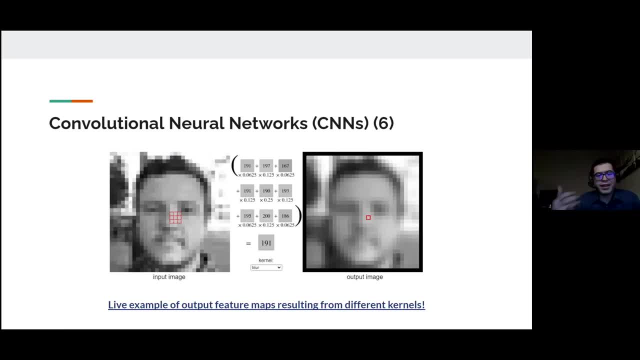 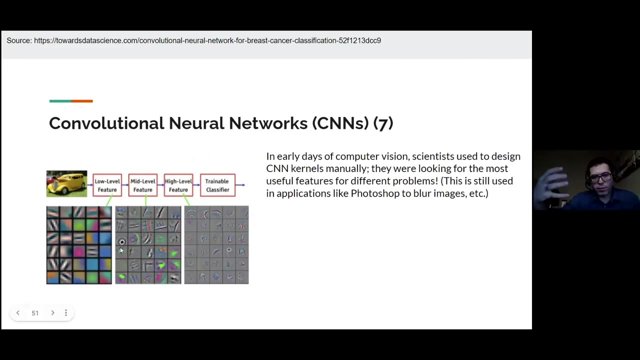 Increasing the contrast, decreasing the contrast. So kernels can have meaning. This is what I want you to know. Kernels can have meaning. These are not random values multiplied to each other. Now things get even more interesting because, as I told you, convolutional operations are applied to previous operations' outputs. right? 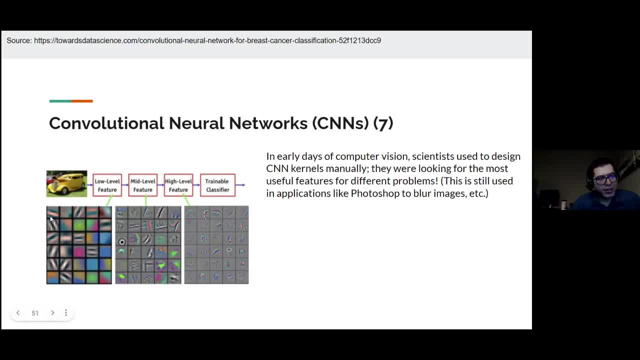 So basically, the first operation detects some features for you And now a second operation is going to receive these input features, as it's another new set of inputs, and create new features, newer features for you. So we have low-level features And then these features are actually fed through newer features. 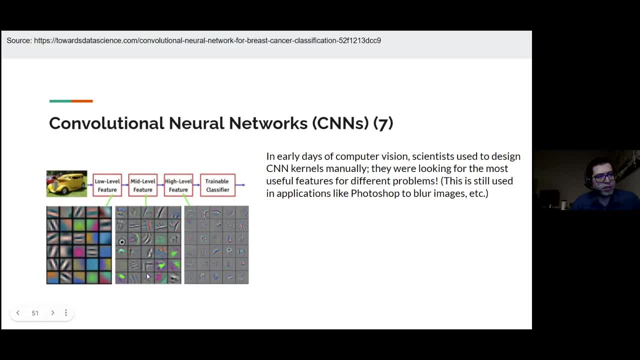 These are actually fed through new convolutional operations, And then they generate these mid-level features, And then they are again fed through high-level kernels, And by high-level I mean that those kernels are down the line right. Those are actually applied at the end of the pipeline. 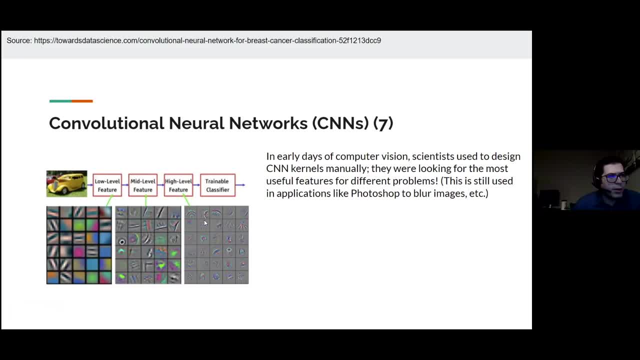 And then they create these different type of features. And now, if you ask yourself, how are these features different from each other? you'll probably notice that you know, the low-level features are exactly those simple features I introduced in the beginning of this part. 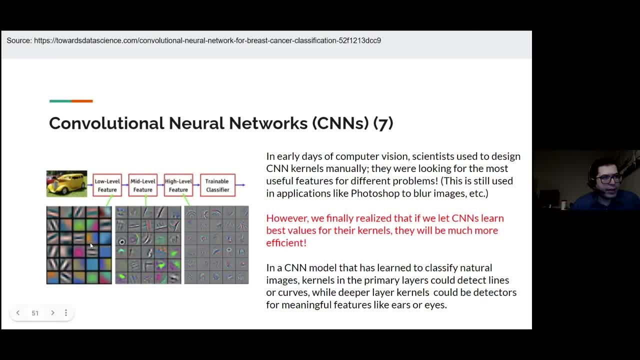 I told you that those can detect lines, Angles, Circles, But what about the mid-level and high-level features? It seems that they are now detecting meaningful things like the eye. Do you see the eye here? Or maybe a flower here? 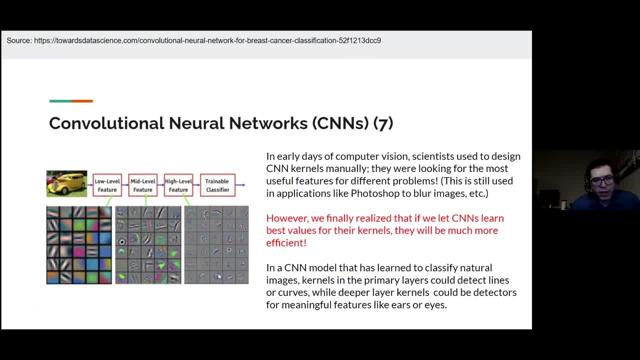 I'm not quite sure, Or maybe something like a sun here. Basically, the final kernels of convolutional neural networks, if trained appropriately, are going to be detecting those features that do have meaning and are definitely important for your task that you're working on. 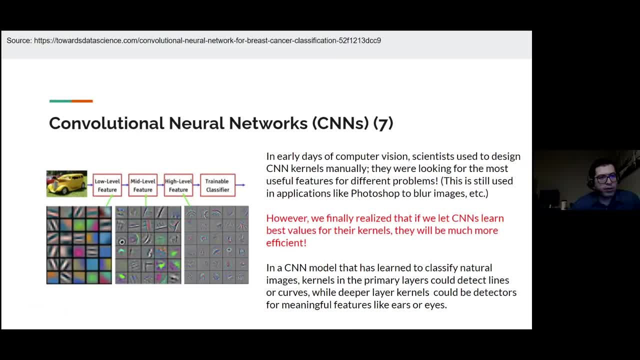 So, for example, if you're training your model to distinguish 8 from 2, the final features of your convolutional neural networks could be something like a sketch of an 8-digit or a sketch of a 2-digit. And what happens there is that now the final network, the final layers, the final convolutional operations are going to understand whether or not features similar to these, or at least a little bit close to these- you know features- are going to be detected. 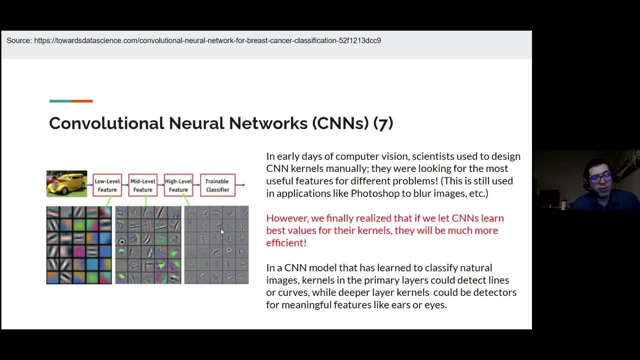 And you know, despite- I mean as opposed to MLPs- these are not now sensitive to the real location of the images. Now, the reason they are not sensitive is actually because of the convolution itself and how the convolution moves into the images. 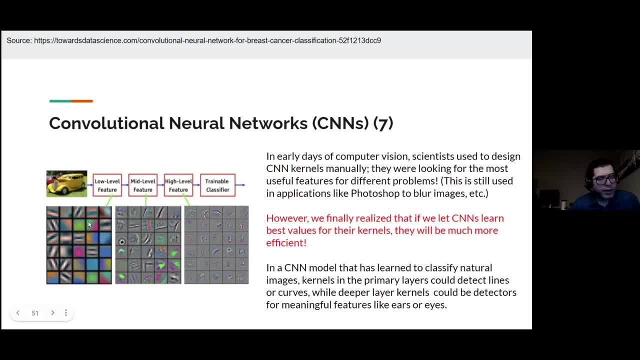 You might not understand this as I say like that, but try to think about that. Convolutions go through the entire image And the entire image for different features. So if I have a kernel for detecting lines, that kernel is going to detect the lines regardless of where that line is in my input image. 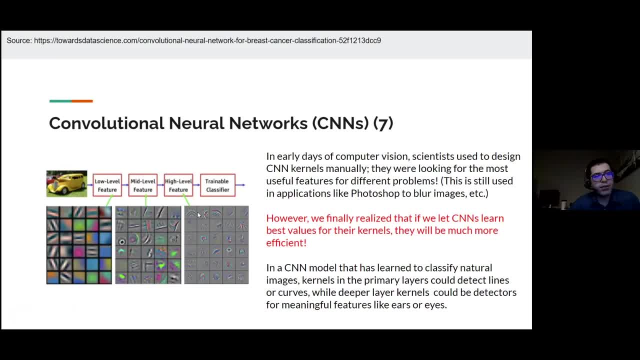 And now, on top of that, if my kernel is looking for eyes, that kernel is going to find an eye into my image, regardless of where the eye is. So if I change the location of 3-digit in my previous slide, if you remember, within the image the convolutional neural network is still capable of saying that it is a tree. 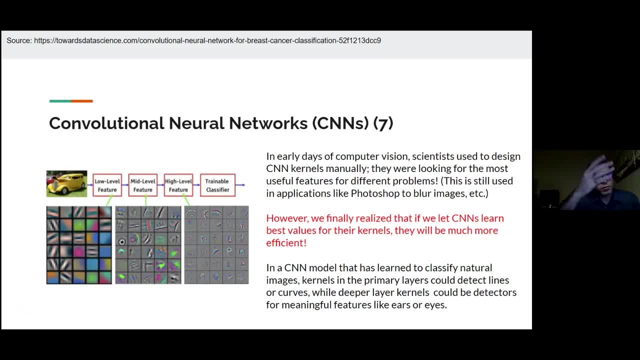 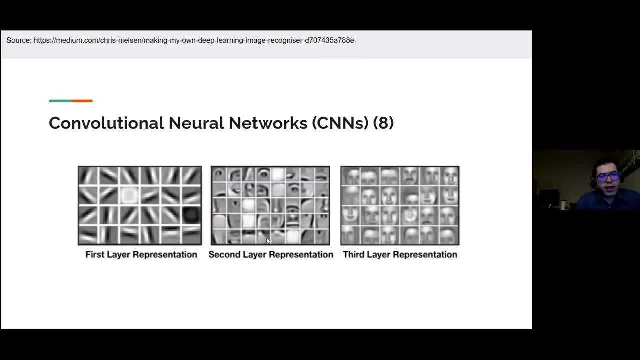 While MLP networks couldn't say so. So this is a nice fancy shape of a convolutional neural network And again another shape of that you see here. this is a model trained for detecting. Oh, thank you, Dr Versandoff. 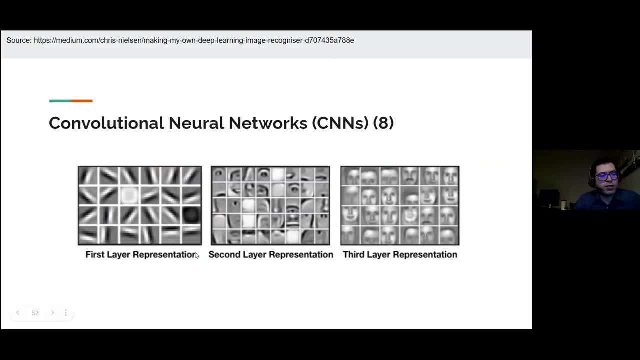 I think I will finish on time, maybe one or two minutes at most, But I will finish on time. So here you see that, another neural network. we have First layer representation. So this network wanted to distinguish human faces. First layer representation: only simple lines. 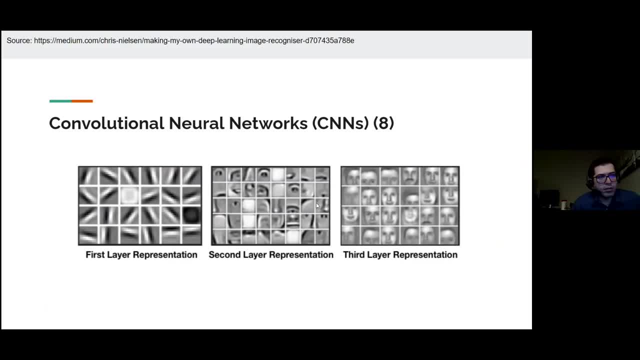 Second layer: things like eyes, nose, mouth. So this is the first layer representation. Third layer: real faces. So you see, now our neural networks, our convolutional neural networks, can really learn to pick those features that we care about. 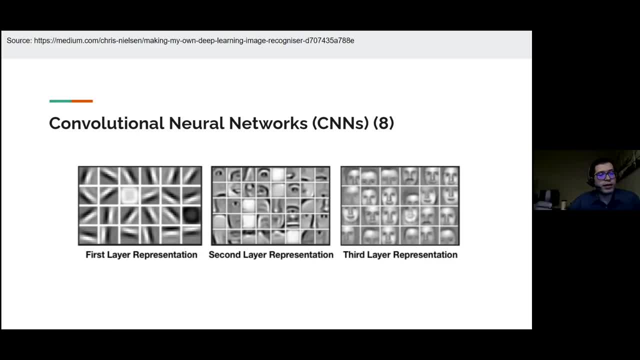 And if we train them in a decent way, then they are going to learn meaningful features And, to be honest, one of the ways that we have to understand if a model is working nicely or not is that we visualize these features and look at them. 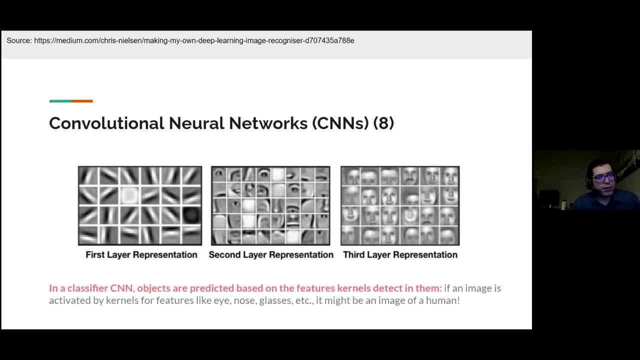 Do they really make any sense to us or not? And, of course, one thing that I can tell you, and very quickly, is that do you remember I told you this is a still image? This is still valuable to transfer. learn from, you know, models trained on natural images for medical purposes. 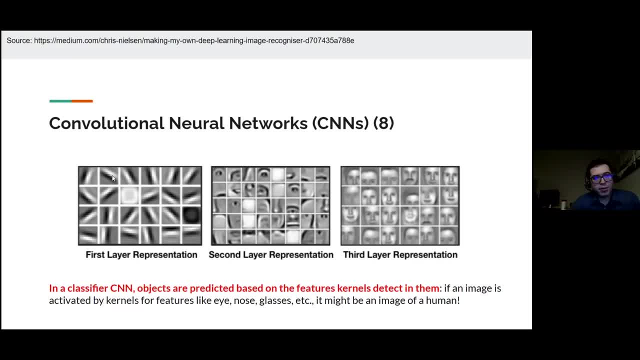 The reason is that natural images on medical purposes. they definitely do not share any high-level feature, but they do share low-level features. A cat and my CT scan image are both made of angles and lines, So if a model trained on cat images has a good line detector, let's put the weights from that and put it in my model. 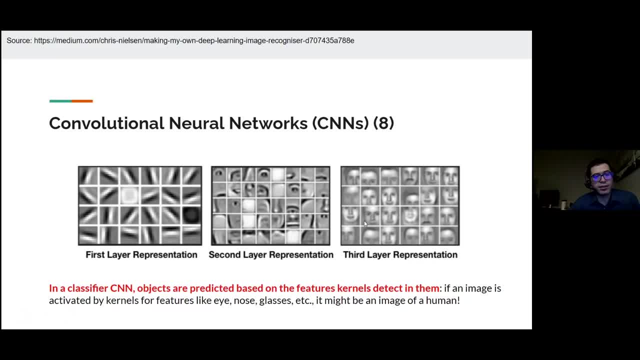 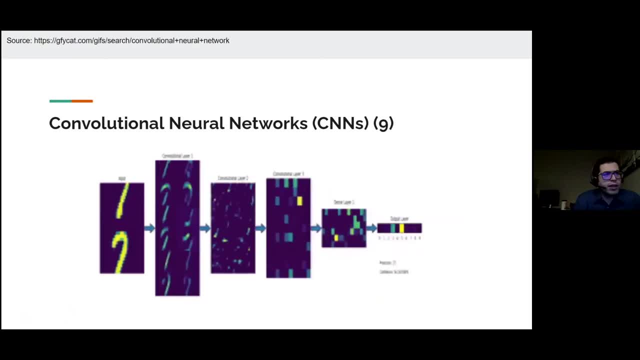 Of course, for the higher layers, for the higher convolutional layers, For the higher convolutional kernels, we need to learn by ourselves. But for lower layers, transfer learning can make a lot of sense, And I believe this is the final concept of a convolutional neural network. before I proceed to the references for further learning, 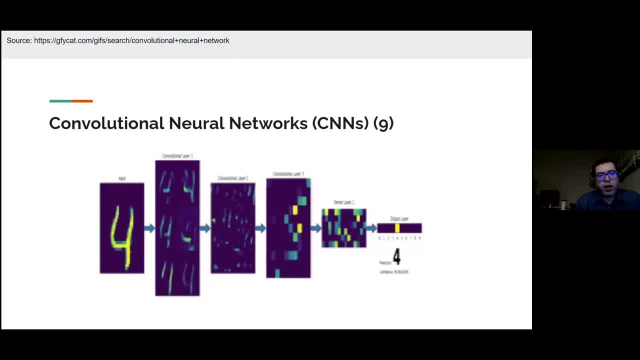 And you can now see how a training, how a prediction happens in a real case. You see the input is actually some real numbers And you see in a three-layer neural network how the features are formed. So you see that, what features the layer one is making, how features layer two are making. 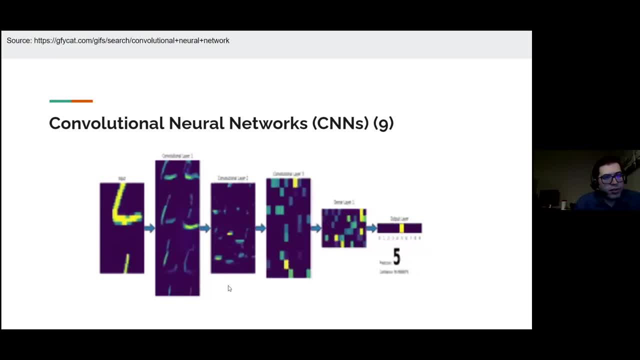 And you see here that after that we are now trying to make a final prediction value for this right. So these are the parts that, for example, this dense layer is our MLP model. So you see that now everything gets coded, gets embedded. 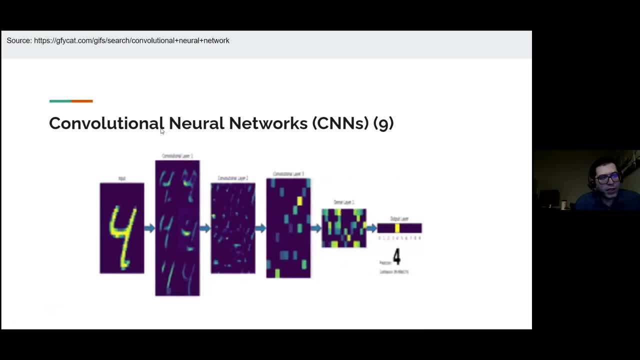 So these features, now that we finally found the main features right here- So this could be a lot of convolutions here- Now that we have the final feature, that has meaning now we try to embed them, We try to concise them, Focus them to finally get a single value like this: you know, 10 vector here, 10 value vector here, saying that this is a zero or this is a six or seven or eight, something like that. 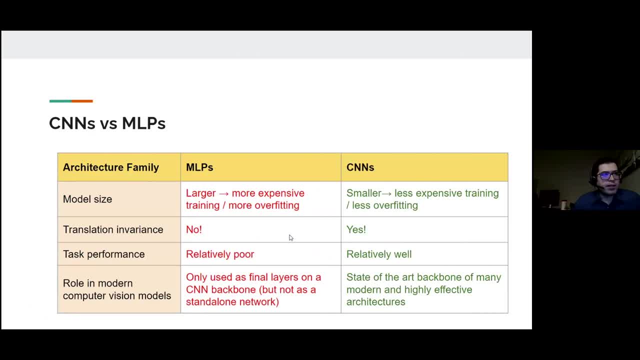 Now, in comparison, MLPs are larger, are more difficult and more expensive to train, They are not translation invariant, They do relatively poor in different jobs And they are only used in combination with CNNs in more recent architecture. So this is something important to keep in mind. 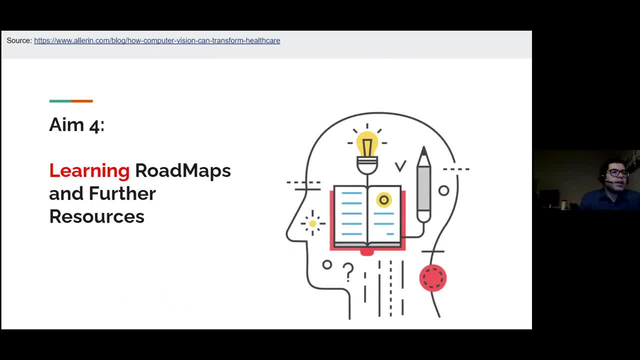 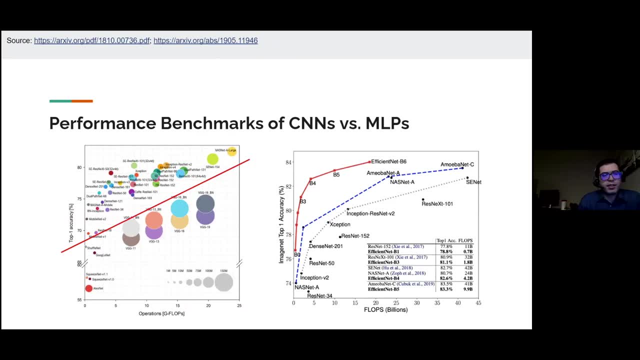 I'm going to skip these things for now. These are only comparisons of CNNs and MLP models. The only point of this chart is that you know, recent architectures are never using MLPs as their standalone- based on architectures they are, And these are the new, different type of CNNs you see in the world published. 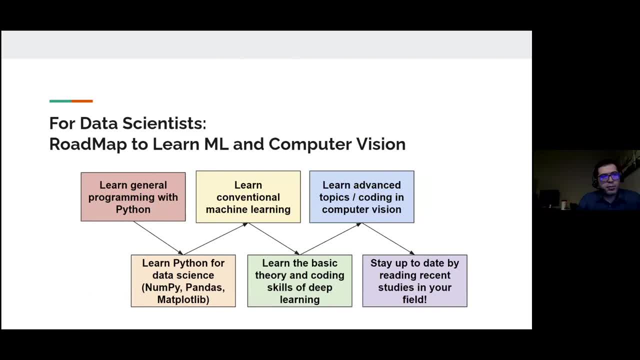 Very quickly. if you are a data scientist, you want to learn machine learning and computer vision, you should first learn Python, Then go through Python for data science. We do have specific libraries in Python designed for data science. Then you should learn Python for data science. 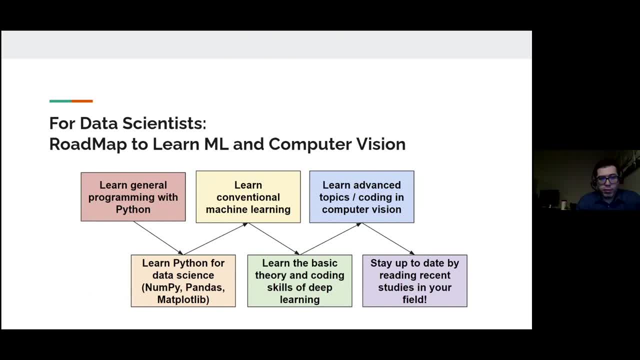 Then you should learn conventional machine learning Probably. This is actually what I prefer to say. Some people say that you could directly go to deep learning, But you know many of the resources out there. they say that it's good to learn at least a little bit of conventional machine learning. 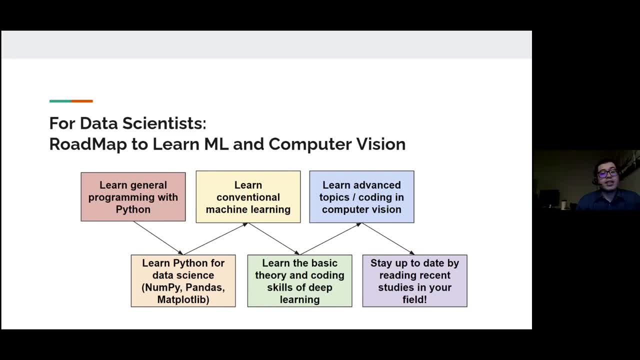 Then learn the basic and theory of you know deep learning and how to apply that in Python, And then focus on your area of interest, for example computer vision, And then, finally, the most important thing is stay up to date. 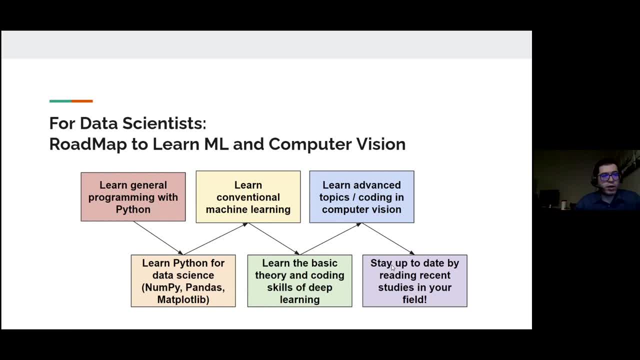 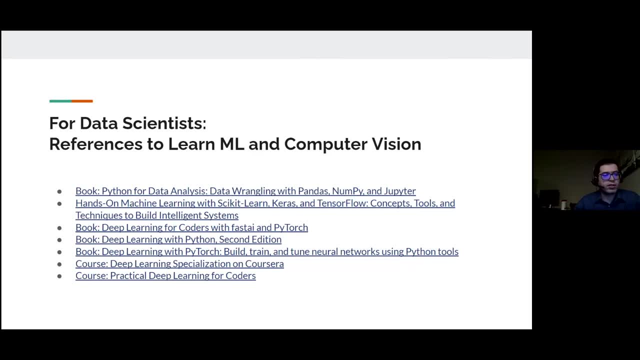 Deep learning is a very dynamic field. It's a very growing field. New papers come out every day And you should really be up to date. These are book chapters, courses And, if you are interested to go through them, these are the good things that Dr Erickson and many colleagues in our lab have already tested those. 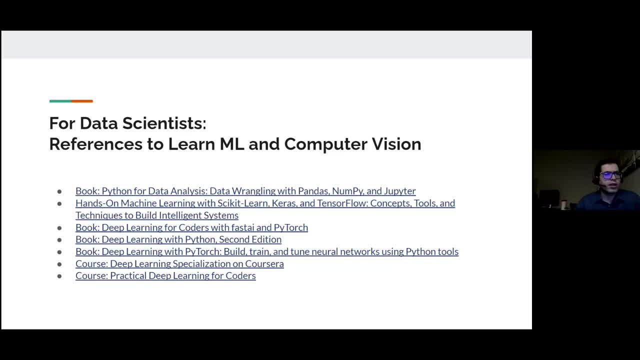 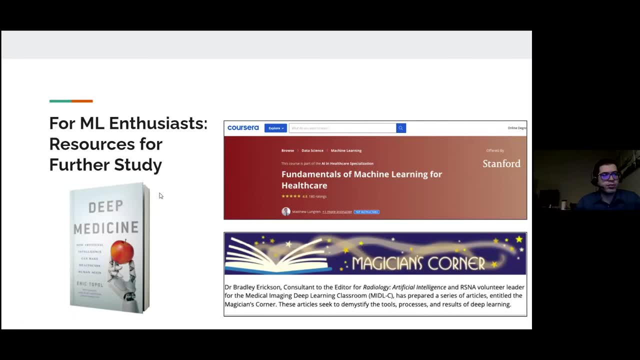 So feel free to test those. I guess all of them are freely available to you if you want to find them. And if you are not a programmer but are still interested in learning machine learning, a couple of things for you. This book by Eric Topol is a good start point.